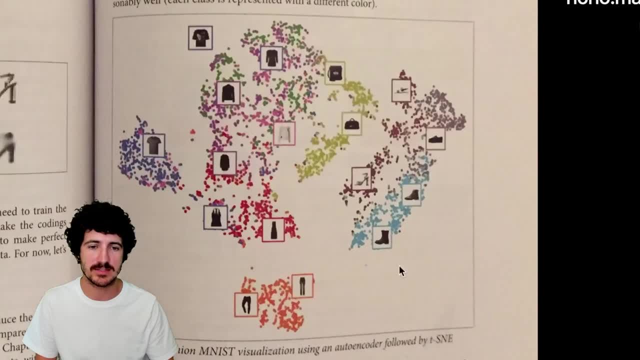 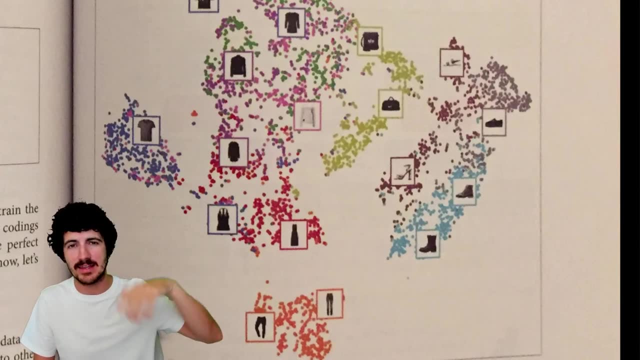 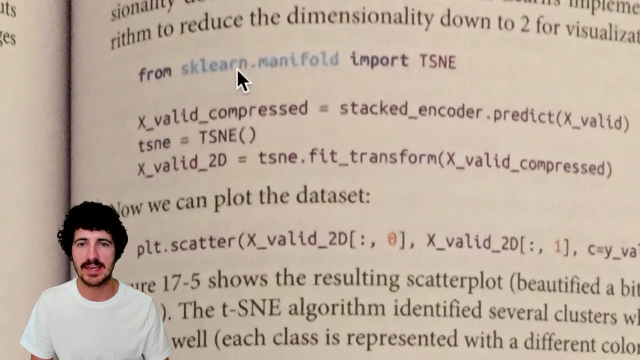 good architectures for generating images, So this is what we would imagine that we can obtain. This is a t-SNE flattening a highly dimensional space with these libraries. So the t-SNE library from Scikit-Learn Manifold, And this is really pixelated because this is a really bad image, but I'm going to show you how it works. 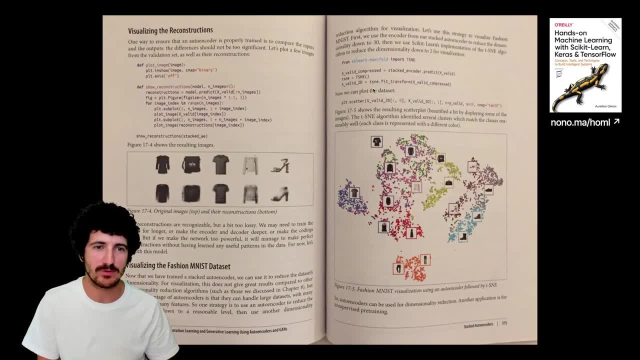 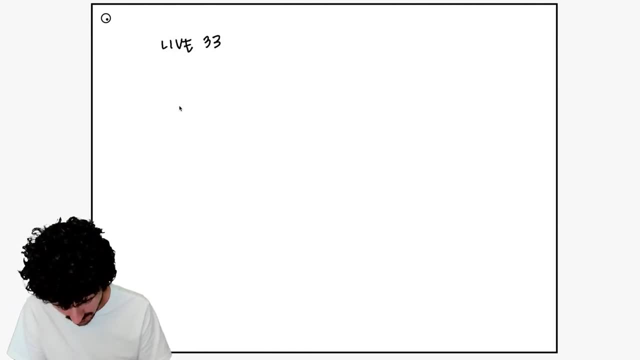 But I have the book here with me. So, yeah, we're going to try to visualize that. Okay, So in Livestream. so live 33 and 34, we did see stacked autoencoders We made, I believe. 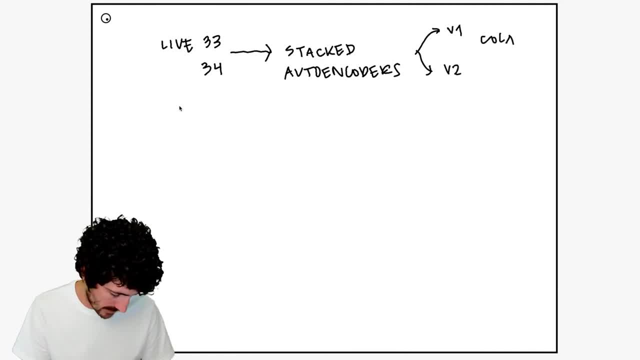 two versions of a collab notebook In there. we were actually having that architecture in which we were taking in an image, So that would be like maybe a PNG. I think that was 28 by 28.. We were encoding that into a 30 digits right. So these were the codings of our network. 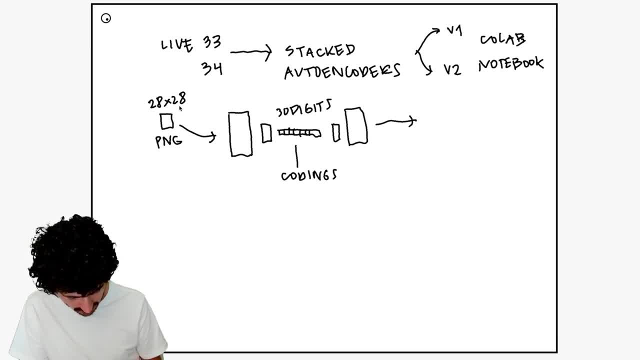 And then we were getting that back into another image that is 25 by 25.. That was the reconstruction And this was our input. So we try to do here is to train this part, which is an encoder, and this part here, that is the decoder. 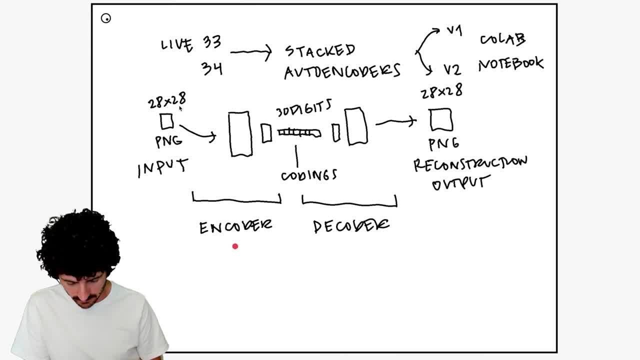 What the encoder learns how to do. So the encoder learns how to take an image. So, whatever it is, And it's 28 by 28.. which is 768 pixels into a one D tensor or Ray that has just, is one by 30.. 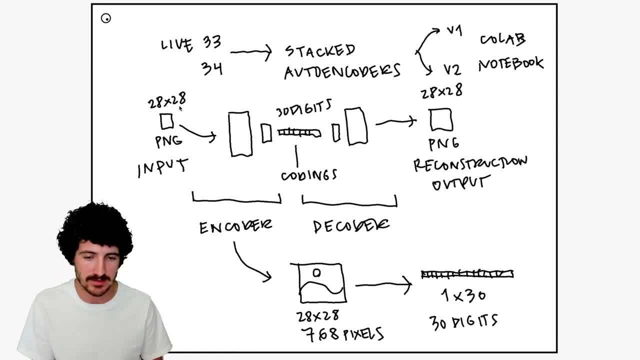 So it has 30 digits, right, It's just 30 digits is not pixels, because here actually we have RGB, So three channels for each of those pixels, All right. So we're trying to get- and I'm going to go to the next page now- trying to get a 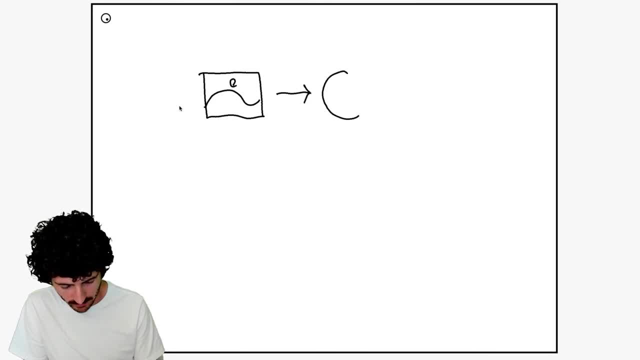 network where we put an image right. So we have our network here, which is a decoder, and we're going to get. so this is our input and this is our coatings, and those coatings that I mentioned are going to be one 30.. 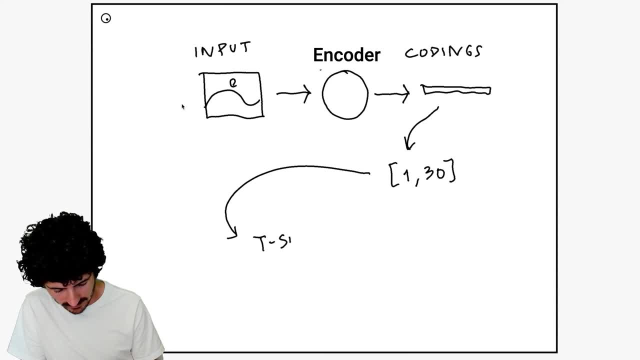 So 30 digits will then input into Disney and are going to be able to plot on a two D image And hopefully We're going to get it Clusters that belong to different classes, So, for example, this could be a type one or type two. 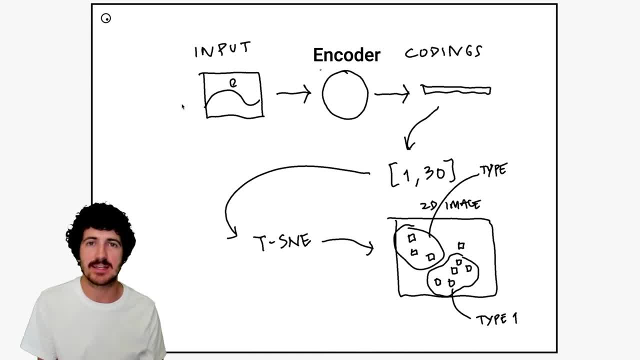 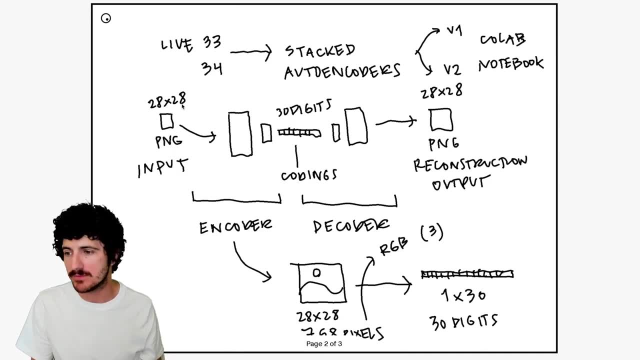 The problem is that the data set that we're going to use- those sketches that I showed before, those- don't really have a like. we don't have a classifier to classify them, So we'll just see how the data samples look in similarity between them. 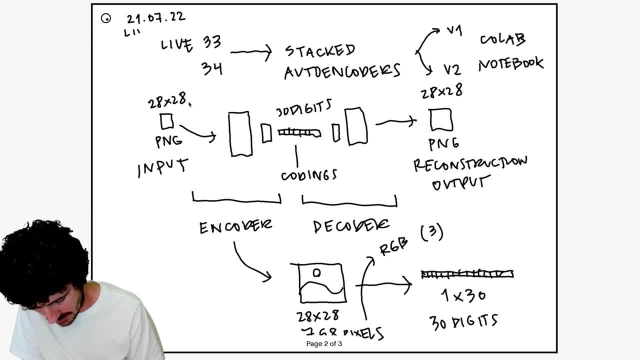 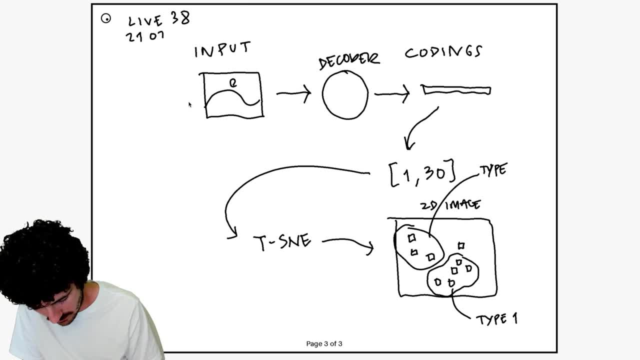 So we're just going to try to do that. Let's just add here live 38. So this is like 38 and it's 22nd of your life, All right, So I'm going to read here the comment from Ricardo. 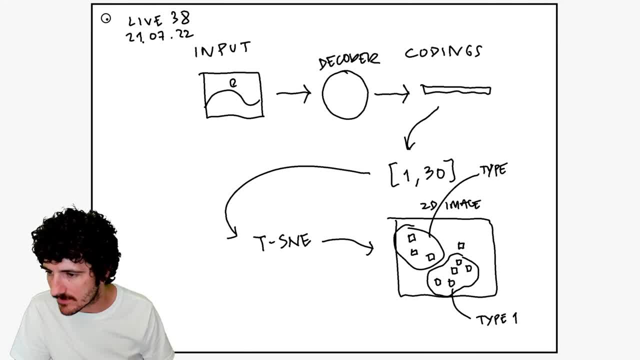 So I've already used this knee. Let me see Oh message retracted. I was going to read it in Ricardo, but you lead it before I could do that. So if you want to rewrite, if not, it's fine. 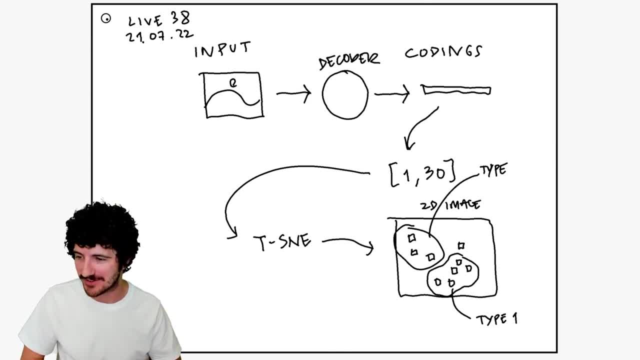 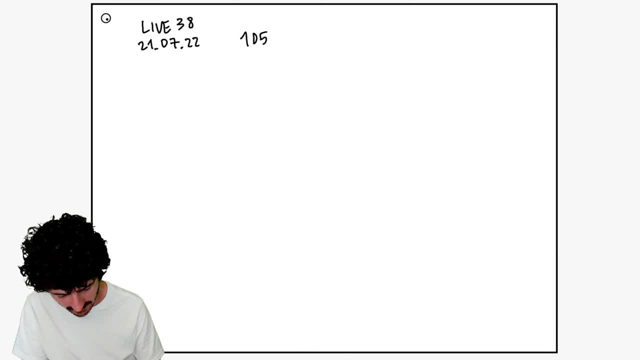 Up to you I was. now I'm curious about where, Yeah, You were going to say that you've already used at Disney. Okay, So let's keep going. We have a set of 105 images, We need to recover our notebook and, uh, we need to make a. 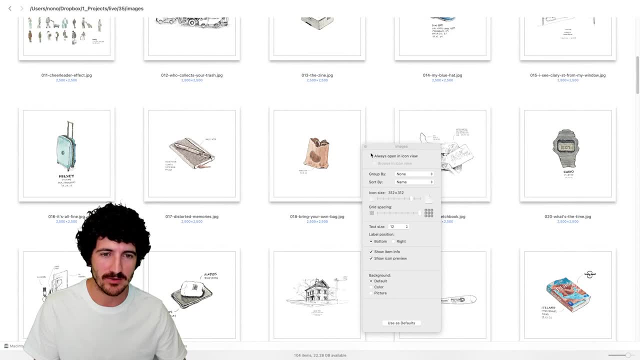 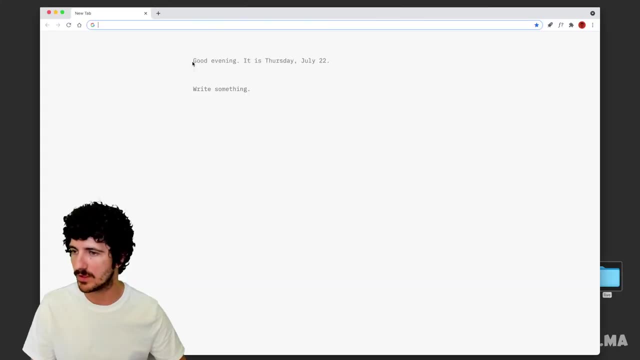 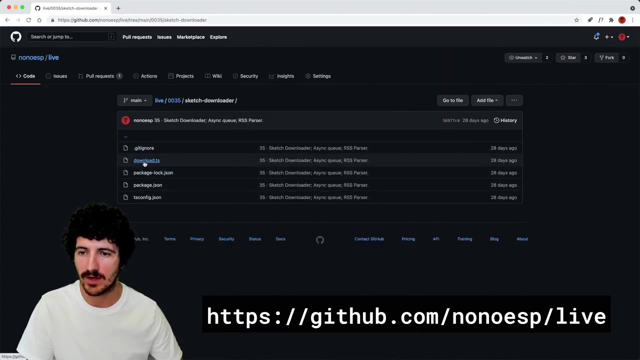 notebook with site kit- learn All right. So this is a data set and these has 105 sketches from the website. If you go Into the live repository, So this is the repository of the live streams in live stream 35.. You have a TypeScript script that will guide you step-by-step on how to use an. 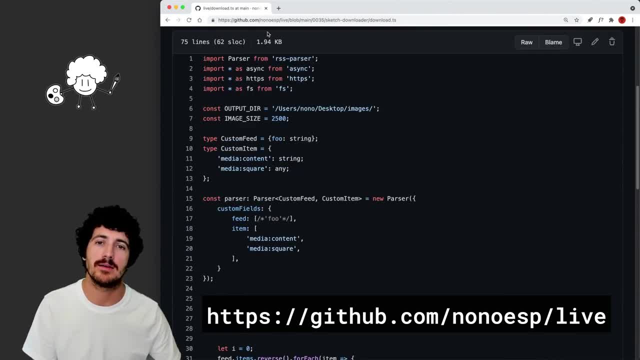 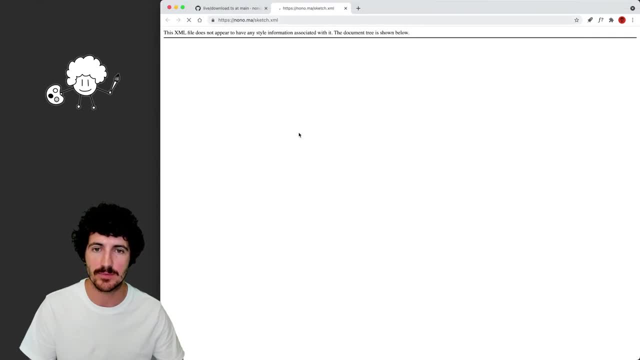 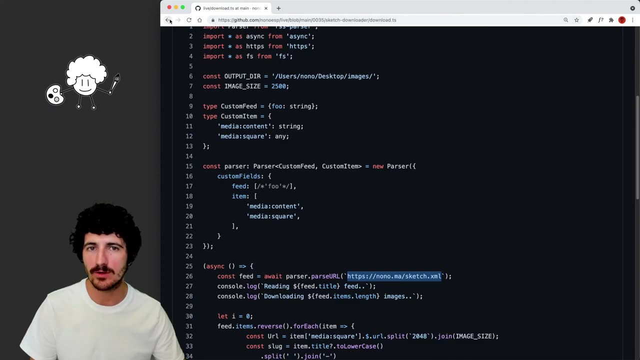 asynchronous pipeline to download those images from my RSS feed. that is here, but you can actually change the URL of the RSS feed and a few properties to download images from another source. In this case, we were just getting the images from here, So you can go there to take a look at that. 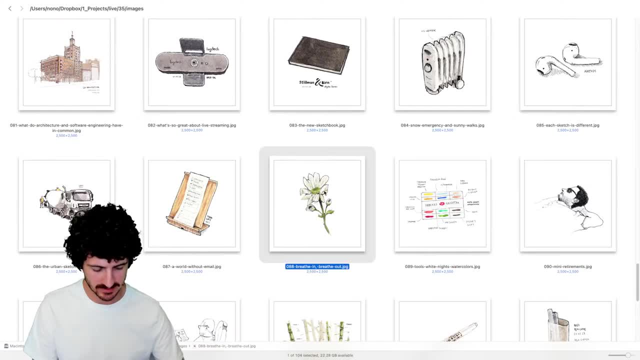 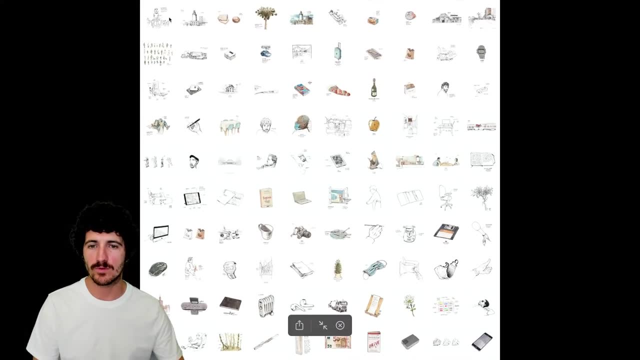 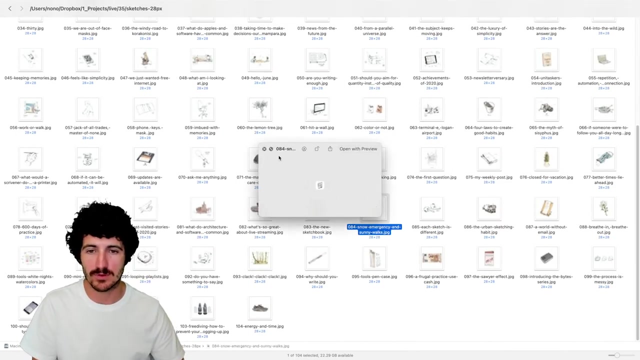 I was mentioning, we have these 105 images. These ones are 2,500 pixels height, So the purpose of having the the images down to 28 pixels is to be able to put them into the Keras model and have the training be a bit faster. 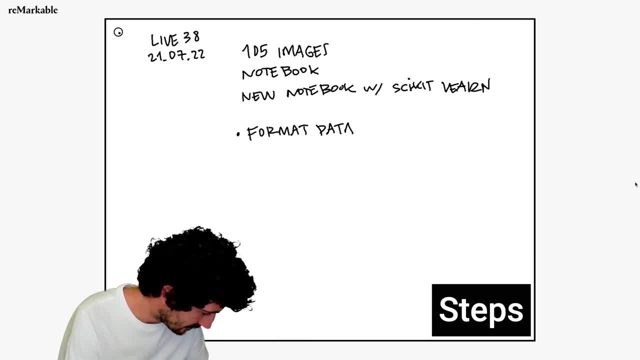 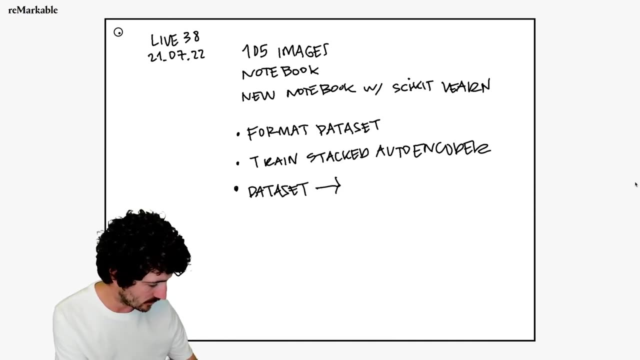 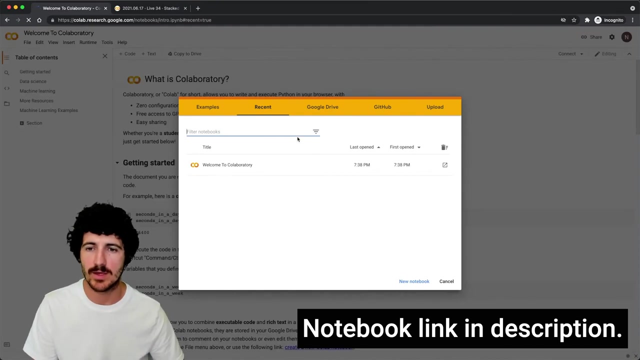 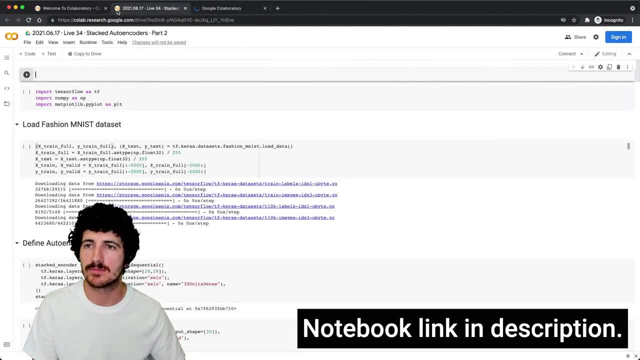 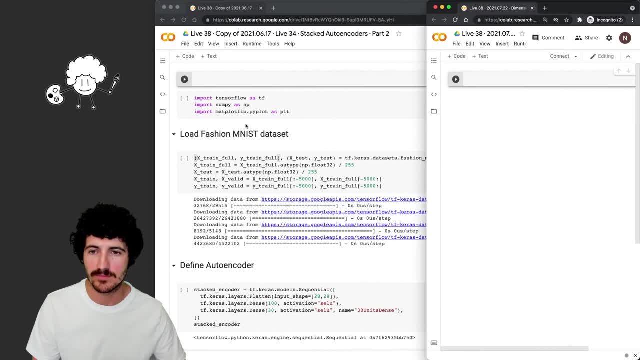 Right, Right, Right. Google call up here and we can now access the stacked out to encoders notebook. Let's see what parts of the code we need from the previous notebook. The first thing that we have is that we have the fashion MNs data set and 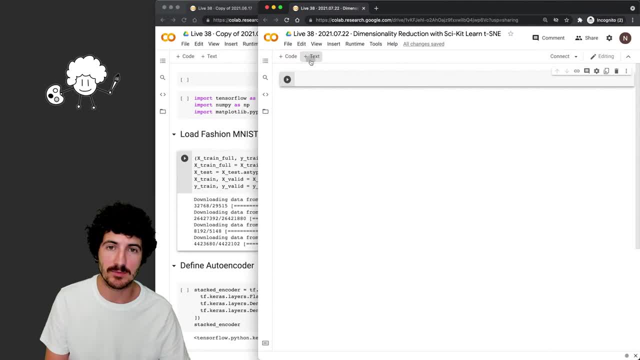 I want to do this with our own data. So what I'm going to do first is I'm going to add a text block here. I'm going to say load to data set and this is like: images are 28 by 28 pixels. 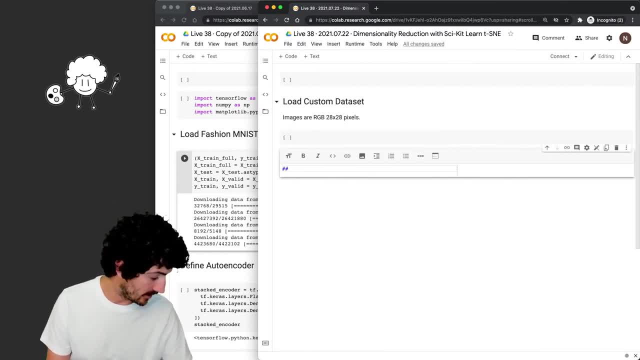 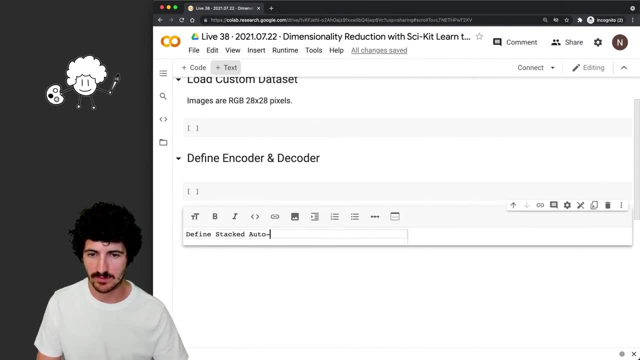 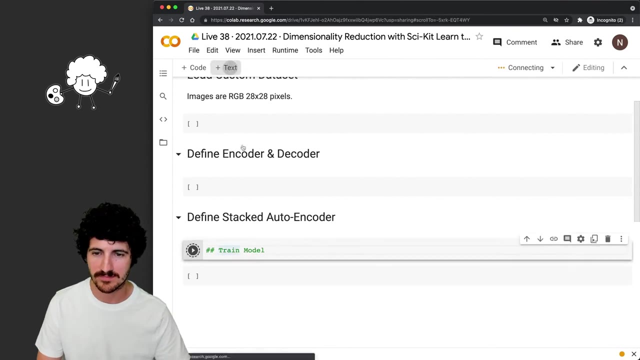 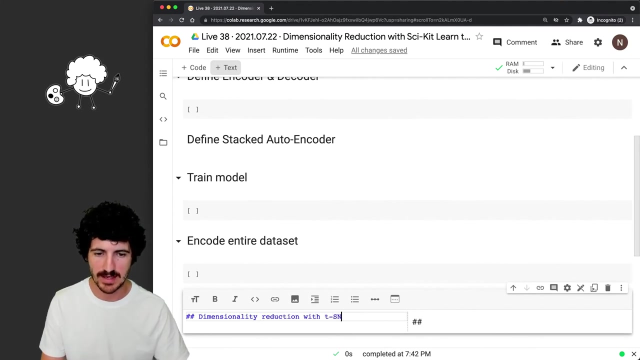 RGB. Then the second thing that I said is that we need to define encoder and decoder, define a stack out to coder, then train model And then we'll have to well, the reduction with Disney. All right, let's take a look at what we have. 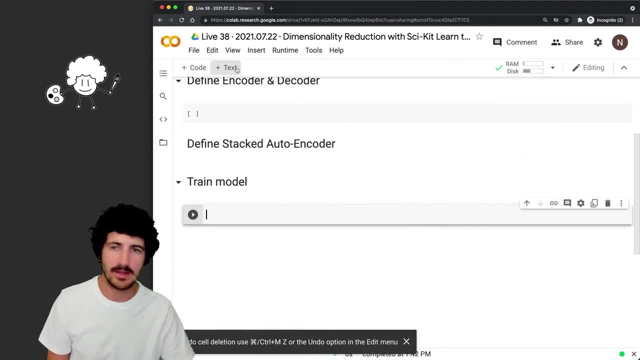 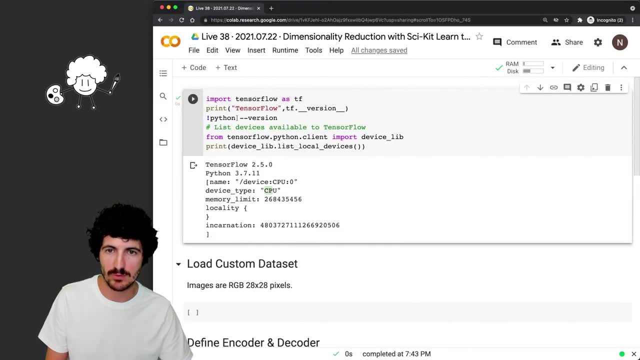 So we have tensorflow 2.5.0.. And Uh, later would have to encode entire data set. We have Python 3.7.. We have a CPU and we don't have any views. We can select the GPU here to make our notebook faster. 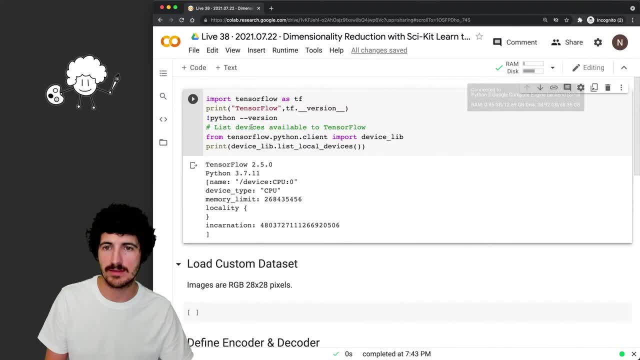 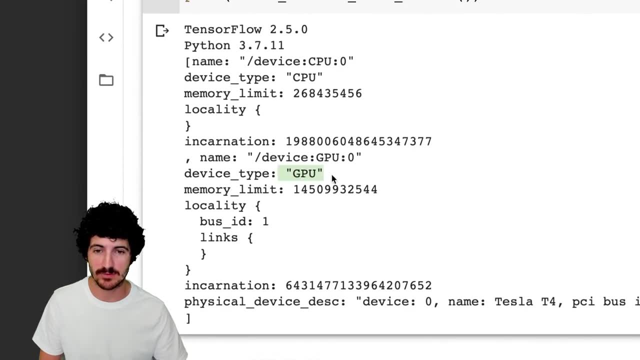 So this is now going to allocate it for you and initialize a new runtime. So now we run this again, We're going to have the same version of tension from Python. So now we have a GPU device: is a Tesla T four? Where do we have our data set? 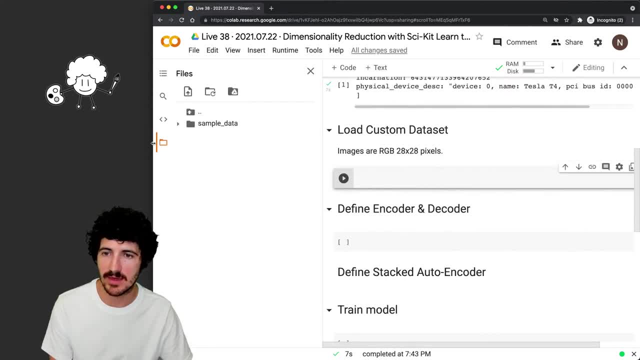 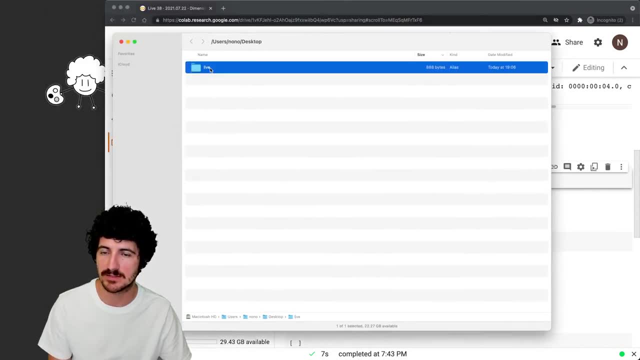 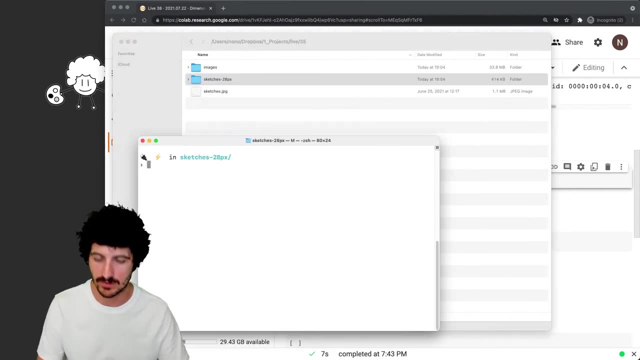 How are we going to put our Data set here, and maybe the easiest is that we just drag and drop, because this is a really small data set. The problem is that these, might you know, require that we do that every single time that we want to do this. but I'm going to go into this sketches folder. 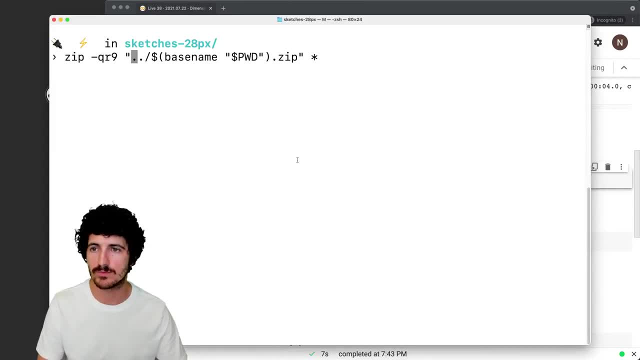 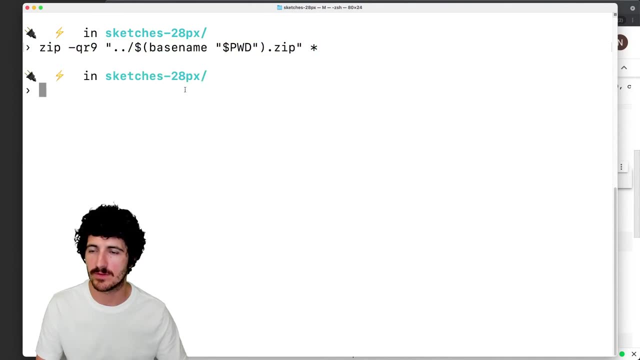 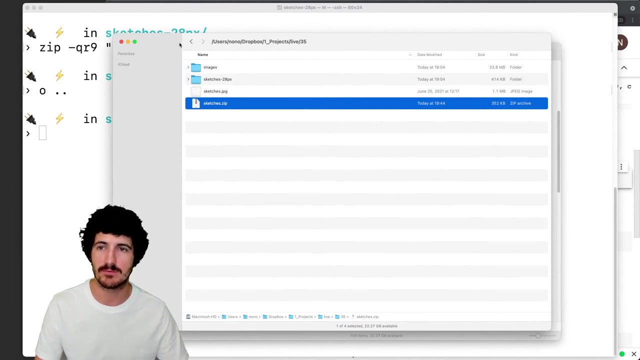 I'm going to use this script to see my file. So it's just: I go into the folder and I just call this, which is just zipping the file with the same name that the folder has. So maybe we just call it sketches, and this is 352 KBs. 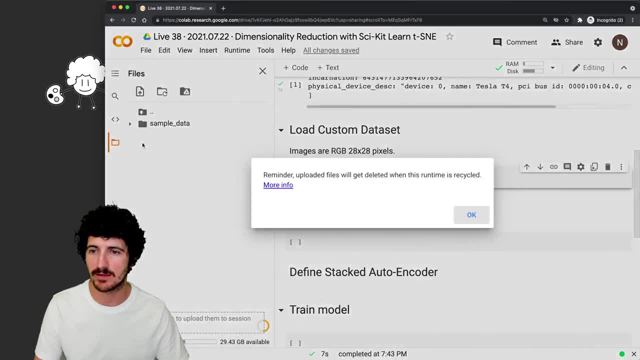 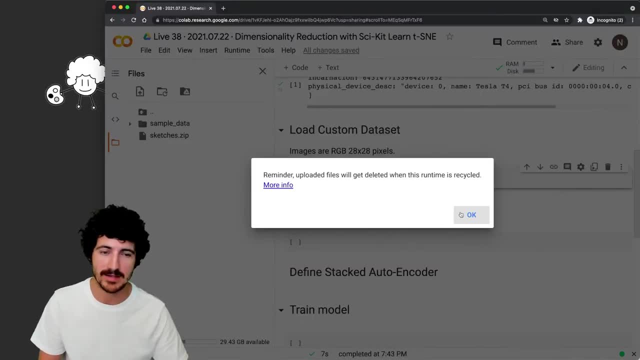 This is super small. We're going to simply drag and drop that into our notebook. A reminder that files will get deleted when the runtime is recycled. So if you close your notebook, go away and then come back, The data there is not going to be there. 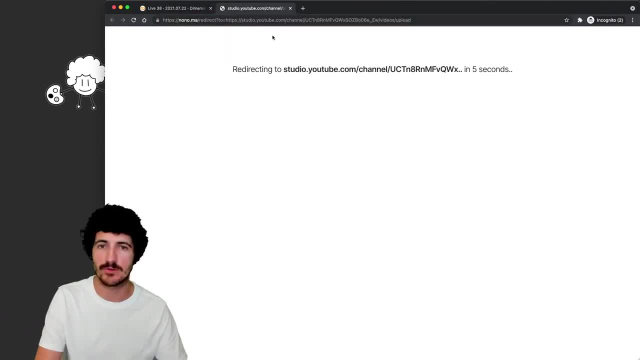 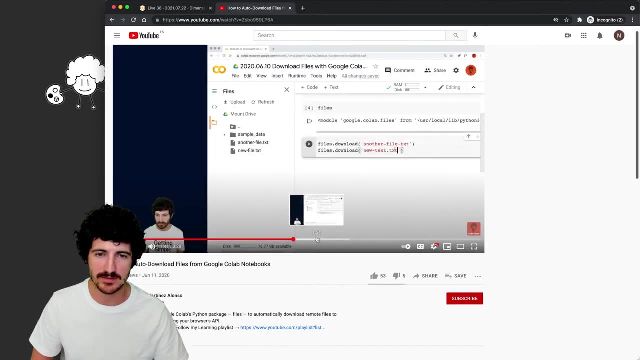 So there are ways in which you can download those files from other source or upload them somewhere. I have a video here on how to auto download files from Google cold up, And this is something that I really liked, because that way, Yeah, You can run your notebook and then your files end up on your downloads folder. 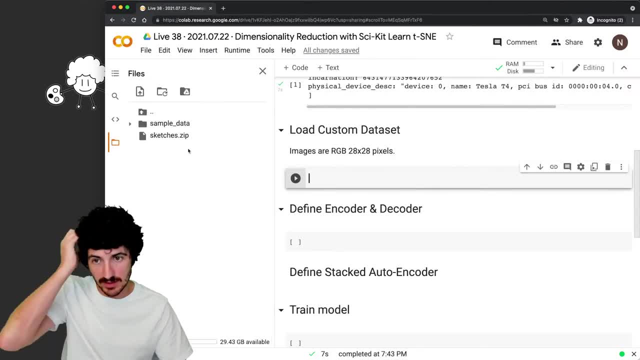 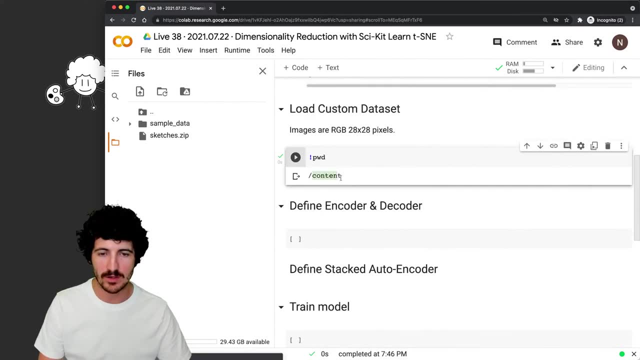 and you don't have to worry about that limitation. Now we have this here and I guess we could unzip them. load custom data sets. We're going to do some preparation here. We're in the content folder, which is this one here, So we can do unzip sketcheszip. 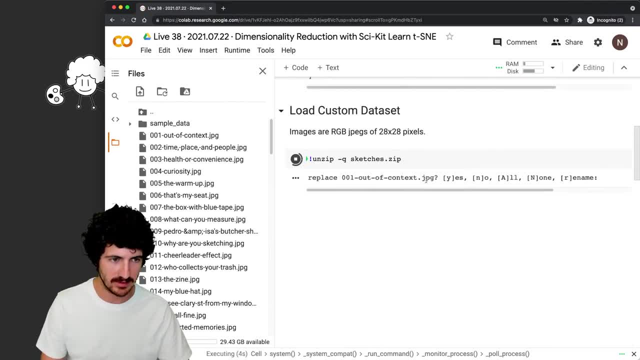 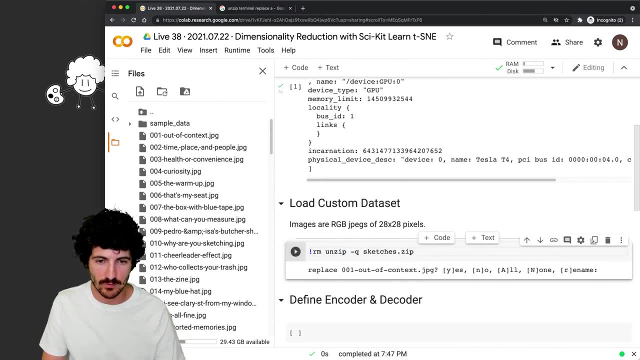 If we put here the, this process is silent, so we don't see anything except for that. One thing that we can do to avoid these sort of questions is we can just say: remove all the JPEGs in this folder and then unzip that way. 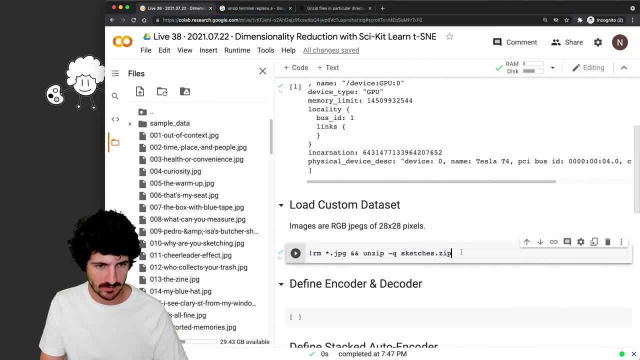 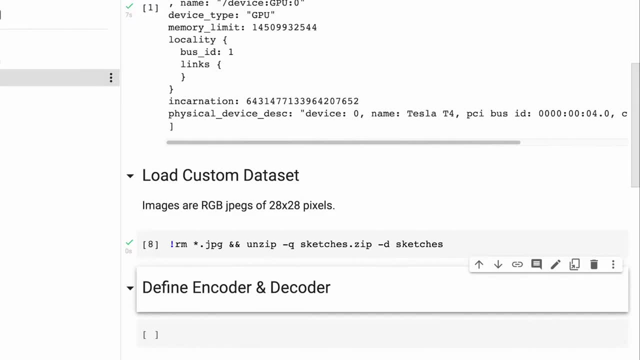 Everything gets removed and then zipped again. We can specify here to unzip on sketches. that way We unzip to a directory instead of to the main folder. All right, So now we have our 28 by 28 pixel sketches here, which is our dataset, which is super small. 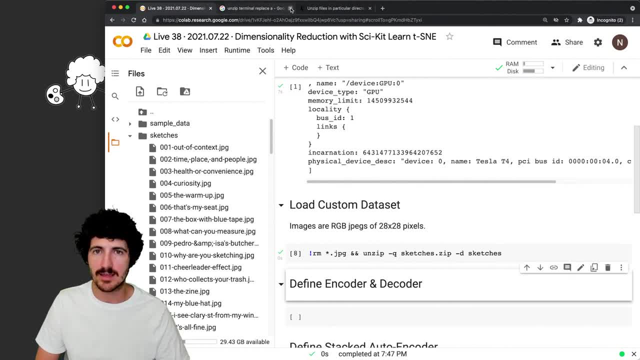 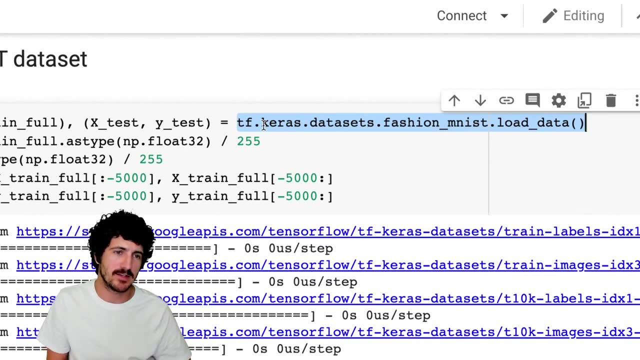 Now we need to see how to load that in the same data format that we had our dataset on the previous live stream. So this notebook here you can see we're downloading with this function here. So tfdatasets, fashion, MNIST, load data. 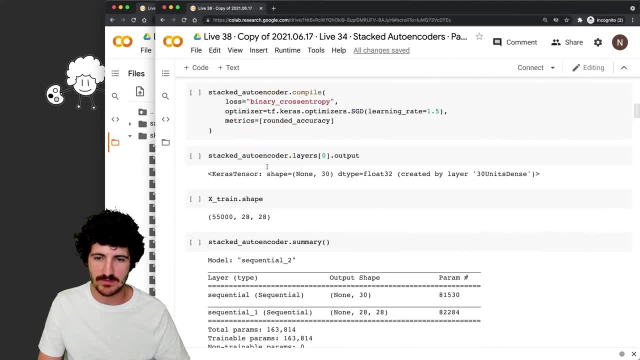 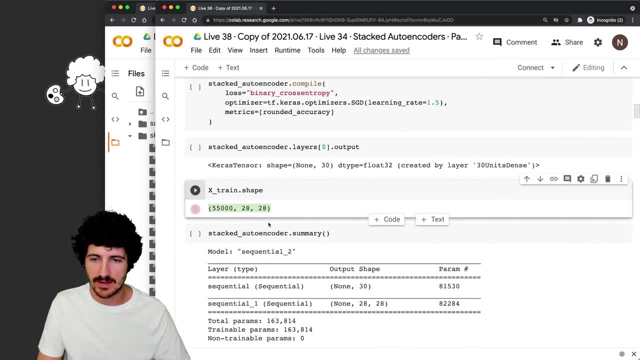 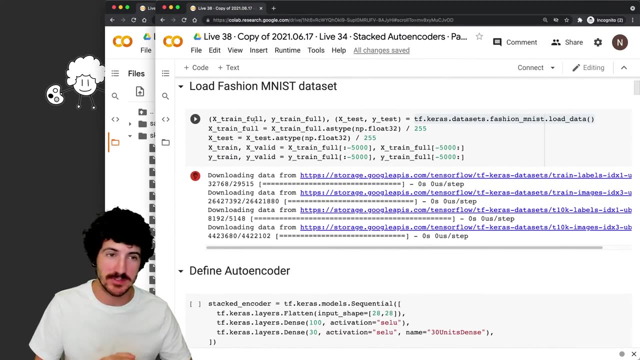 This gives us data in a really specific format at 28 by 28 pixels, and they're 55,000.. So we want to get our data in the same format, but in um, having less, less of them. We only have 105 samples, which is going to. 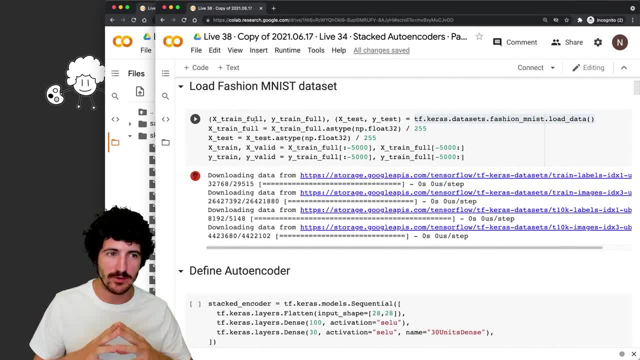 To overfeed a lot And this is not something that I had thought of, but at least we can set up this notebook So we load all of our data. We have extreme full white rainfall And there's the test. Let's try to load our data with TensorFlow. 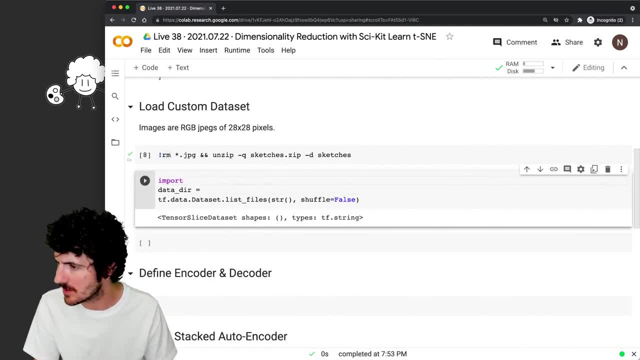 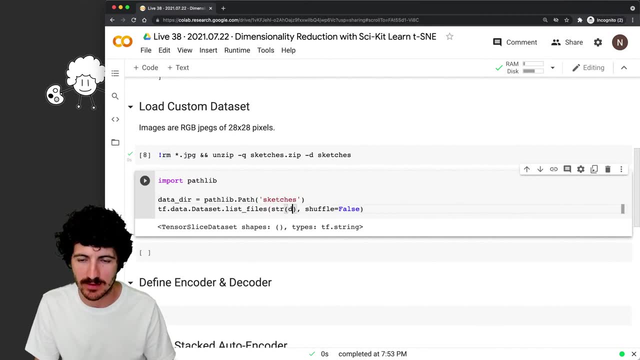 Let's take a look here, So just to see if this works. so I'm going to import path lab and I'm going to call path lab, path sketches, And then here we're going to do data there, And then our pattern here is going to be just everything here with JPEG. 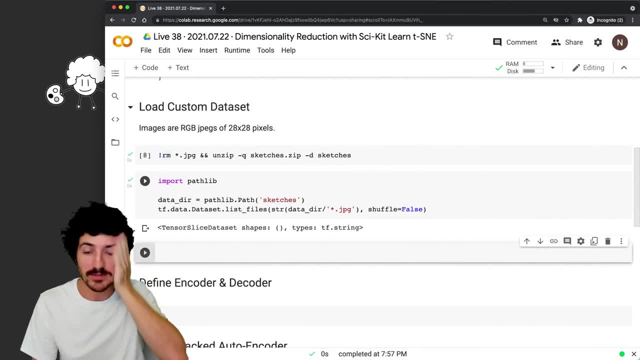 All right, Let's see if that executes. All right, We get shapes, types, strings. This was good before, just that. I don't think we even need these things If we just put here sketches, but keep it for later, just in case. 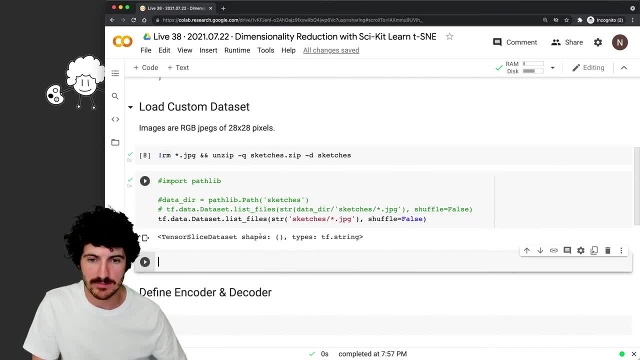 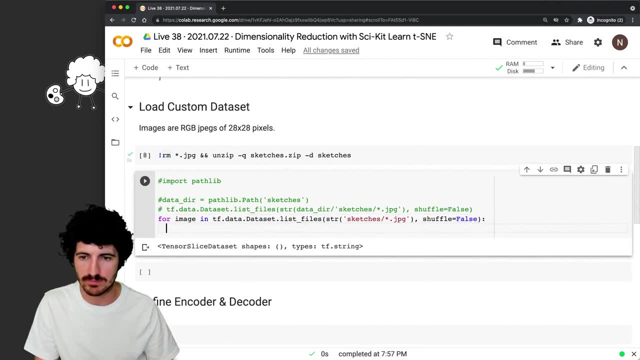 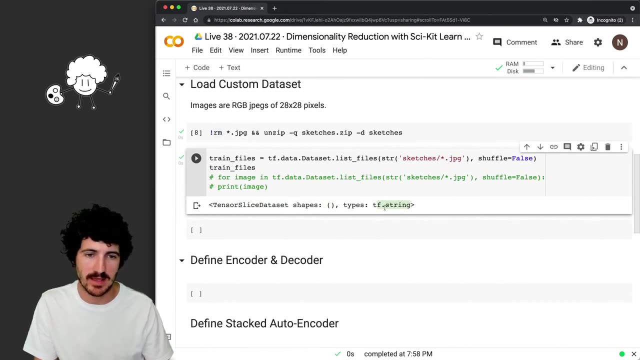 I think I was doing something Okay. The problem is that these are strings and they don't have a shape. so we could say for image in. So what we have here is a tensor slice, data set which doesn't have any shape. because if the type is string and with those train files, so we can say here train files and we can say here file, we can print the file and, yeah, again we get these binary, a string, here. 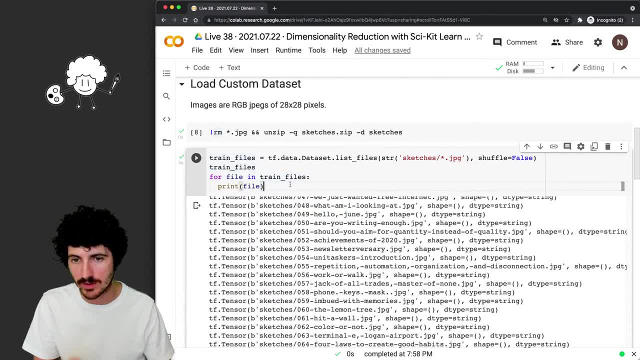 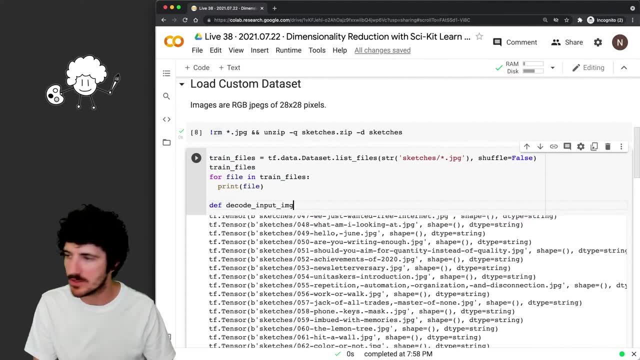 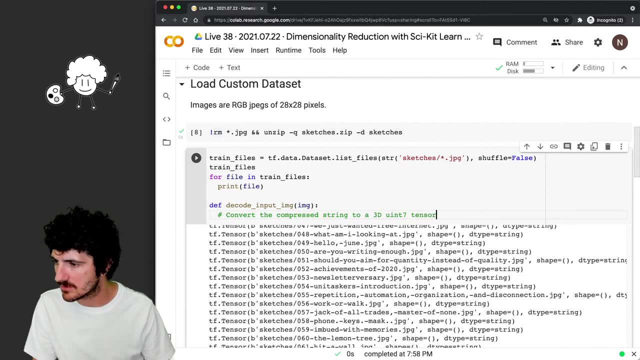 That is just the path to the string. So we need a function now to decode those images. right? So the code JPEG. we're going to define a function that is going to decode an input image And convert the compressed string to a 3d you in a denser. 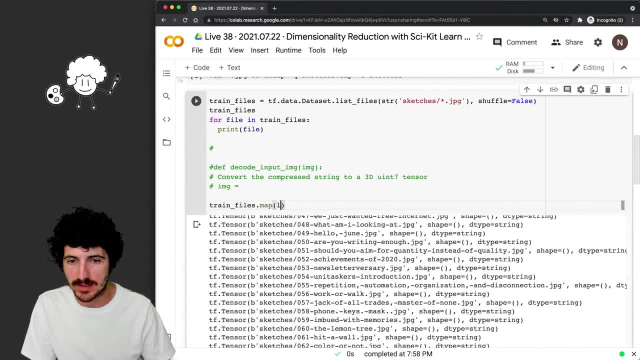 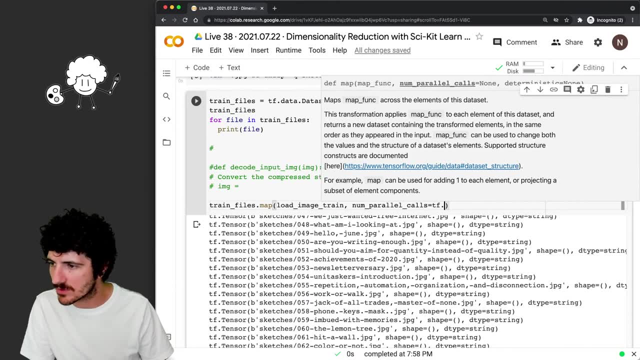 We're going to need to call on train files. We'll map and then call a function that we haven't defined yet, That is, load image train and non-parlaying calls. We're going to use autotune and, of course, this is going to fail because that function doesn't exist. 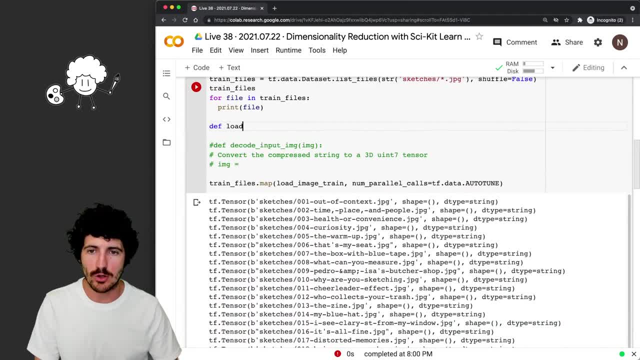 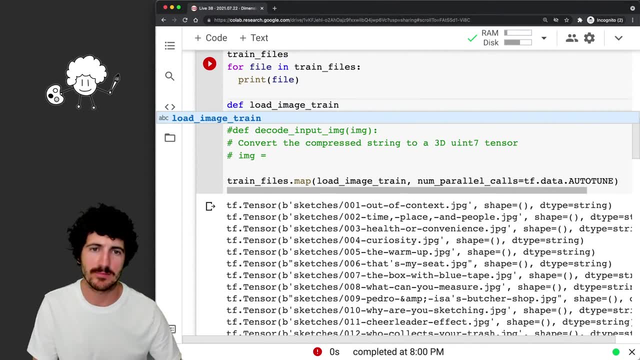 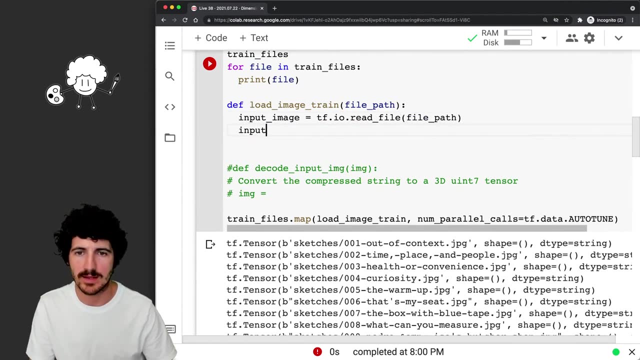 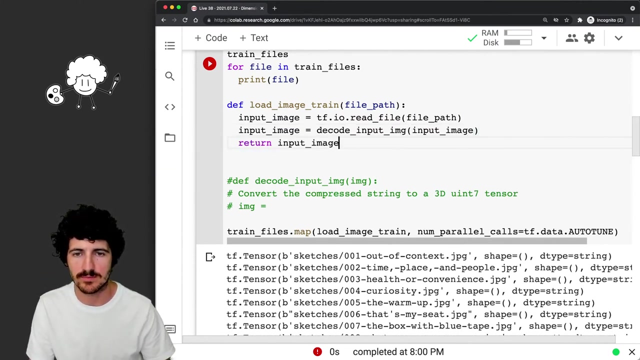 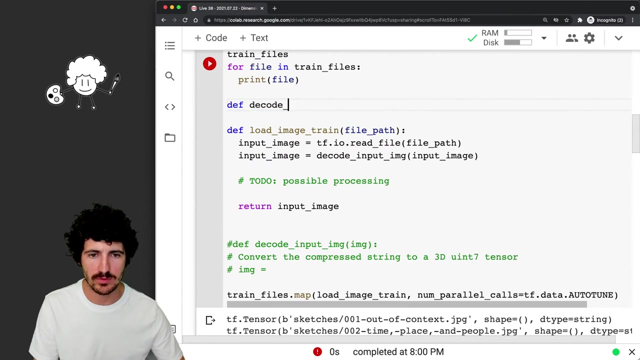 So we're loading the data set and we're going to define that load image train function. We get the file path and what we do is that input image is going to read the files of the file path and that input image of the code, our input image, and we're just going to return that input image. and we could do other processing here that I'll show here and we need now that decode input image function that I was going to define below before. 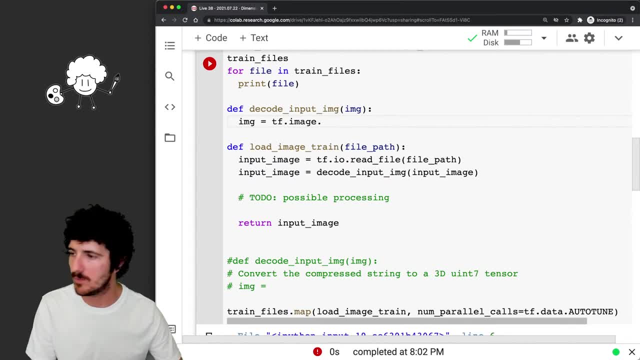 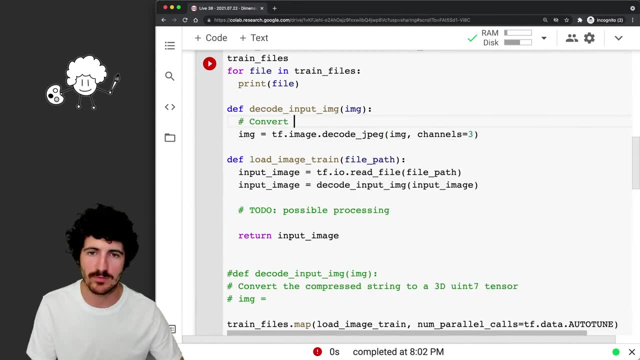 So we're going to get the input image. We're going to get the input image- TF image, decode, JPEG- with that image data that we've stained, And we have three channels. What this is doing is that we're converting the compressed string to a 3d. you in a denser. 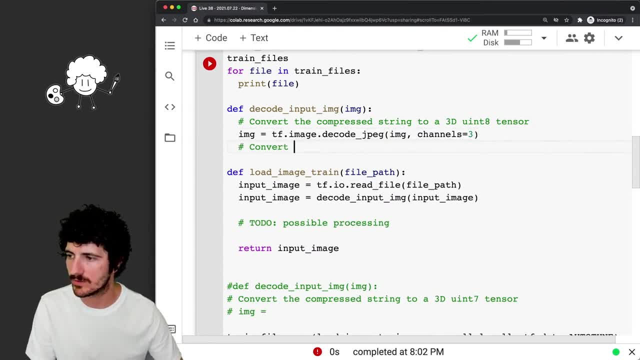 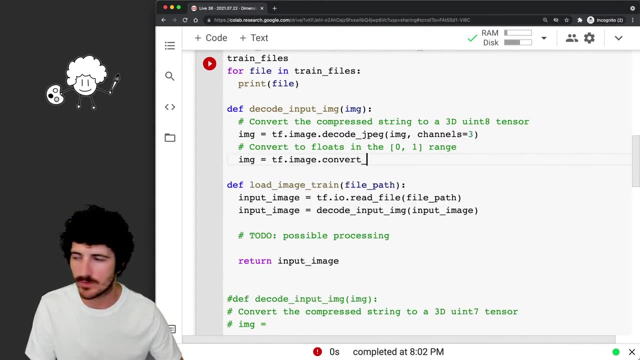 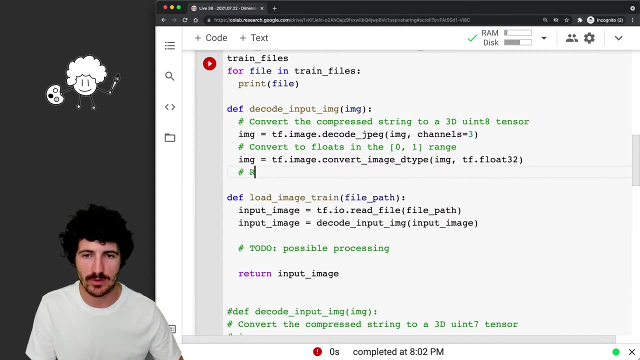 And now what we do is we convert to floats in the zero, to one range. So we use TF image, convert image D type And We Get a TF flow 32.. Now we would maybe here resize the image to the desired size, which you know it's going to be here 28 by 28.. 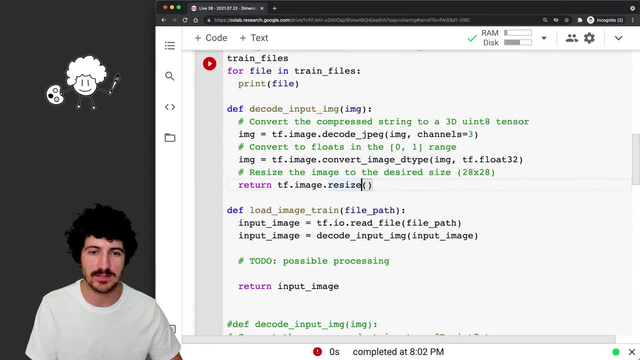 But if we do this, then the data set doesn't need to infer the image size and we can do other operations. So we can do here Image with an image height and anti-AIDS. we can choose here. They're true or false. 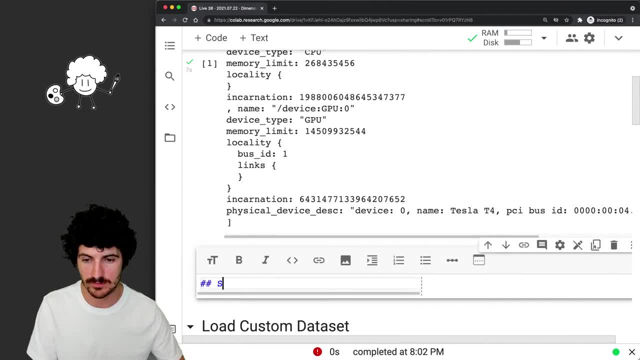 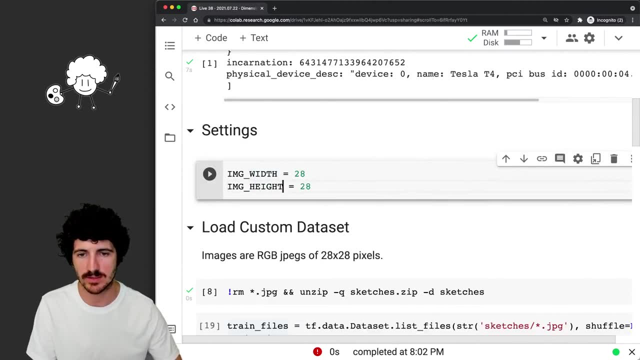 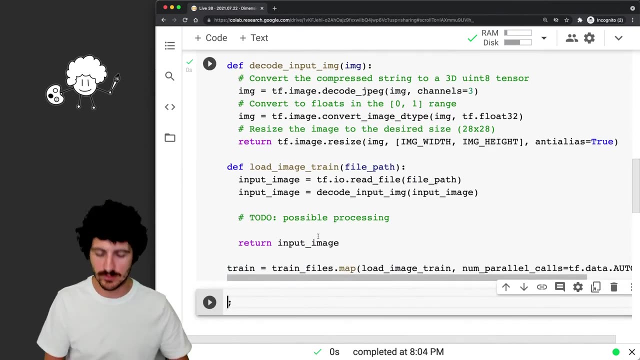 So a hyper parameter here. I will put: here are Settings and we'll put here image with equals 28. image height is going to also be 28.. We're here, So we're loading and then we resize the image. So this is going to be the train data, which we don't really have: test data. 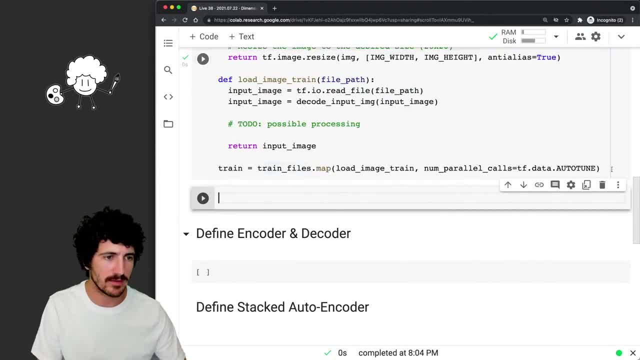 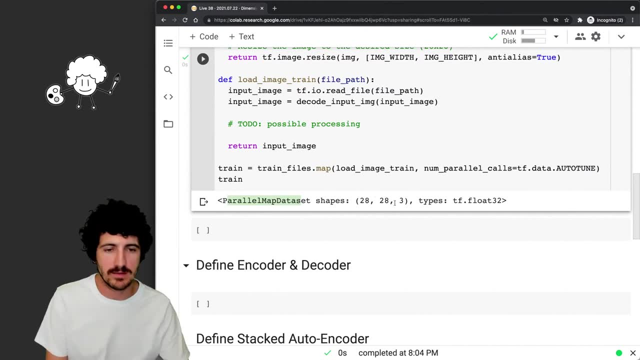 So we might need to do some split later, But for now let's see what we got here. So we got this train. We have a parallel um data set with shapes 28 by 28.. By three. There's one thing that is different here. 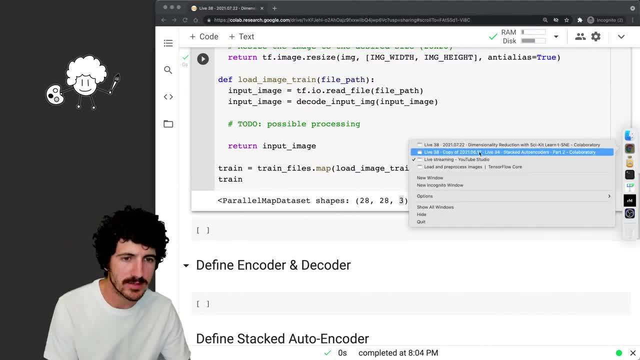 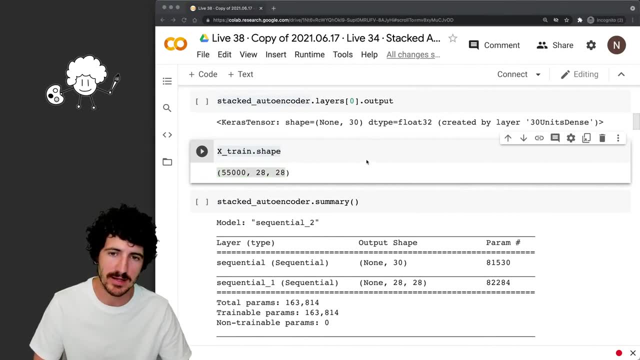 Wrong Um the previews. So we were getting the shape right, We were actually getting just black and whites. Well, I mean, we do want the images to be black, to be color, but maybe that makes this a problem. 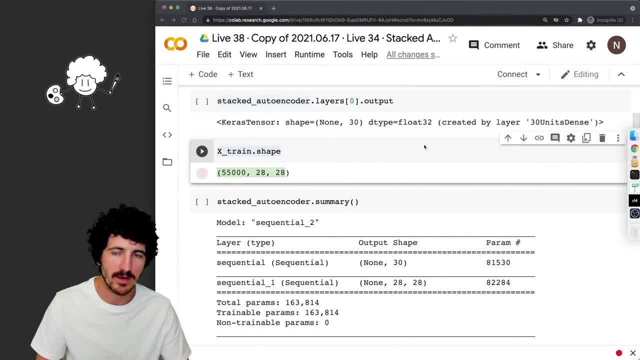 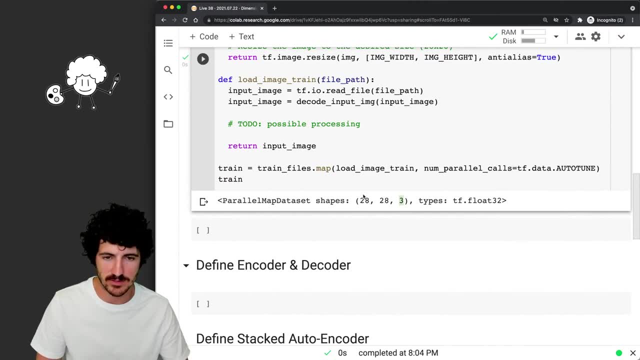 I have been more complex, a bit different than what we had before, And we'll have to change the um, the neural network architecture. So we have 28,, 28,, three- These are the shapes train, If we do a train data set and we run. 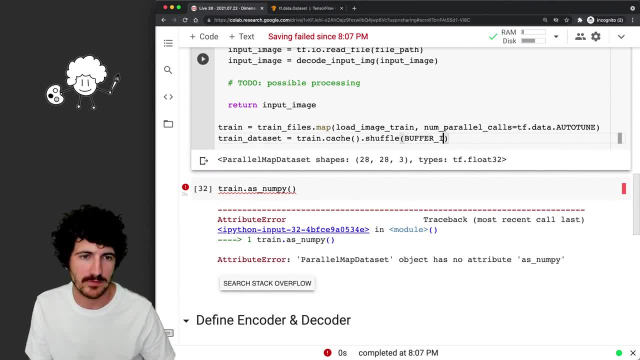 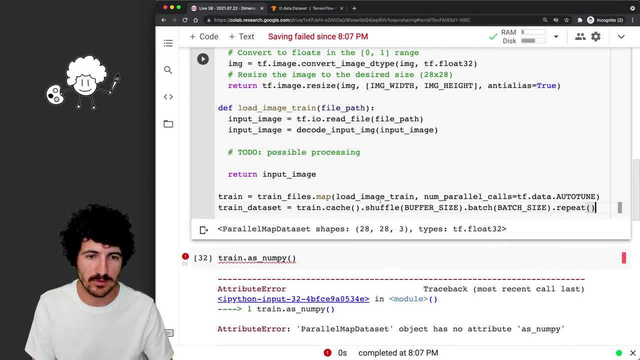 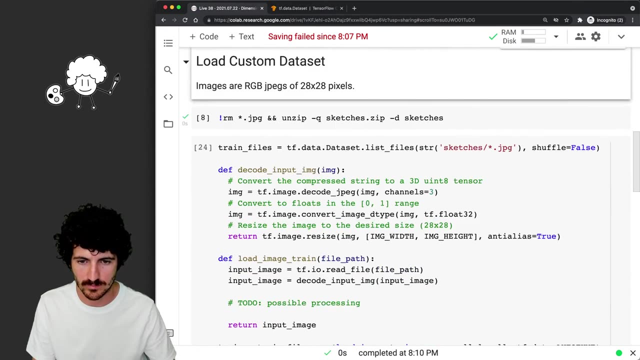 Run train cash shuffle buffer size, which we need to decide hatch but size, All right. So he's going to ensure that we have more data samples and we now need to define these two hyper parameters. So let's say, our batches are 32 and we're going to see now if 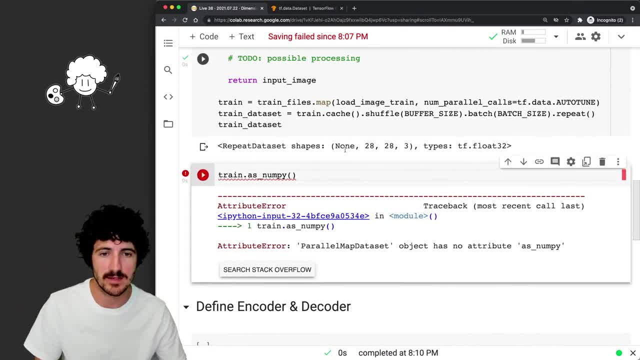 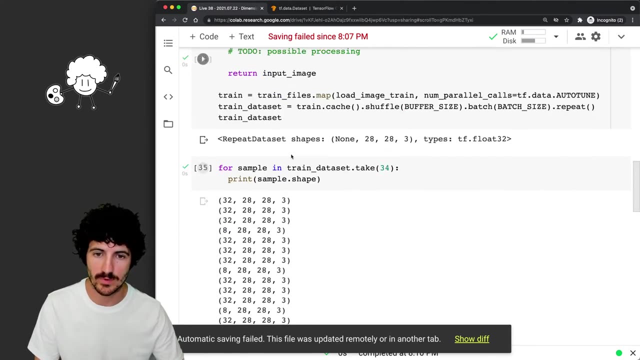 this gives us something different. So repeat data set shapes We can now do for sample in train Data set. take 128.. Well, let's, let's do just 34. green sample shape, All right. So we're getting batches and so let's say we just get 32 multiplied by three plus eight. 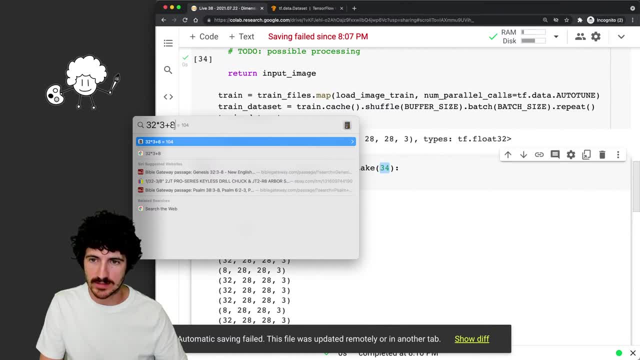 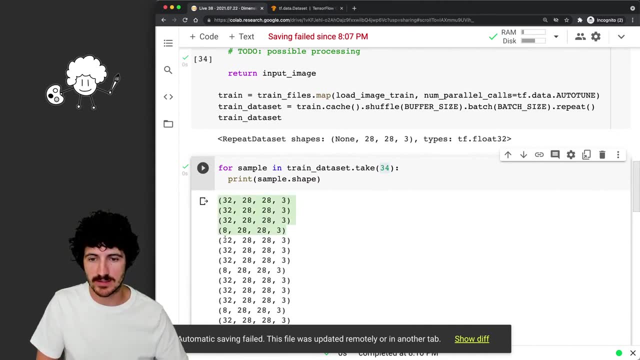 That is 104, right, So all we can get here is these four batches And then we reset, because we only have 105 samples from the data set. They shuffle and then they start again here, because 105 we can not really well 35.. 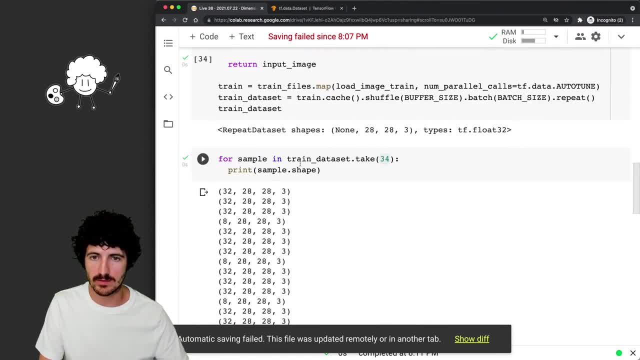 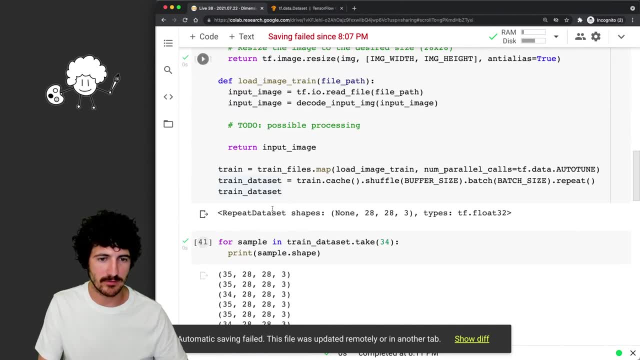 Okay, Okay, Okay. So our batch would be, for example, 35, and now maybe we still get- oh, because of the buffer size, 35. Well, we still get 34.. All right, Let's actually leave it here. 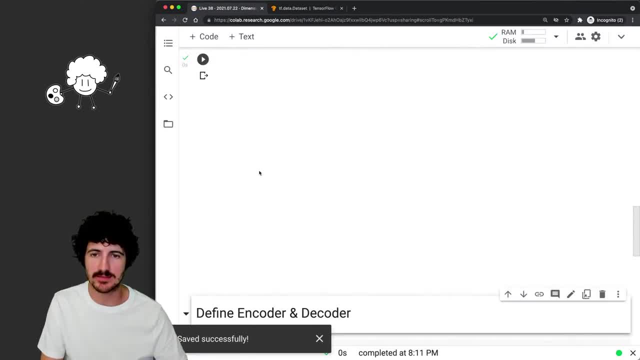 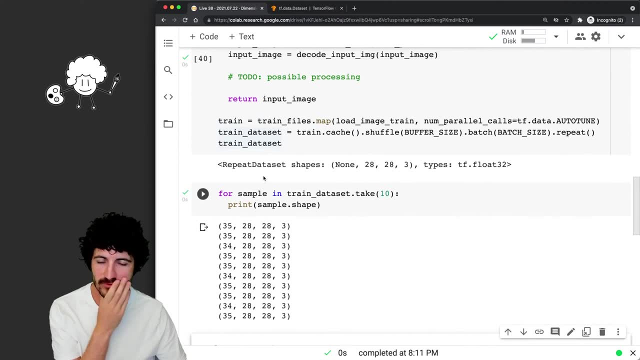 We can get many different batches, so we can say 10 batches and we'll have more, more samples here And um. we don't really need these data batch, but we have an RGB image. One thing that we can do here is: 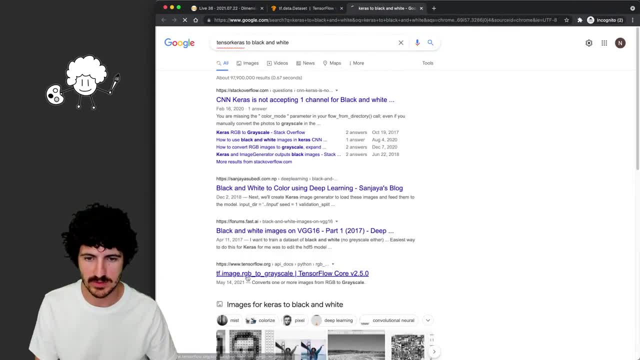 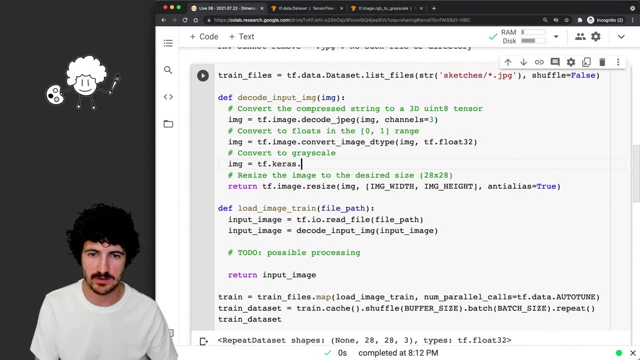 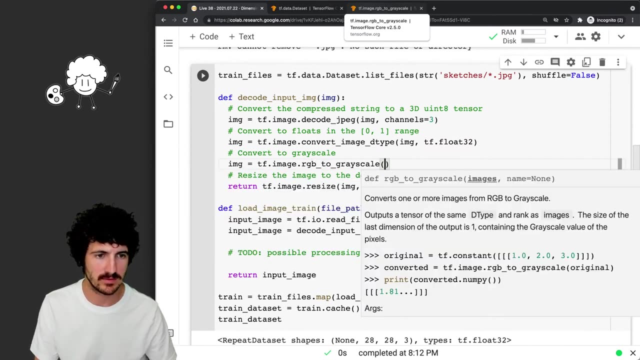 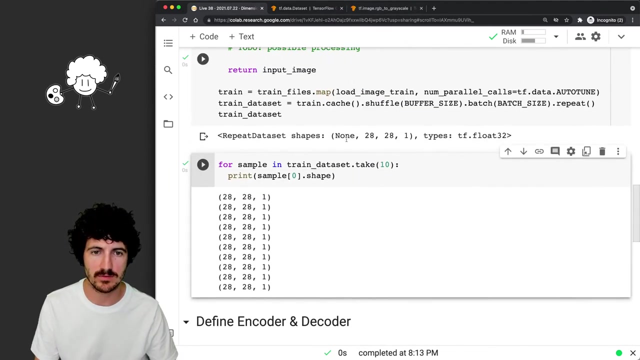 So Keras to black and white, the RGB to gray scale, So we can actually convert to gray scale. So TF Keras image, RGB to gray scale image. All right, Let's try that out. Now we do have the shape that we wanted. 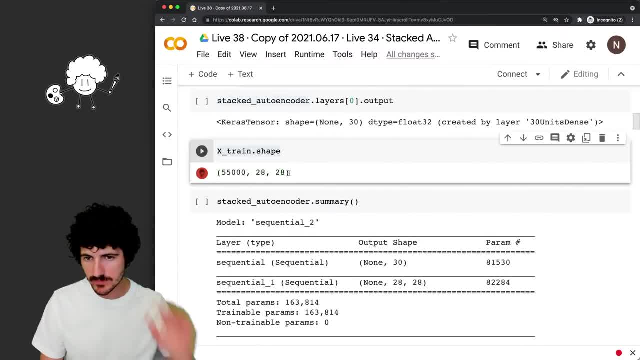 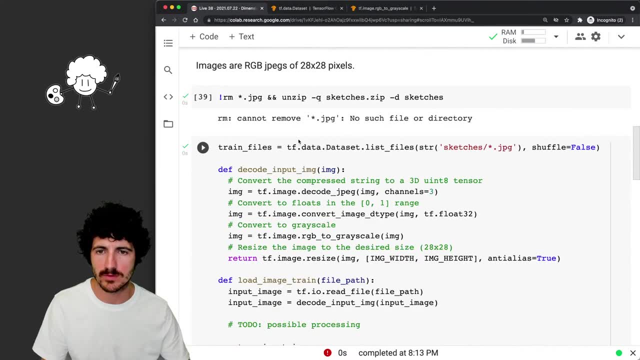 So now these are going to be the same proportions, So 28 by 28.. We can bring this all to to all the other notebook. Let's just try to be back with this. All right, So we have this here, Okay. 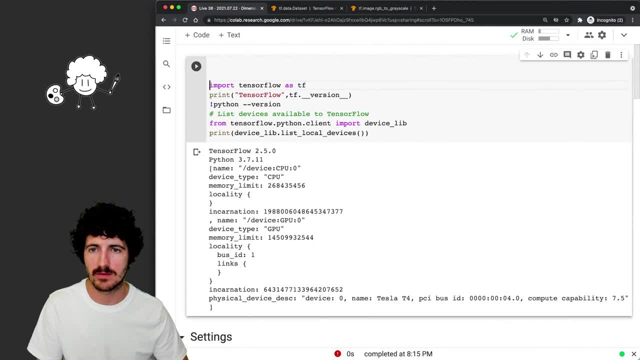 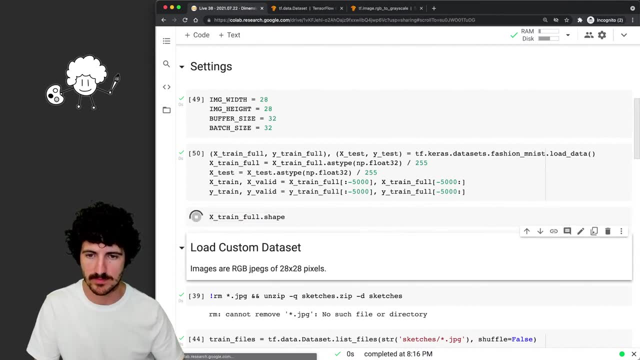 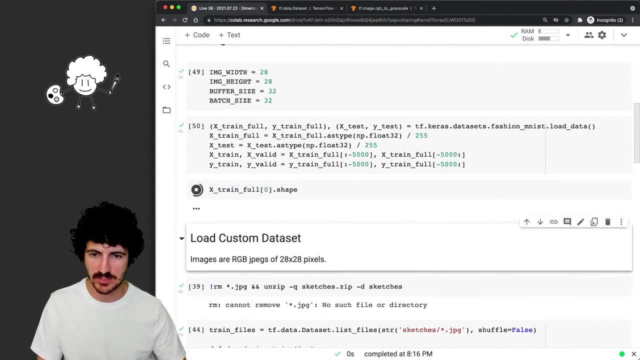 Import, maybe import numpy SMP, And here we have, for example, X train, full shape. Okay, So this is a 6,000 of 28 by 28.. So we get The first one. what's the shape? 28 by 28.. 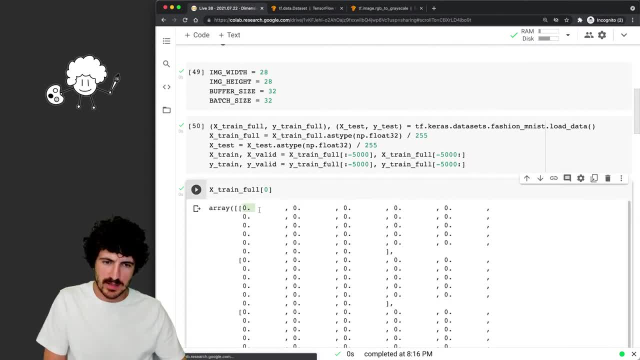 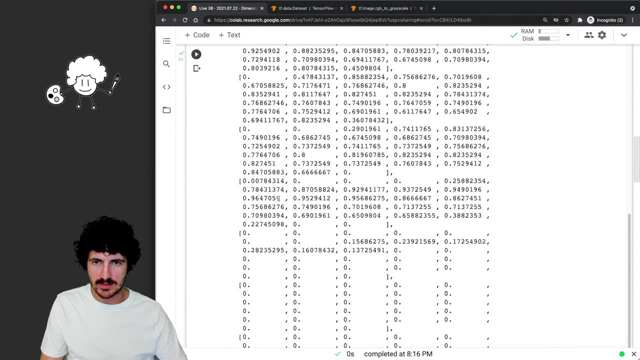 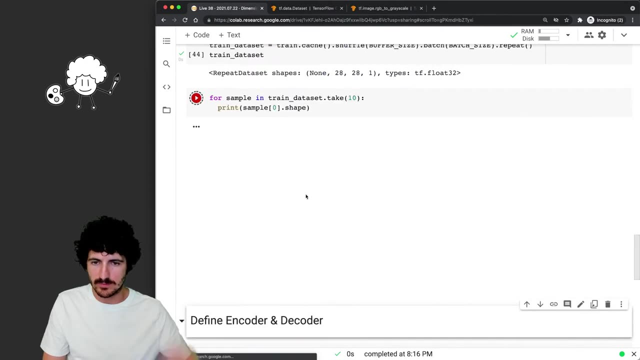 And if we print it, 28 by 28,, so there's 28 items of 28 digits. If we do have something that is like our data right, We have here The sample: 28,, 28, one. So these means let's, let's just print it. 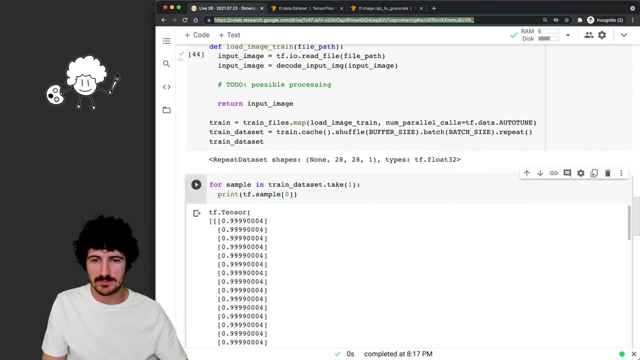 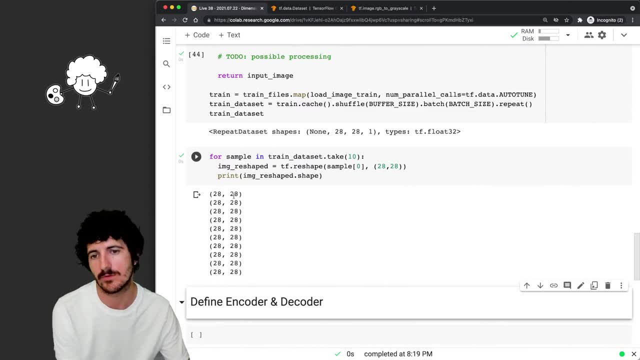 So let's take this one batch. This is the opposite of expand. We have the sample now here that we've reshaped, So we get 10, you just get all of those. All right, We have a way in which we can do that. 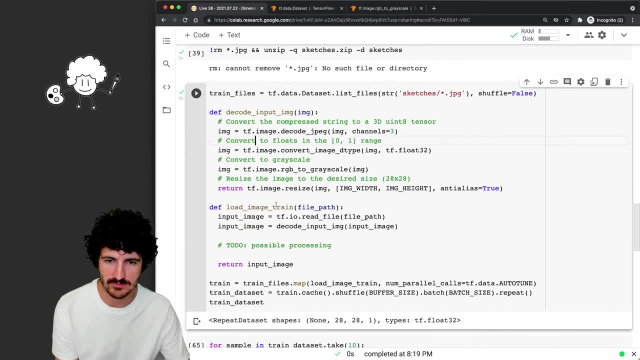 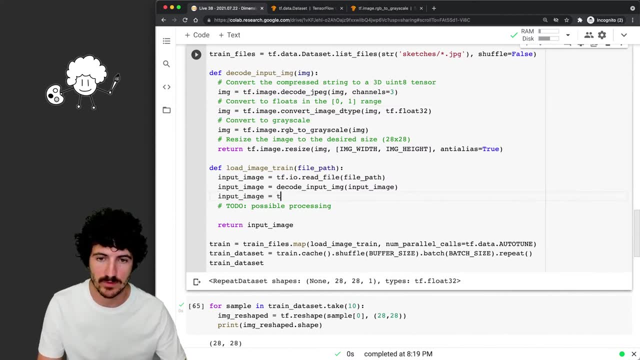 We probably want to, because this is returning the images and here we're decoding the input. So maybe input image. here we do the reshape and we say that our input image is going to be reshaped to 28 by 28.. Let's see if this works. 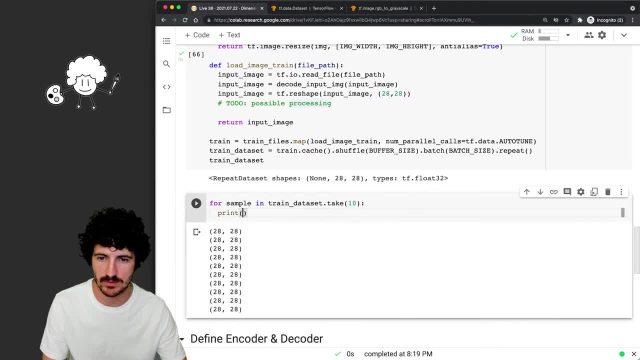 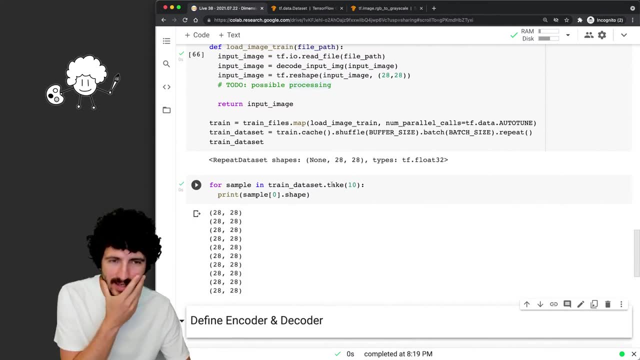 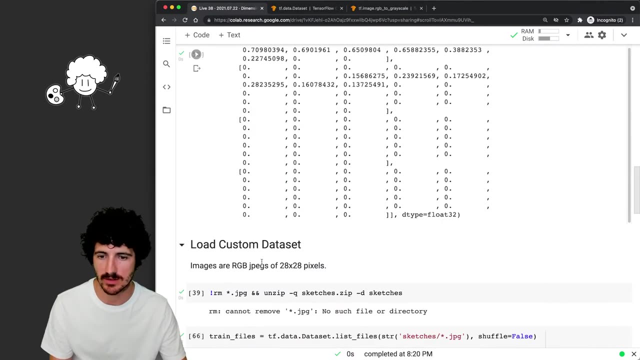 All right, Nice, Now we don't need to do any reshaping, So we just print the sample shape. Our data set has a set of images that are 28 by 28.. And I guess individually each of these is 32 by 28,, 28,, which we saw up there. 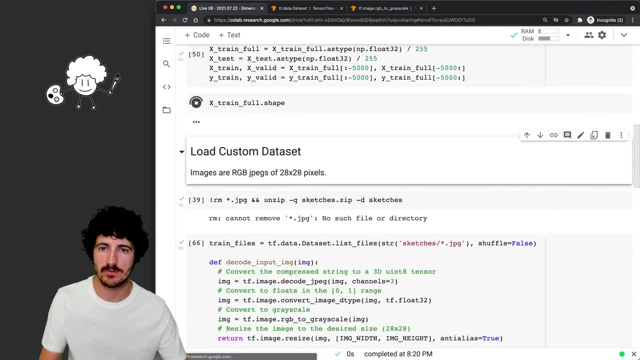 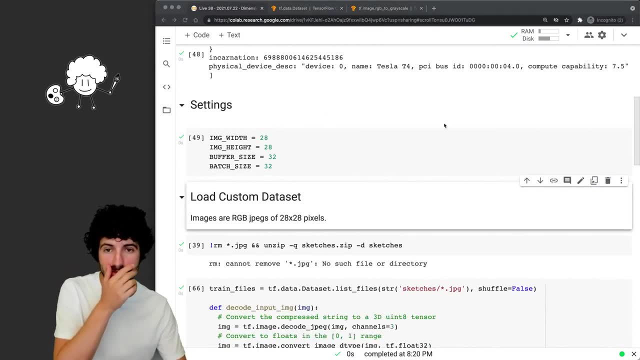 What's the shape of this? 28 by 28 and the full is 6,000.. All right, Awesome. So we're loading our data set in a good way that we can now use it. We're trying to load a data. 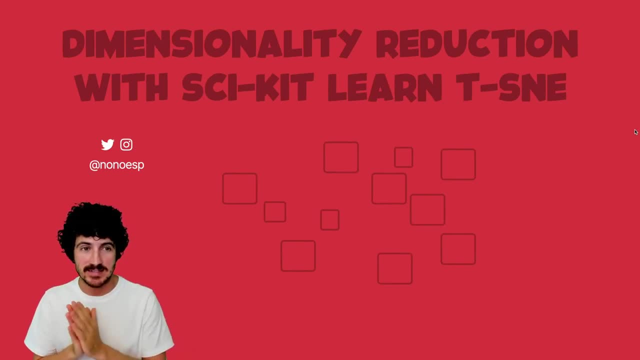 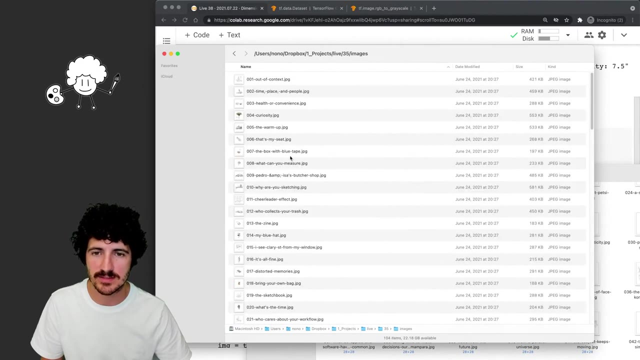 Set to do a dimensionality reduction exercise with the Disney implementation that comes with scikit-learn. So we're loading these images in 28 by 28 size, really small to see with your eyes, right? These are super, super, um small images that are pixelated and we drag and drop. 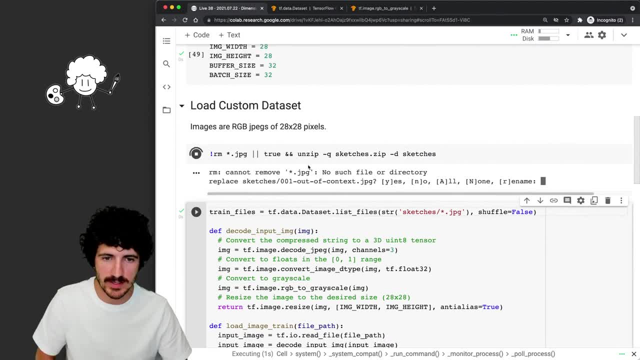 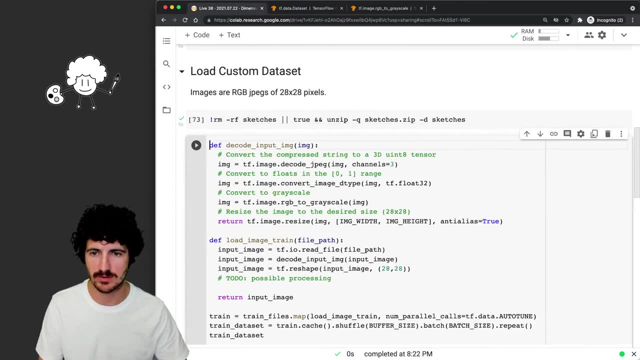 those to here as a zip file. So we unzip those files. These removes the folder and then unzips- Great, So we load the data set here. We actually don't need to do this here. We can put these functions. We have the data set here. 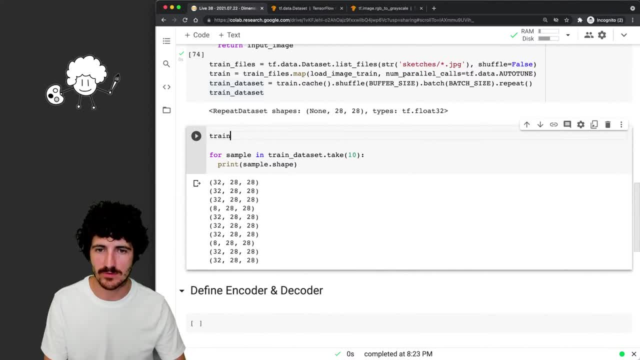 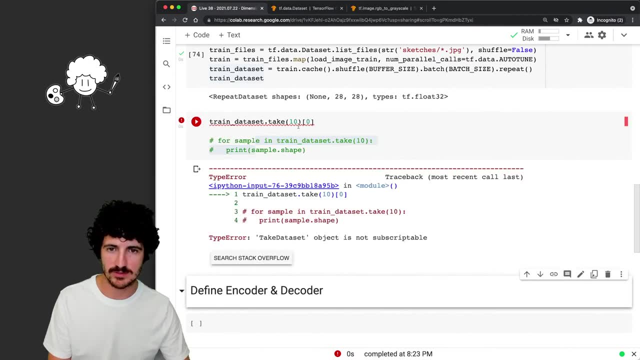 Here we can load a set of things. So if I do train data set, take 10 and I get the first one. let's comment this out. Take that to say it's not so scriptable. All right, We made that on an object that is not going to end up any time. 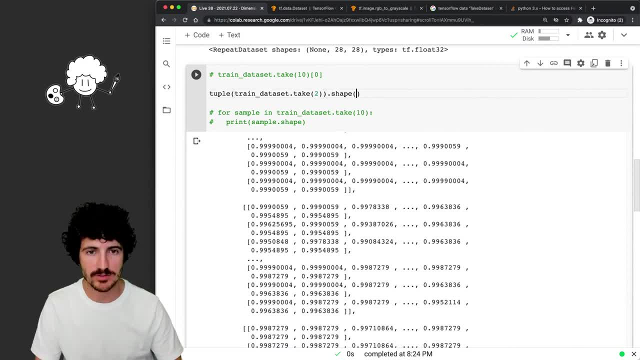 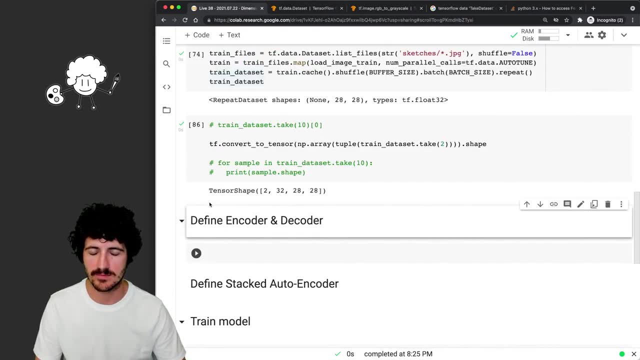 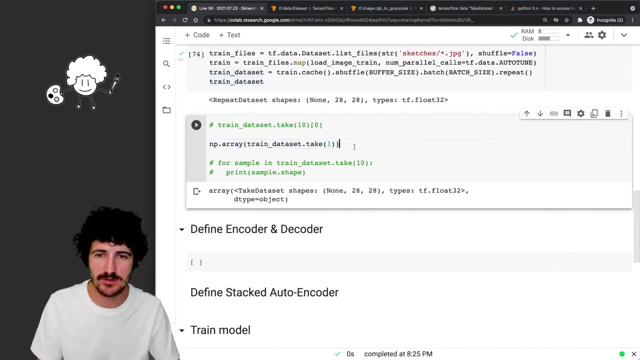 So maybe just make it into awesome. So let's see shape Convert to tensor, right? I don't know this. This seems a bit like a hack, but I might get there. All I'm trying to do is get the um, the, the data set that we have here, right? 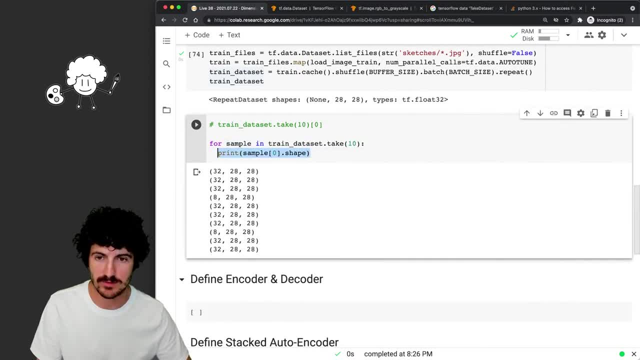 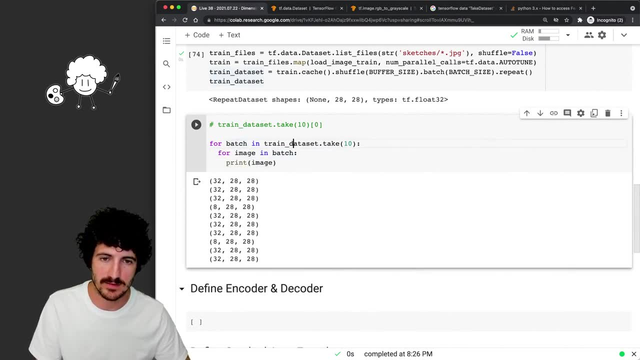 So we have a data set and if we get the, let's say the, this is actually a batch on our data. So for image, in batch we can print the image and maybe we just take one batch. So we have the image. shape is 20.. 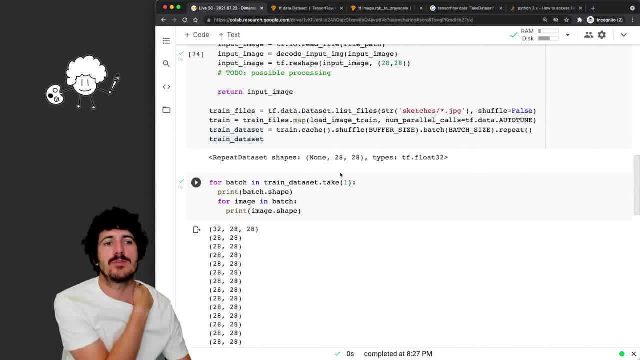 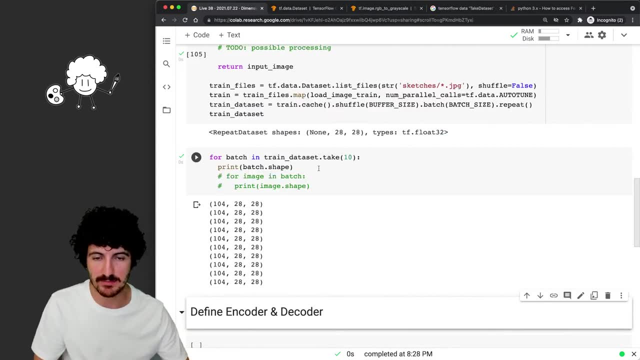 By 28 and we could actually plot this. Let's see what we can get. Um, not sure if I can do here a prefetch, here I'm getting at least a batch, so we can say: can I get just the first batch? 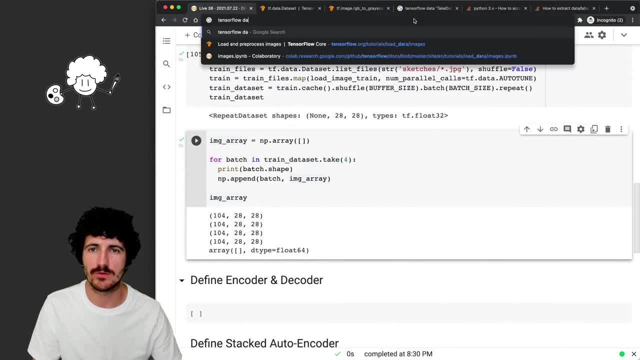 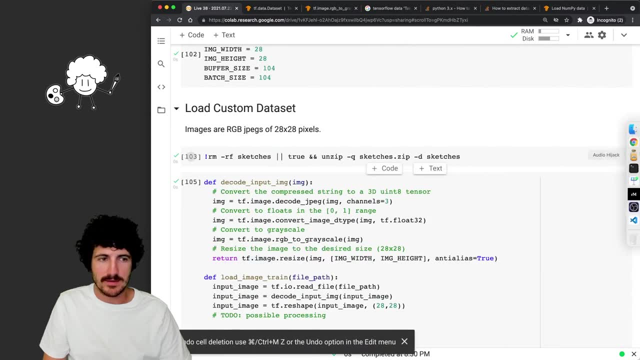 All right, I think these might work for now. Right, Thanks for full data set to an empire. right, We have the train data set, We can train with that and it seems like that's going to be okay. So let's say we just load the data manually. 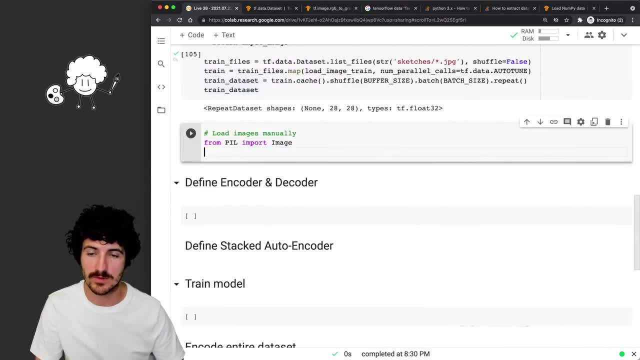 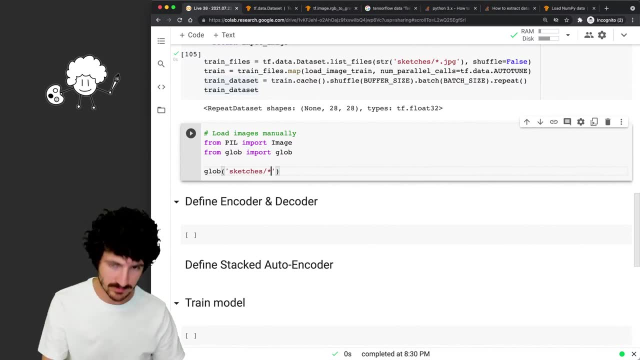 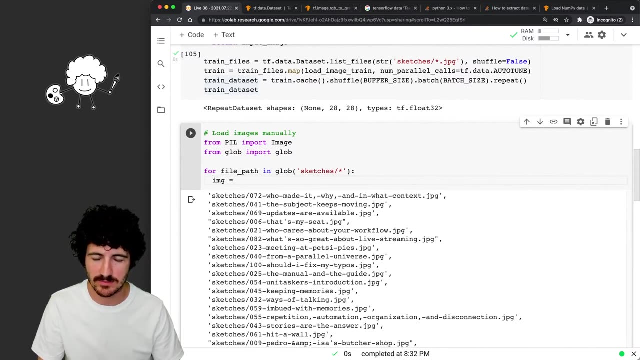 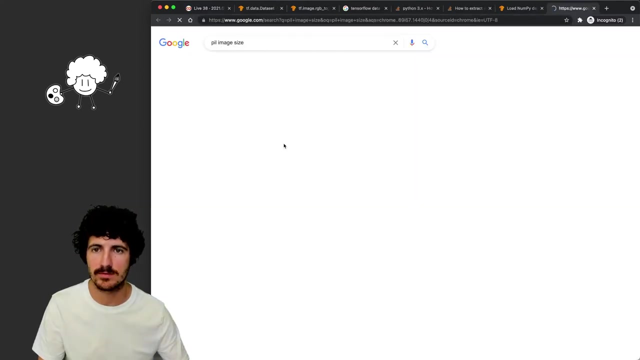 So load images, Man Only import image. So we can do import glove from glove, import glove. We do glove sketches. We get all the paths right. So for file path, in this we can say our image is going to be image open file path and we can print, for example, the image with image size. 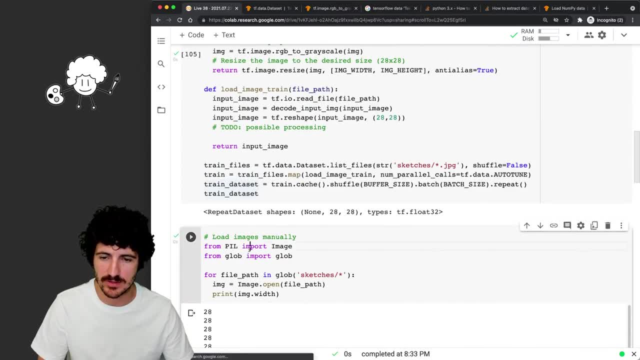 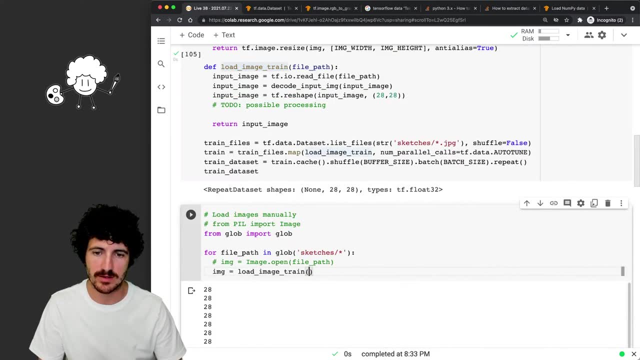 So it's 28 by 28.. Once we have the bath- actually even if we don't use spill, we do have these load image Train, So we can do load image train and then we put here that the file path, and then we can say print image shape. 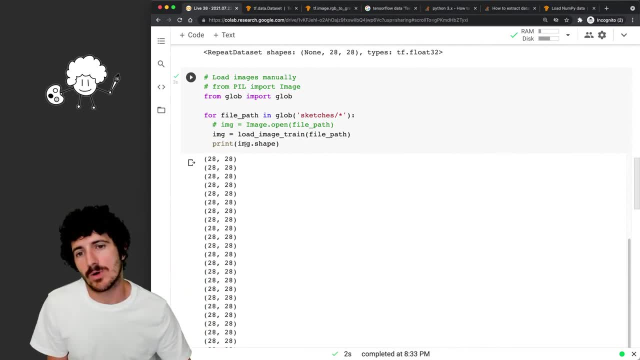 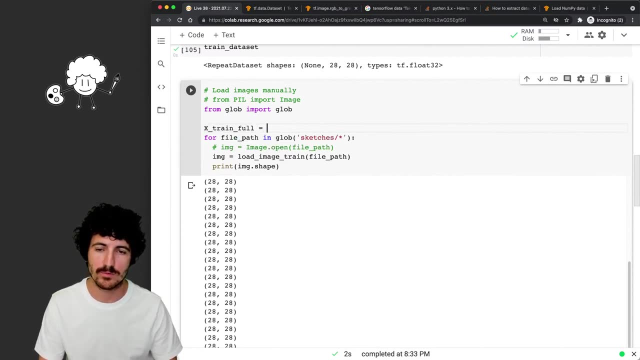 Do we get? images are 28 by 28.. That's well, we could say: okay, are like, let's say, X train full, could be that, And we just do X train full, append and this image, and then we print X train for shape, which I think. 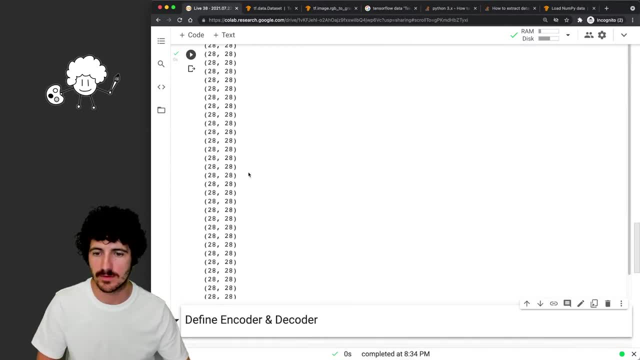 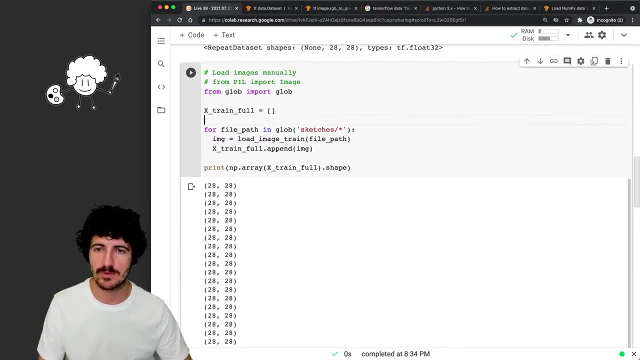 We need to make into an MPI right. All right, So we do get the shape that we want it. We don't need to print here, So we're just appending. We don't need pill, Right. So this is what I wanted to do. 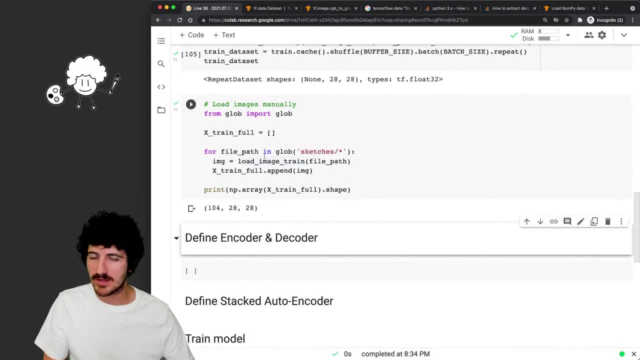 I wanted to try to do it with with the TF data library, And once we have these are also black and white. these are the type that we wanted, And so we could say: data, So DCs, So our data is going to be this right. 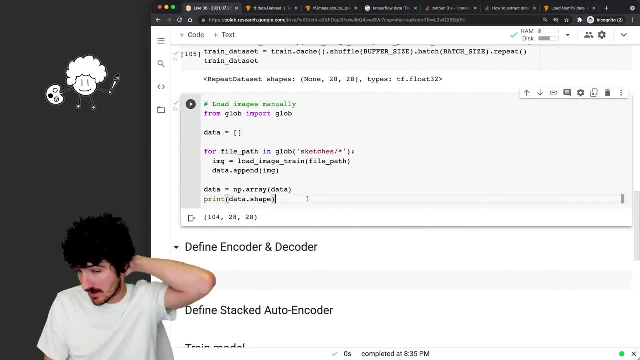 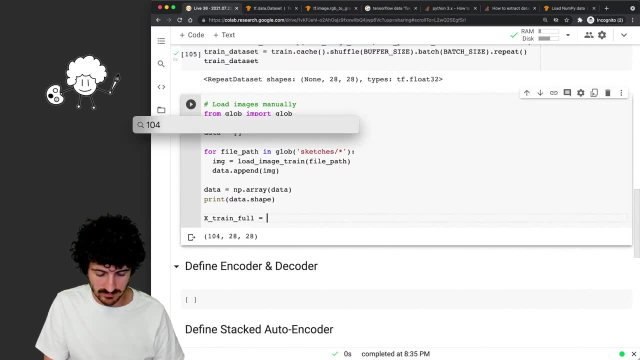 And then we can say, okay, we have data on the shape of this And because we don't have more data, we're going to have to say X train full is going to be so a hundred I'm five, 104.. 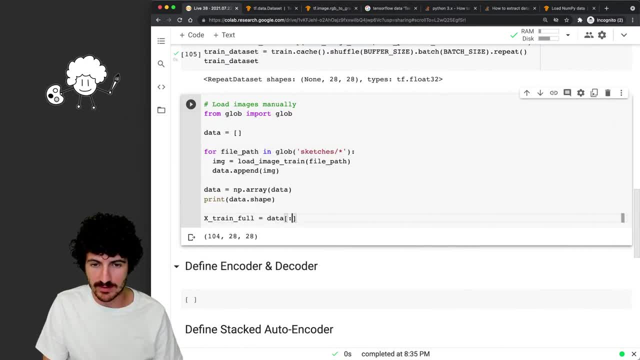 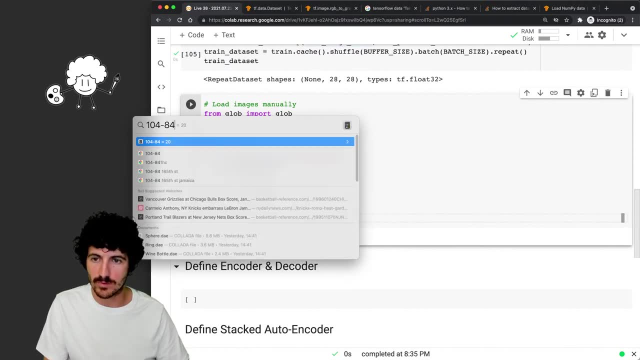 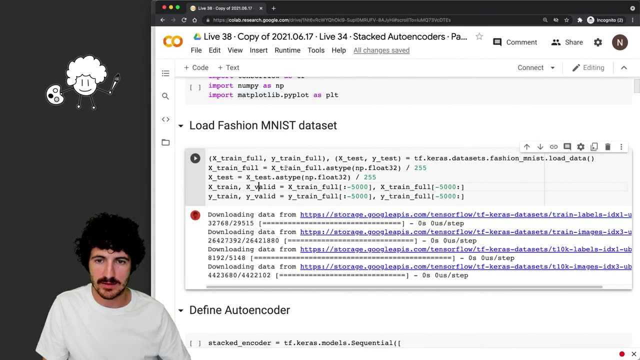 I'm not sure why it is a hundred and four. We do here data and we get the first 104 multiplied by 80. So let's do 84. So we leave 20 X ballot. All right, So extreme Full is going to be. just is the data and why train full? 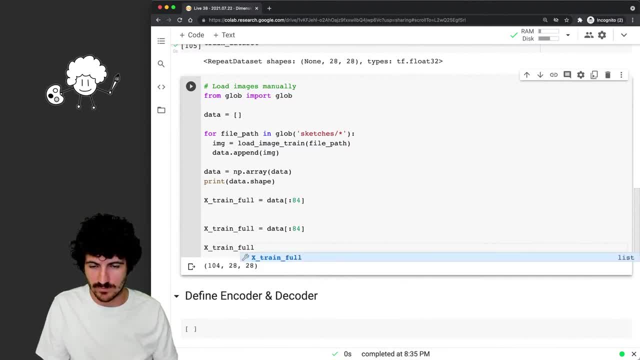 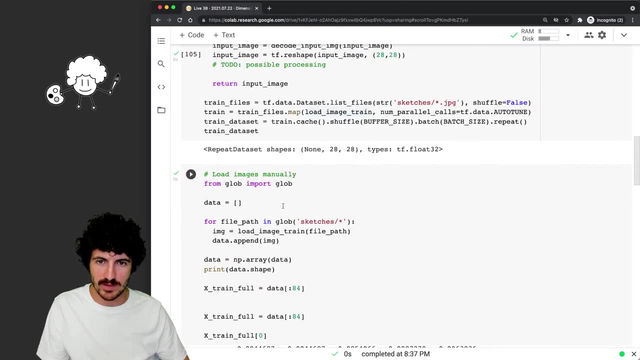 So we get here, we get the X train for zero. They're already converted to D type. That is what they're doing here. to flow: 32 divided by two, 55. That's what we were doing here, So we don't need to do that. 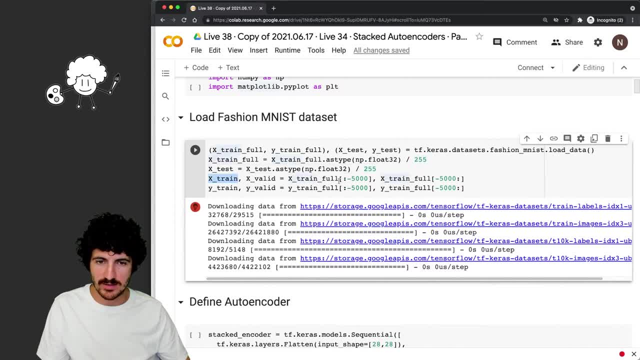 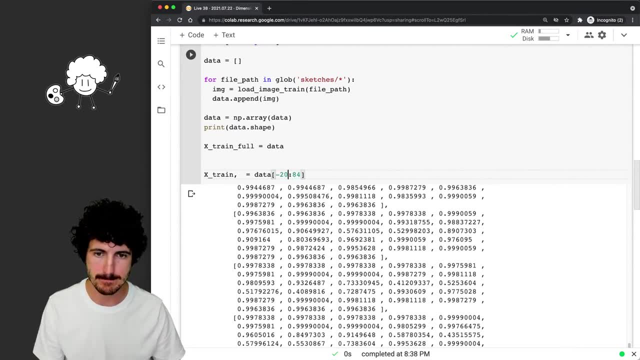 So all the data, and now we have X train, white train, So we get here X train, So we're going to get here. Um, Man is 20 dates. So extreme for extreme for minus 20, and this would be X ballot. 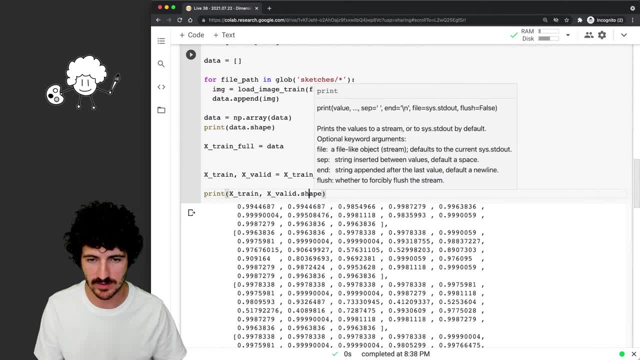 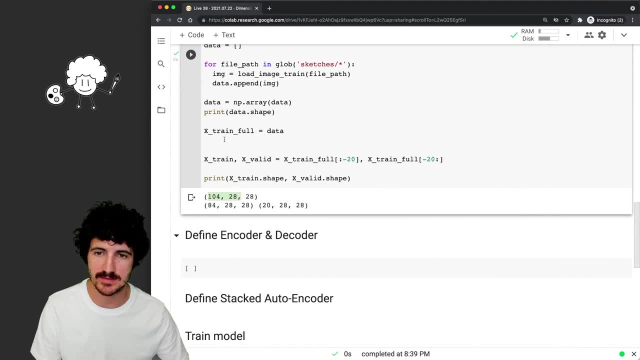 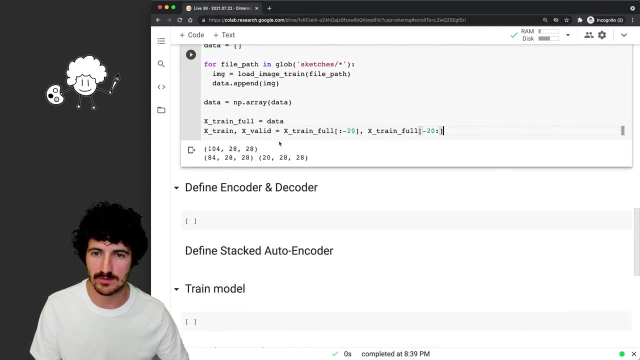 And we'll print here: X train, X ballot shapes, shape train, probably the other way around. All right, So we got the entire data set. is this shape? Then we have all the data and then we have the training and the validation data set. 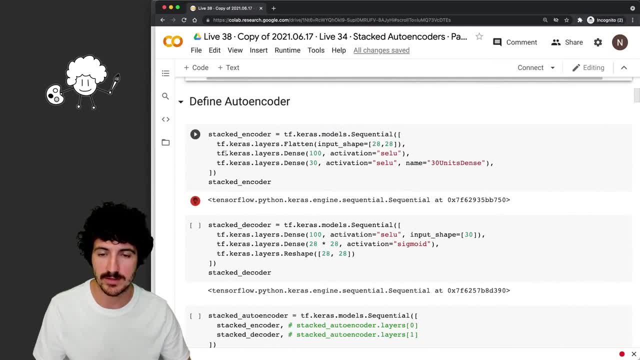 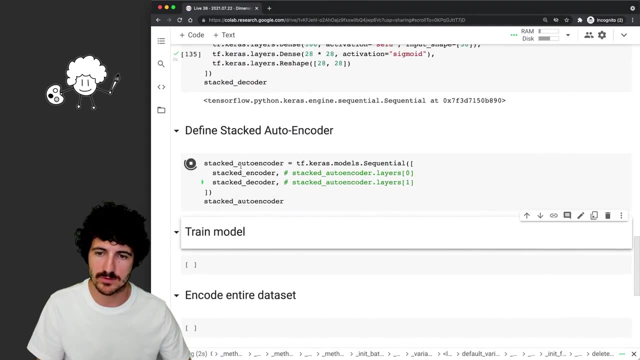 Cool, So we can get the encoder, decoder, architecture. So we're going to copy and paste here for expediency, Otherwise we're not going to get there. We have the encoder and we have the decoder and we have the stacked out encoder which we're going to paste here. 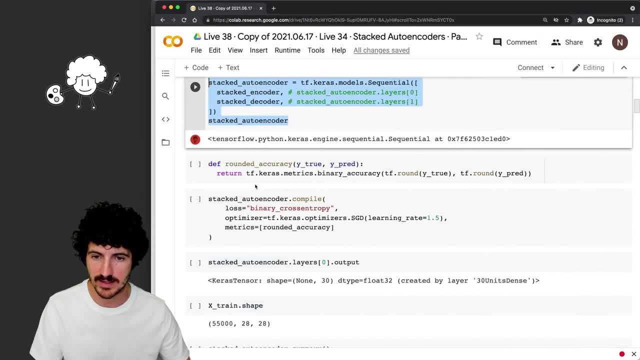 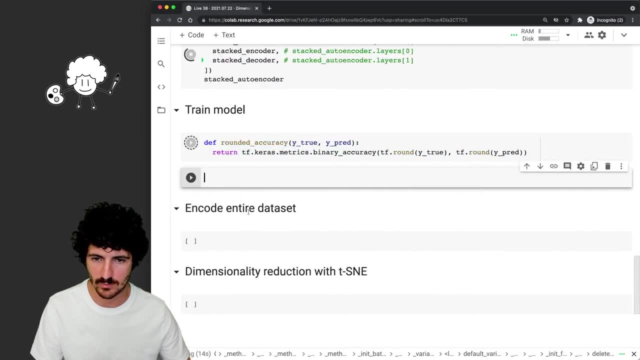 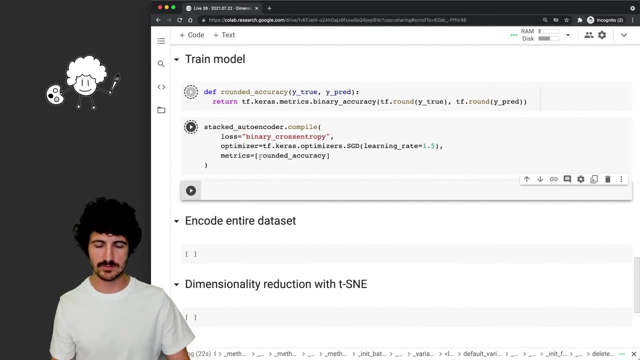 Awesome. So we have our stacked out encoder and now here we define that uh rounded accuracy, which is our custom metric. We compile the model with a binary cross entropy and this learning rate And our custom run that accuracy metric, So we could run everything above the cell. 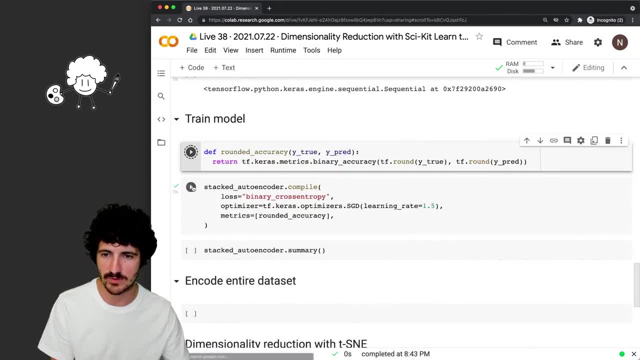 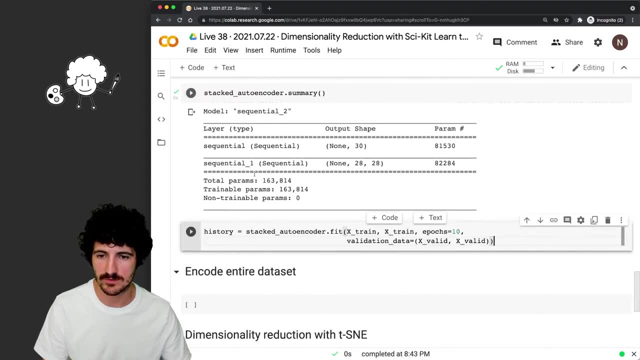 So run before we have our auto encoder, we define our metric, compile this, we get a summary of the model and we have to train now. So this is the actual cell that trains, and the input and the output data is the same. So the goal that we're trying to reach is the same. 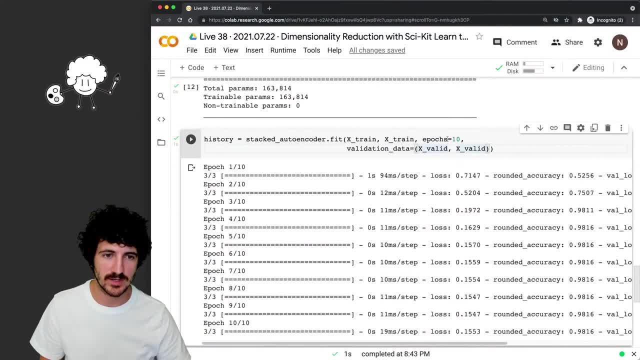 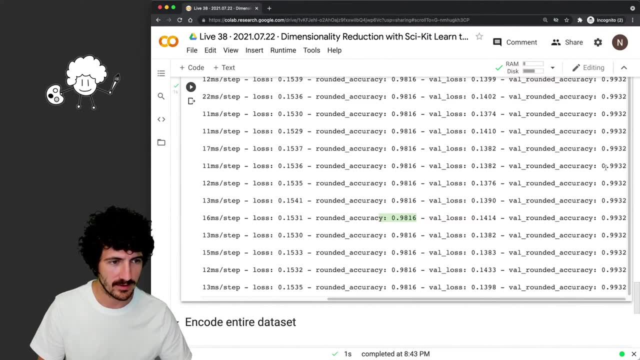 So we use the same input and output data set on one training. All right, So these super fast, So maybe we can train for More. It seems we might be overfitting there, because we don't really have too many samples. We just have 104 images. 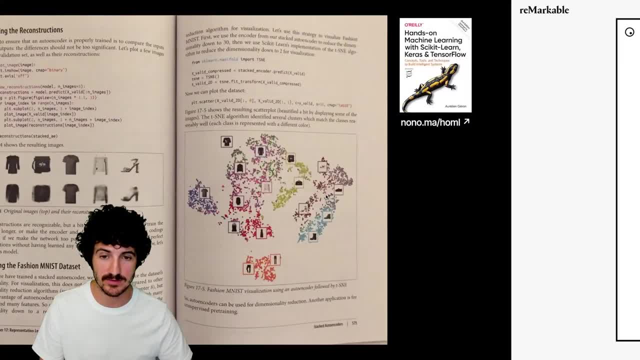 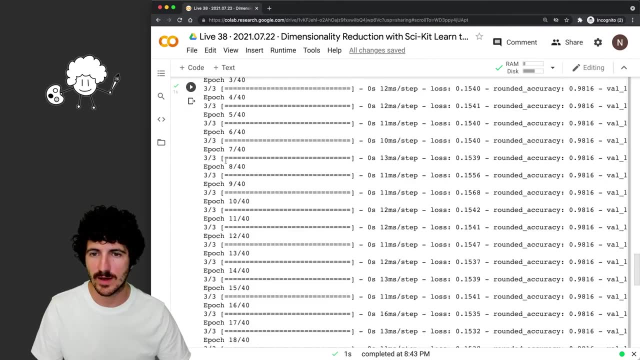 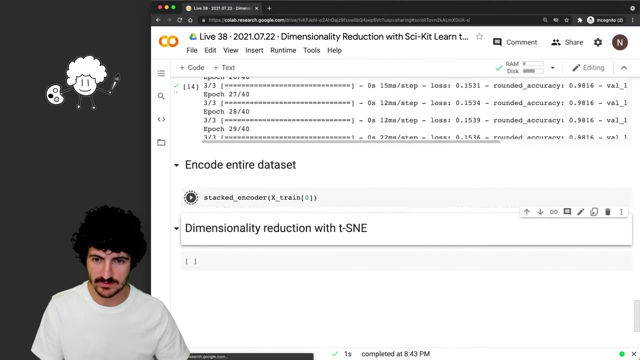 We have gone through this and this and now we need to see we can get the coatings so we could get a soup network of what we had before. So I believe we can pass an image through our stack encoder So we could X train zero. 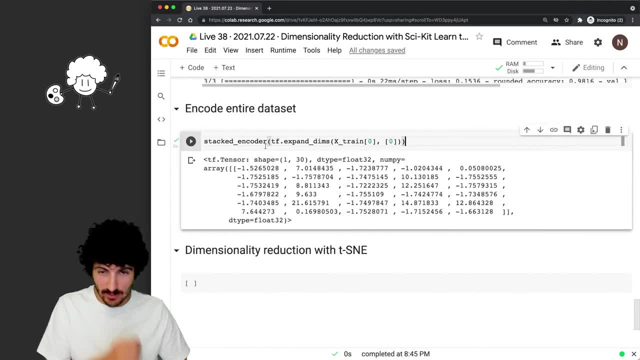 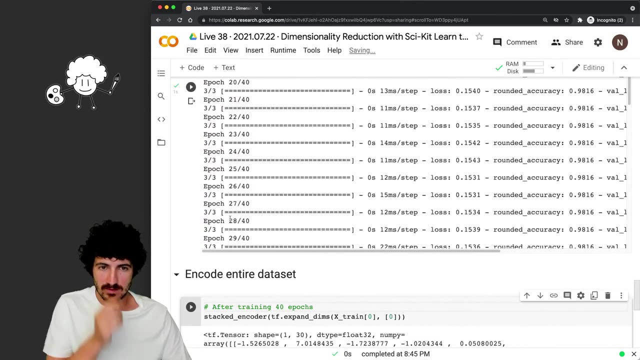 All right. So if we pass the image through the stack encoder, We're passing the first image on our data set. here we're getting the coatings, which are 30 digits and what I'm not completely sure. So this is, after training, 40 epochs. let's say we retrain. let's say we retrain for. well, if I retrain now, I think continue from where we were. 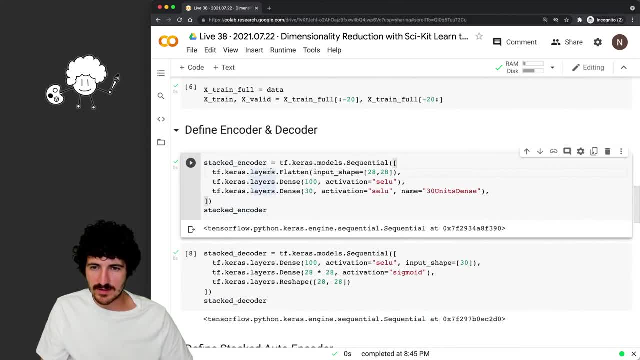 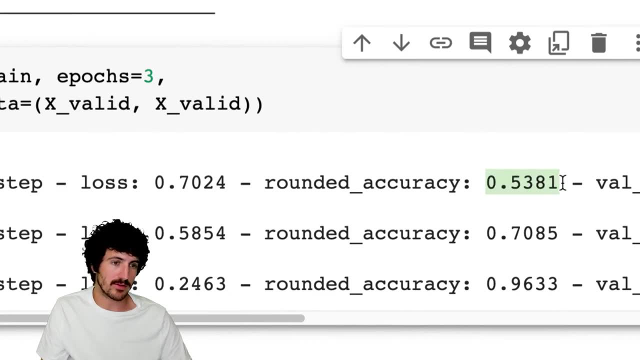 So we have the same accuracy. so we might need to reset our model here and train again. So you see that the accuracy is starting from I'm from, or if the run starts from 53,, 70 and 96, we get really fast. 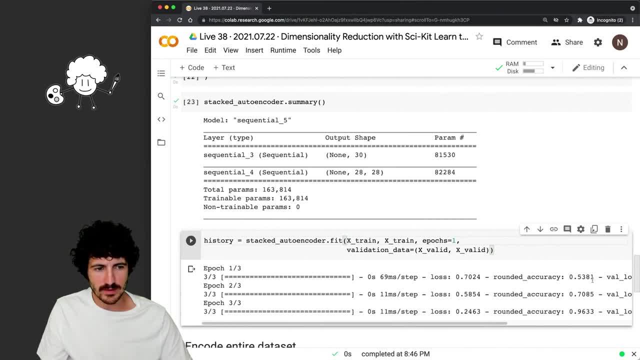 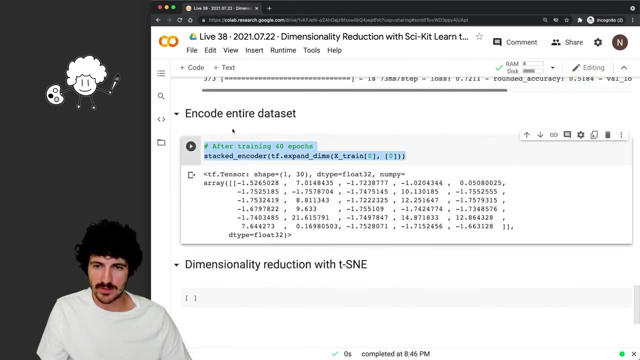 We get really high. So I'm just going to put here one. So we get just to this step and I'm going to go through all of the cells Again. we have this model here and this was with 40 epochs. We're going to try to do it now just with one epoch. 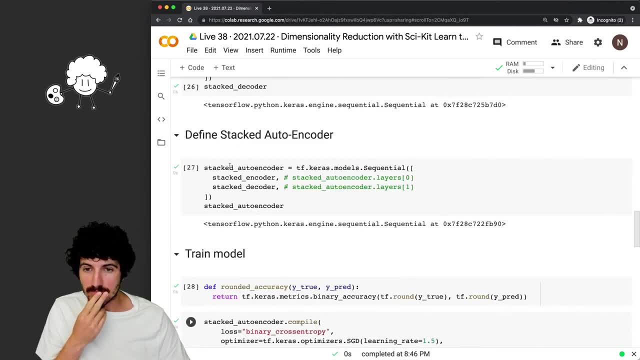 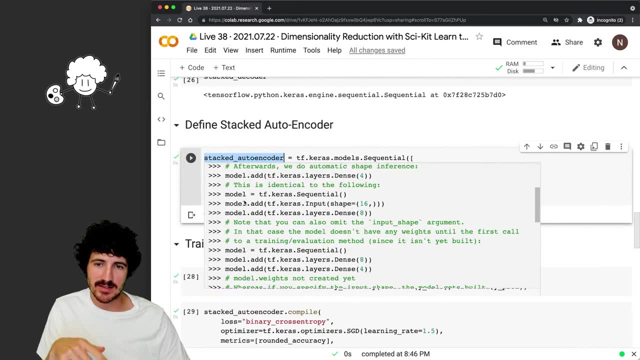 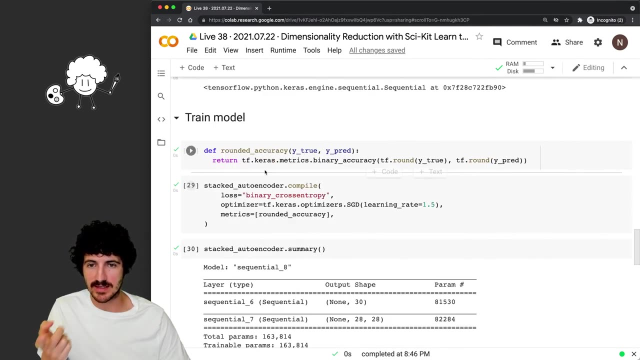 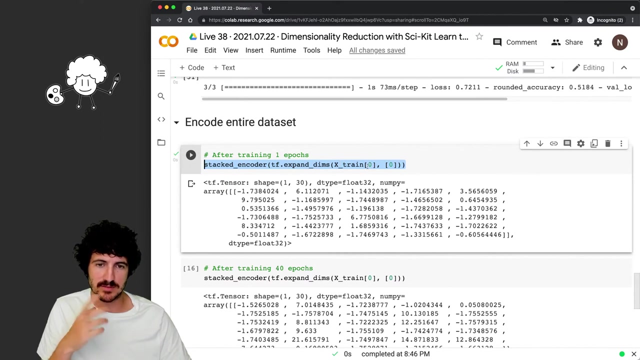 All right. So the encoder network right, which we defined here and we included here in the auto encoder, Has actually been trained and its weights have changed. So when we run this feat method, the auto encoder has inside the encoder and we actually have this network here that can get these image, this input image, that is 28 by 28 image, and then generate the coatings. 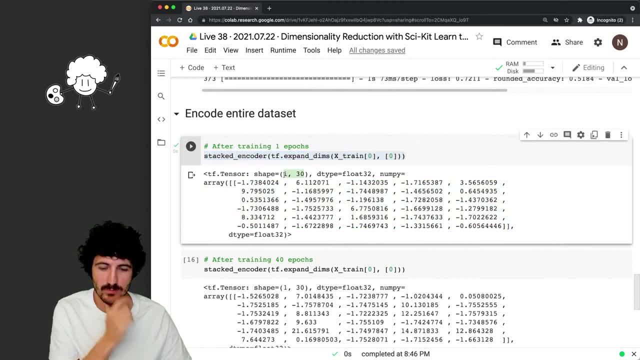 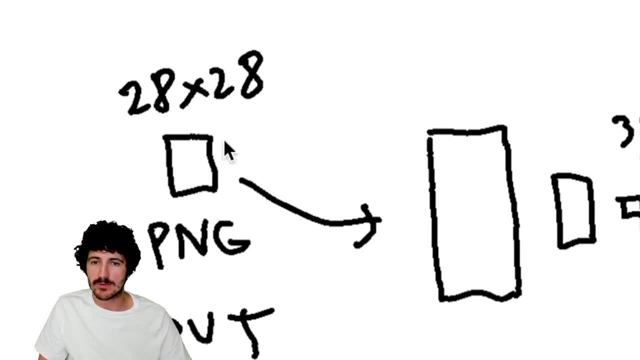 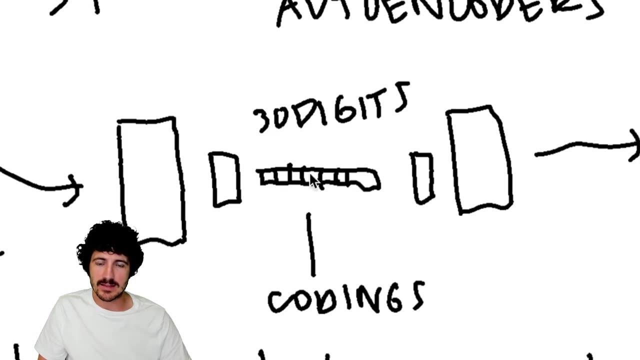 And what we have here now are 30 coatings right, What we talked about before. So these are those 30 coatings right. We were talking about a 28. By 28 image that was passing through a network. So we were training in this loop of encoder, decoder, and in the middle these encoder part ends up with 28 by 28 on the left and then 30 on the right. 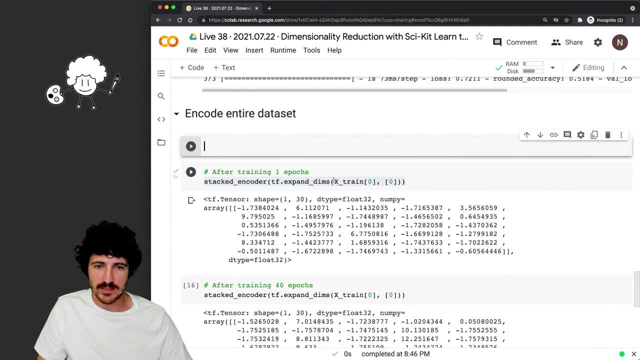 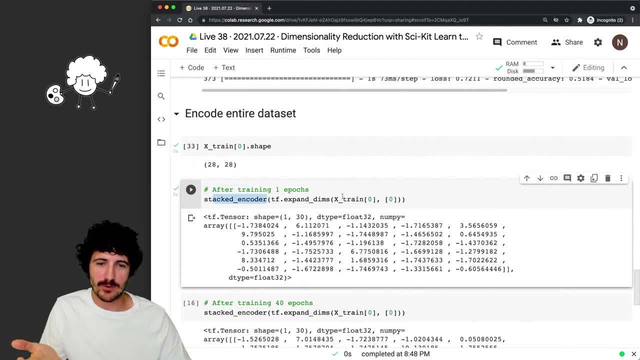 And we are actually seeing that here. So if we look at the shape of X-train, so we look here is 28 by 28.. I put it through the encoder and, as promised, if we get the shape of this, yeah, it's one by 30.. 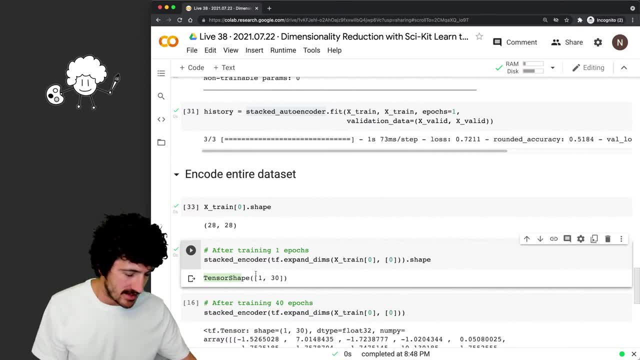 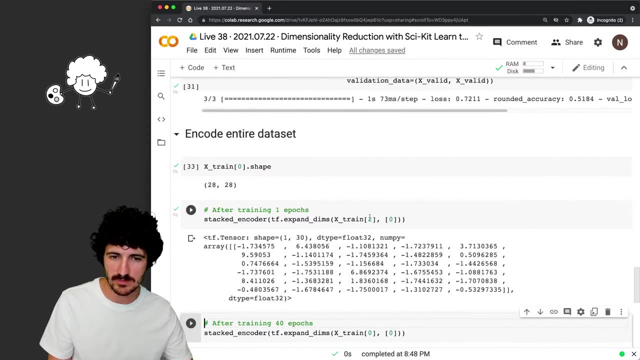 So It's a linear tensor that has 30 digits inside of it And you know promise achieved. if we change the, the input- So I'm taking different images here- The coatings on the bottom slightly change. They change a bit because the input is a different image. 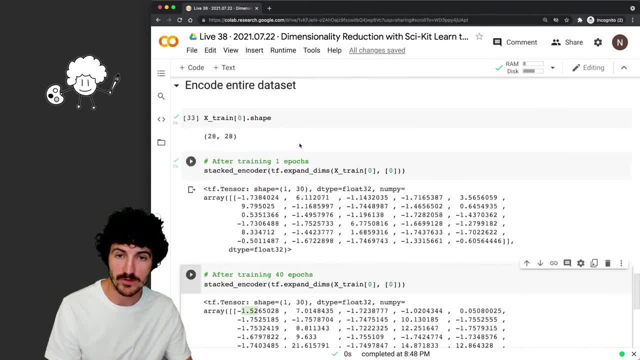 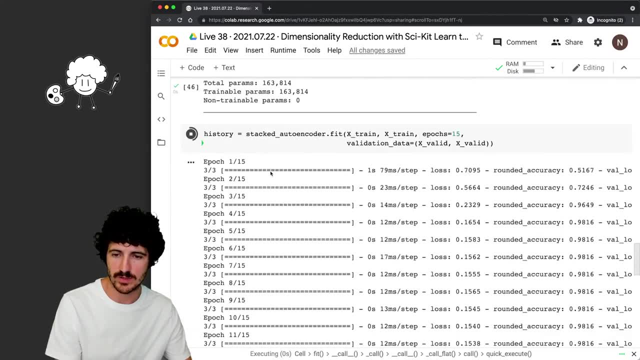 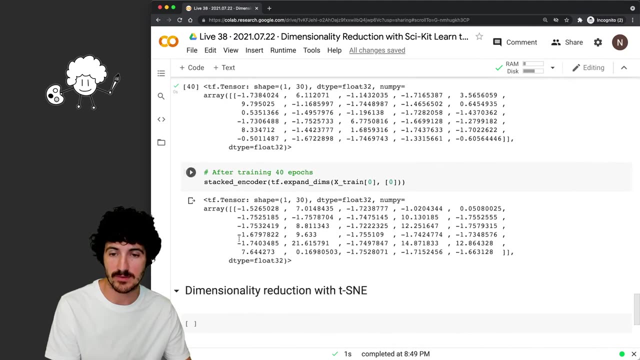 They're different, So one 73 and one 52. So I'm going to go to 15 epochs and I'm going to rerun the cells and retrain right. So we retrain there. Now our render accuracy is again at 98.16, which I believe is the same that we'll get if we go to 40 epochs. 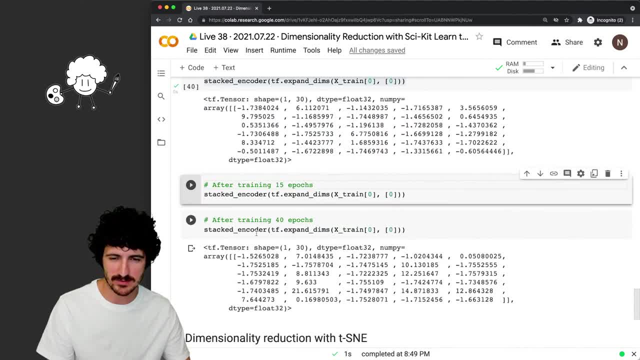 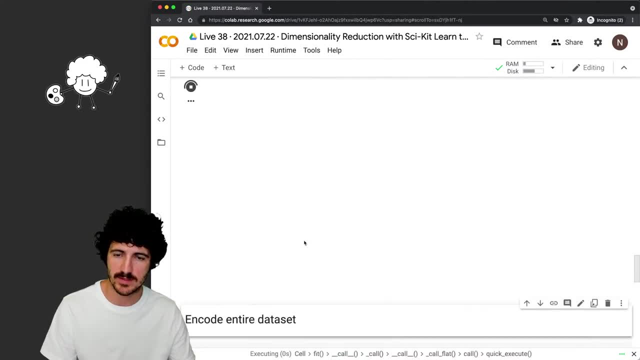 And what I'm going to do is that I'm going to put here 15 epochs, but I expect to see something similar to be low. Let's do actually 10 epochs and redefine everything from scratch here. So that's 10 epochs. 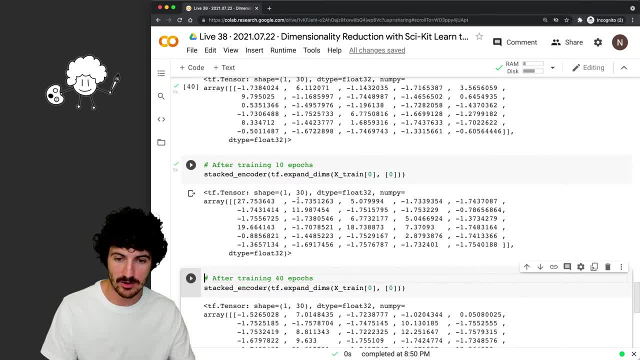 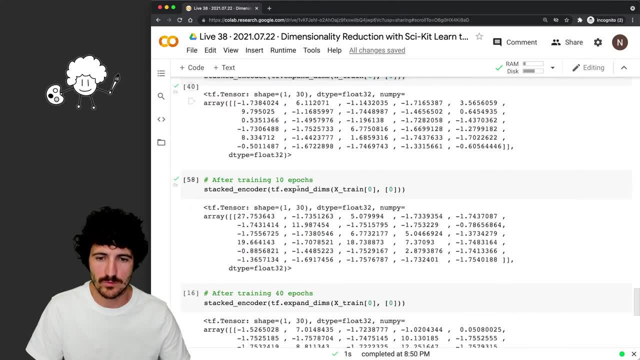 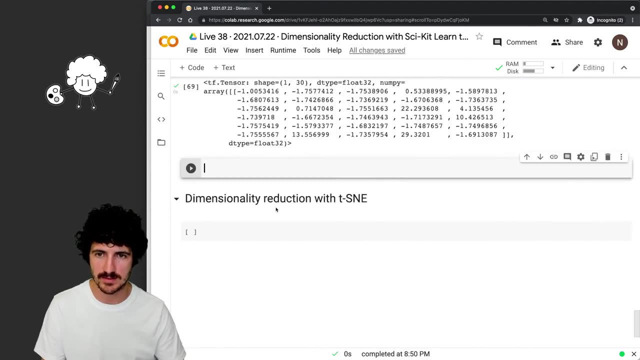 I'm going to put here 10 epochs and now we're going to put 40 epochs and I do think we need a larger dataset. So 40 epochs around this minus one, everything. One thing that we can do is that if we run this by the stock decoder, right? 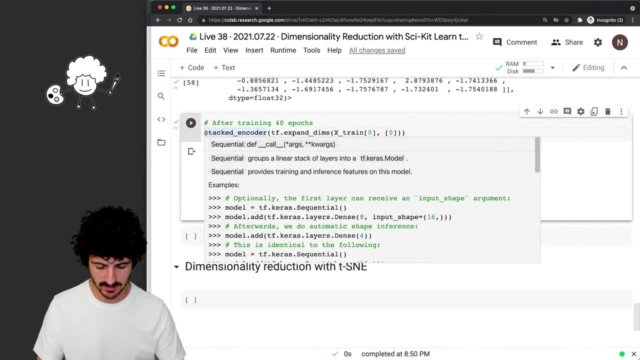 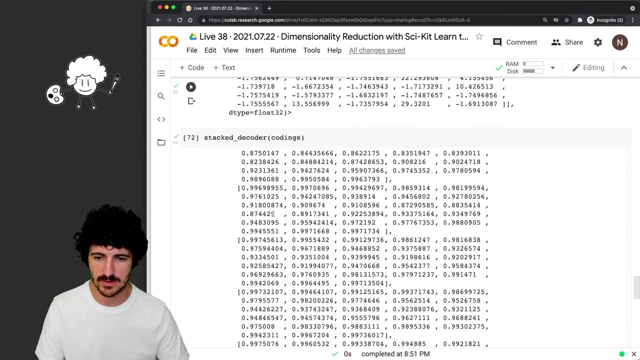 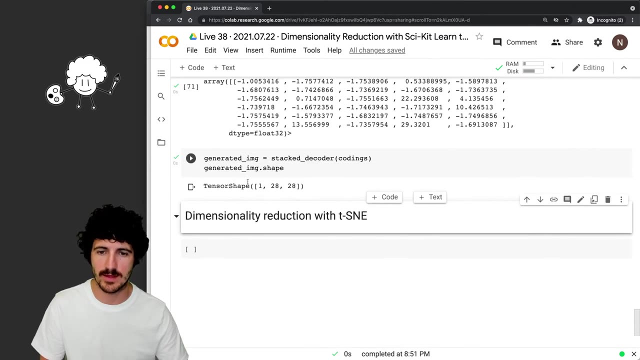 So if I now get this output from here- so let's say the coating, and I run this, my print coatings, you see them. So now I can pass the coatings back here and we get back. So this is a generated image. generate the image shape: right. 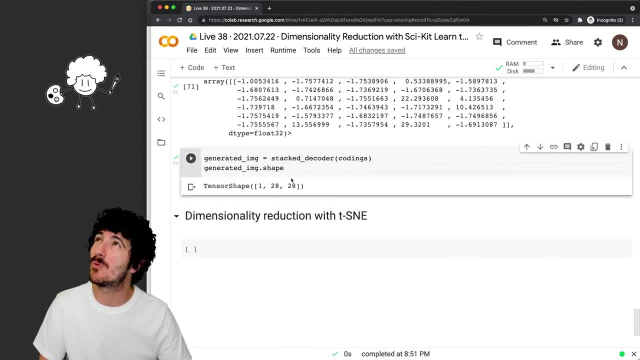 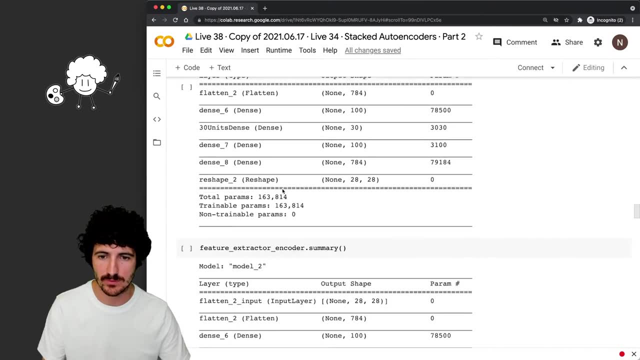 So that's again A 20 by 20 image. that is black and white, And if we get the first one of that batch, we get an image. So let's take a look at how to plot those, because I have the code here. 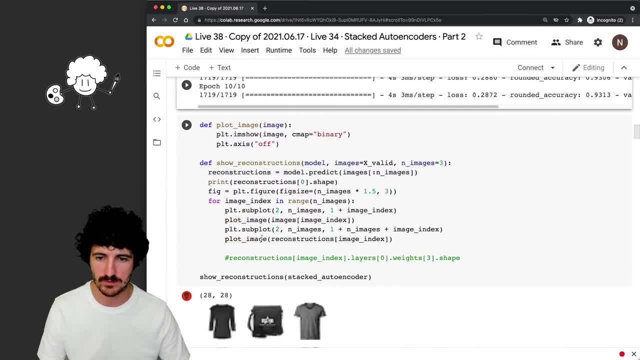 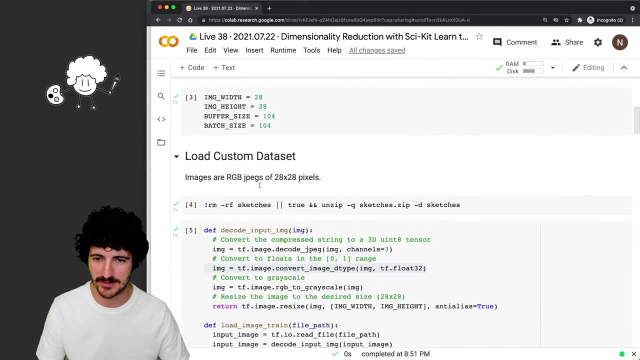 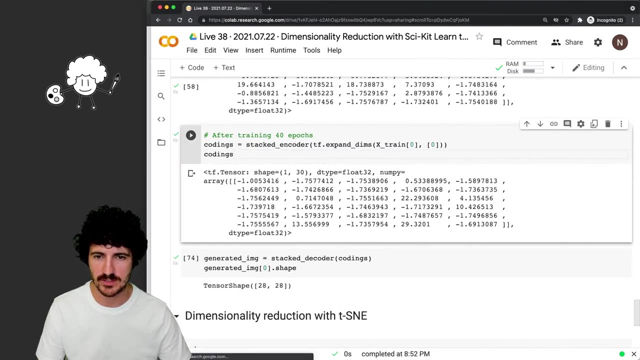 So plot image. we have a helper method, plot image- show reconstructions. right, We just need to put these helper and we'll have to do some cleanup. Not going to do it today. All right, Helper here, So we can plot the image and I'm not sure if these changes. 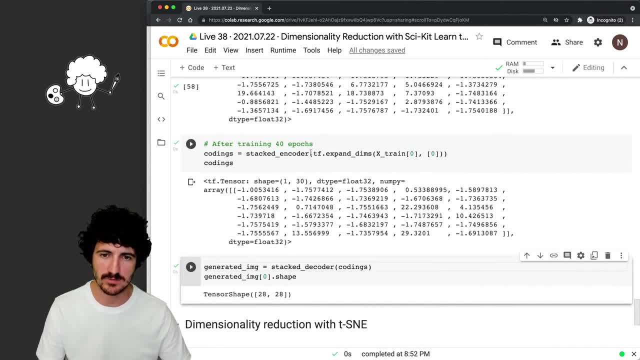 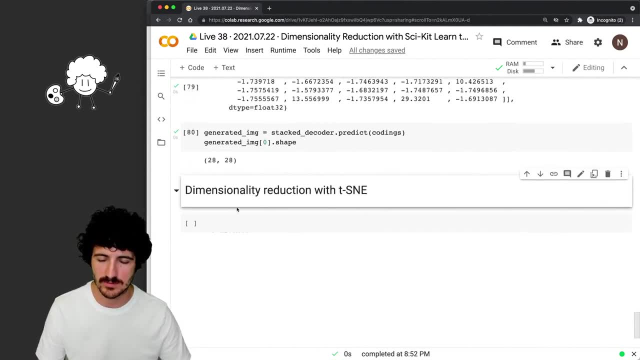 Okay, Anything, if I do here predict, I get a tensor, And then if I do predict, I get something different, but it's, at the end of the day, is the same result, And then I get an array as well. All right, 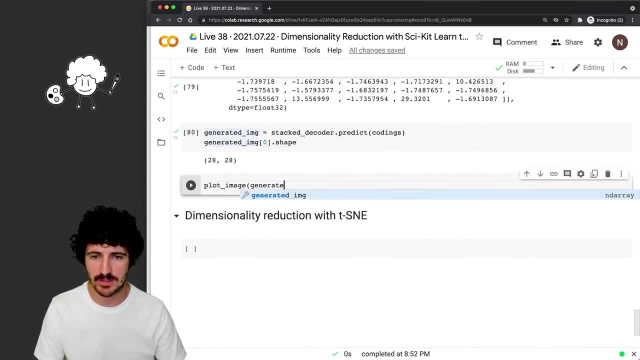 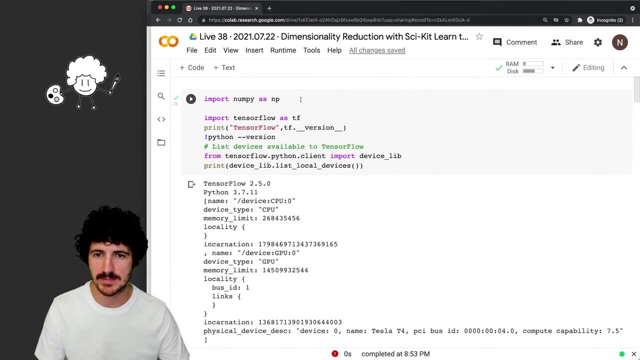 We wanted to plot this image right, So we're going to applaud the generated image. Let's see what that does. Plot is not defined. All right, PLT. We have another dependency and then we go back and we got our plot image. 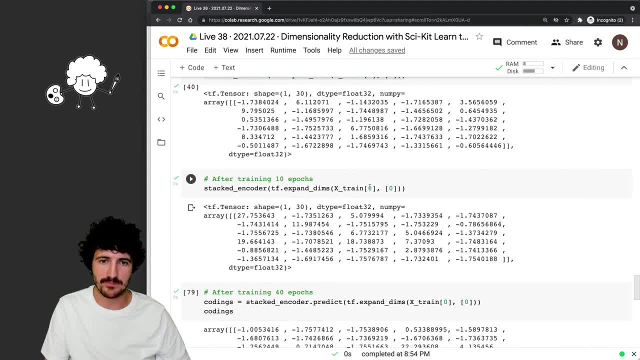 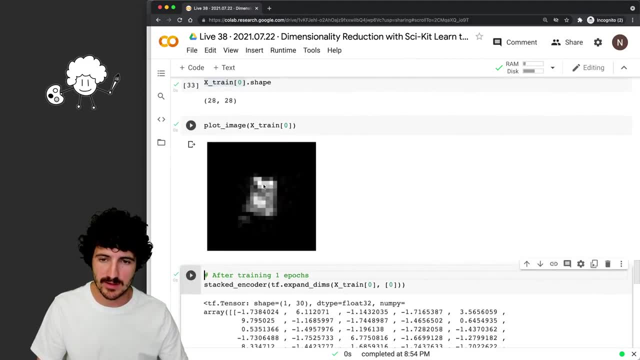 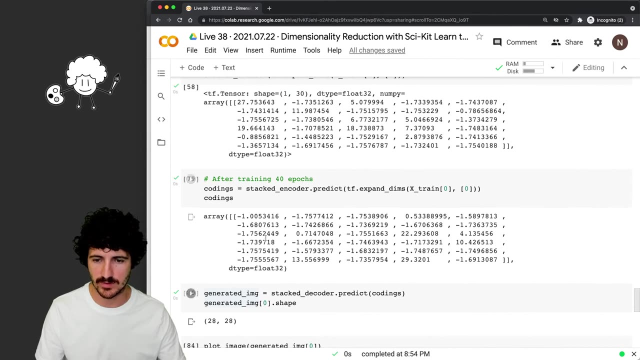 So it's learning something. We got them The input that we're using here. we can also plot it. This is the input that we're inputting to the network And I think we also have something to plot: the digits- Maybe not, but digits- the coatings. 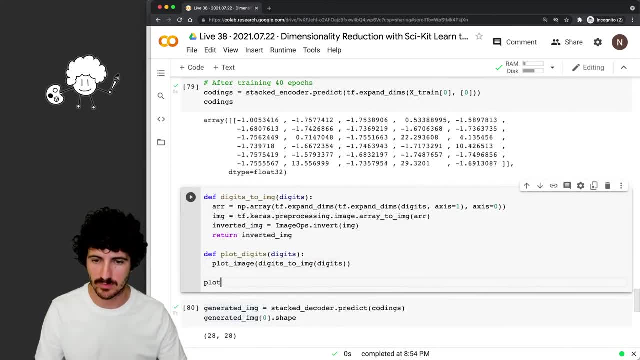 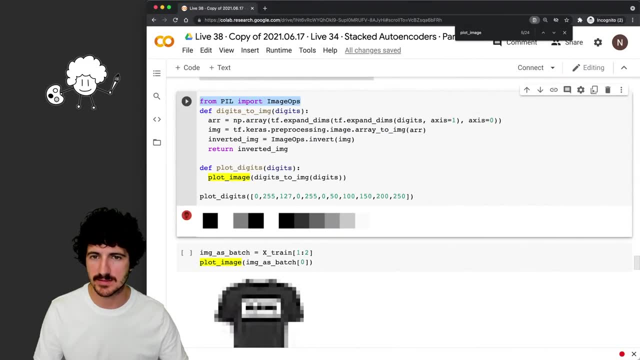 So if we plot here those coatings, so let's say but digits, and we do those coatings, zero, and we'll probably have to put all of these dependencies in the same place. All right, So those are my coatings. So they go from there: 30 digits. 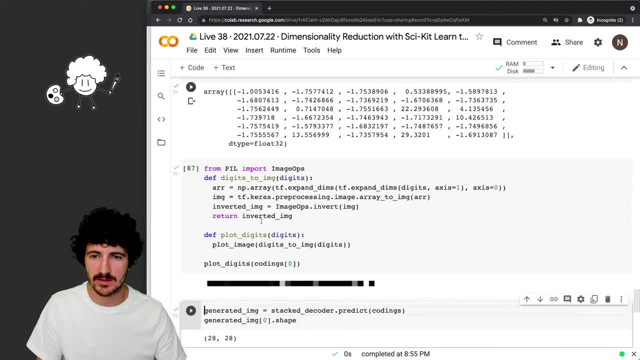 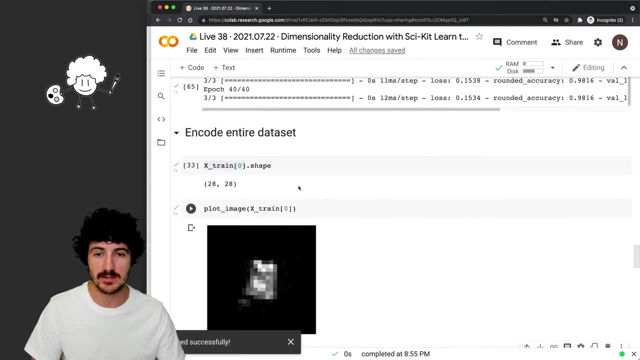 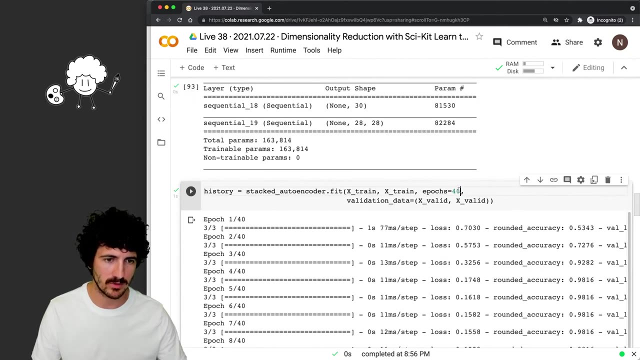 From zero to one and they're 30 and depending on when you load them, So like at what point or after what training they, they change. All right, We define the model, We do this definition here, We train summary, and then we're going to train for 10 epochs. 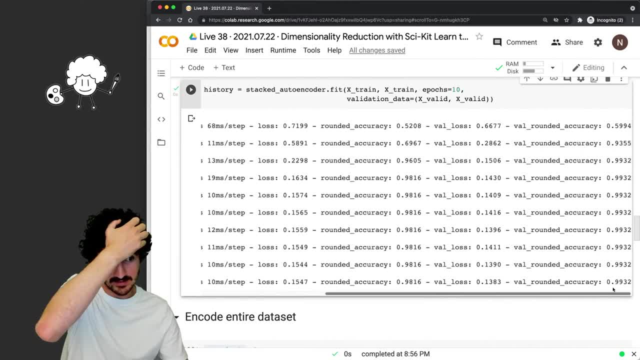 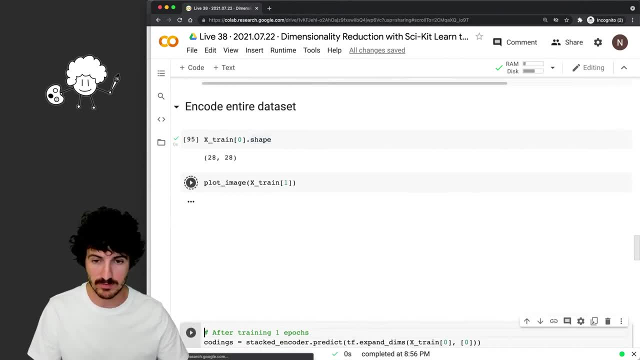 So still, the model always gets to the same place right, 99,, 32 accuracy and that's 10 epochs. So we still have the same input. We could Maybe take this one or this one right. These are different sketches. 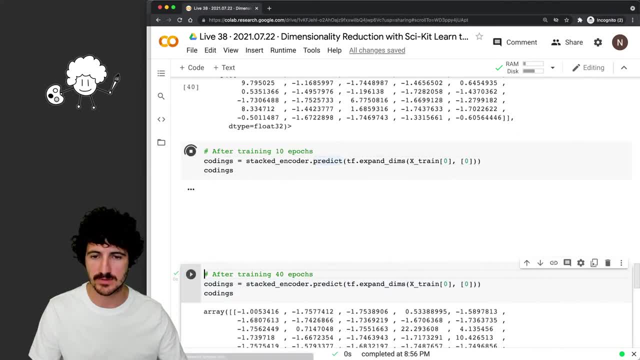 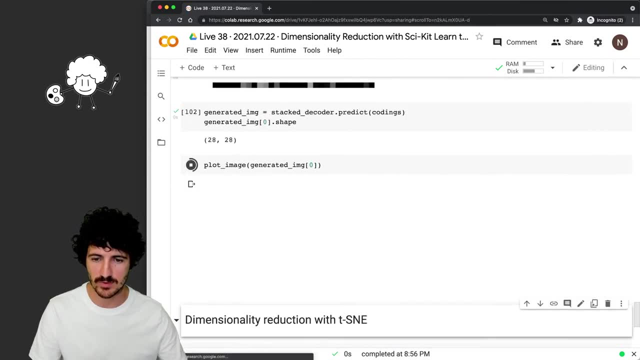 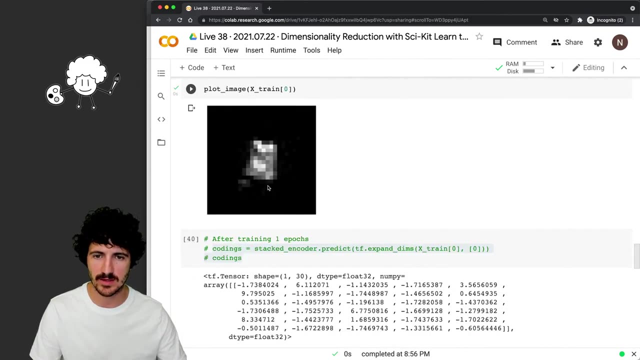 And that we pass that through, this one that says it wasn't 10 epochs, And now we can plot our digits. It's slightly different than before: we generate an image and now we predict. So this is a slightly different than before And we could actually just comment this out and we're going to take another image. 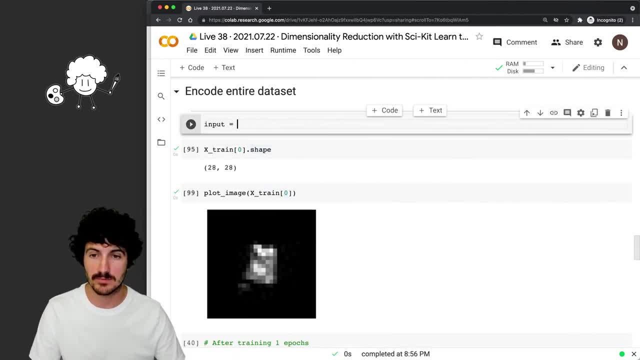 So let's say you met image 80. So let's say input is going to be X, train 40. So now we just do this, So you just get the input, You don't need to do a lot more input. And now we can choose from here with a number. 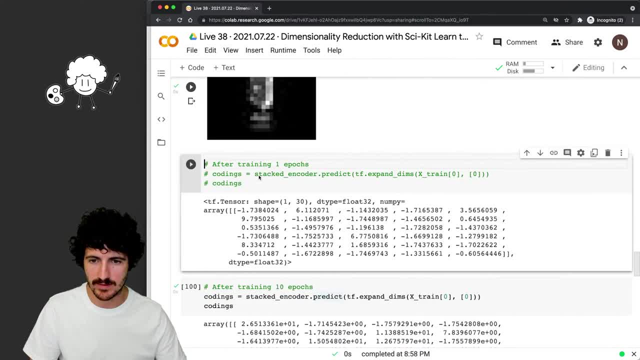 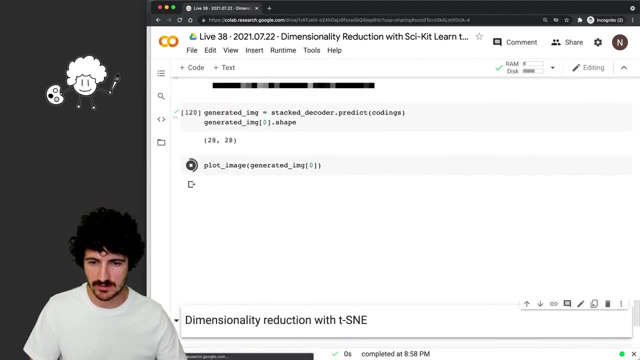 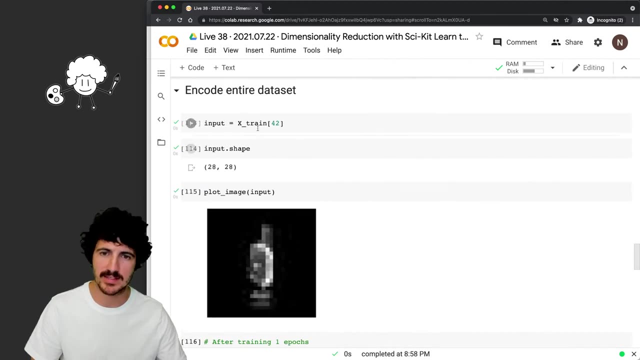 So we say the input is a sketch 42. We have that and this doesn't do anything. is any something? Now we plot our digits and now we reconstruct our image, which doesn't look anything like this at all. So I don't really understand what's going on with, with the data set. 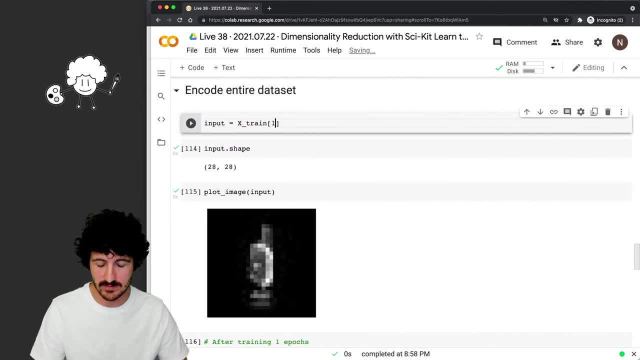 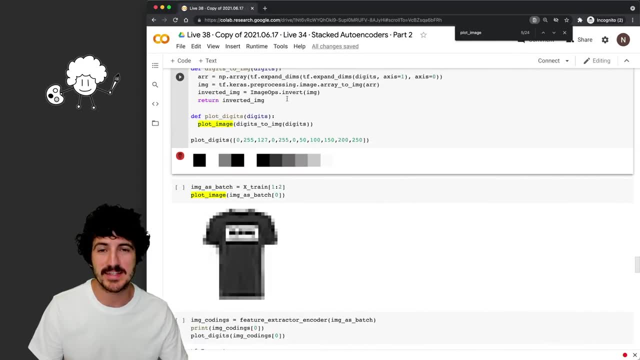 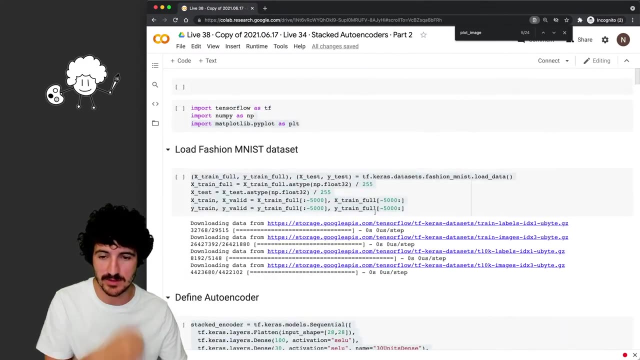 It might be. It might be that it's over Fitting, And it's just like learning something that it does something really similar for everything. for all the images, The, the fashion companies data set has 60,000.. So that's probably one of the things why E is performing so much better. 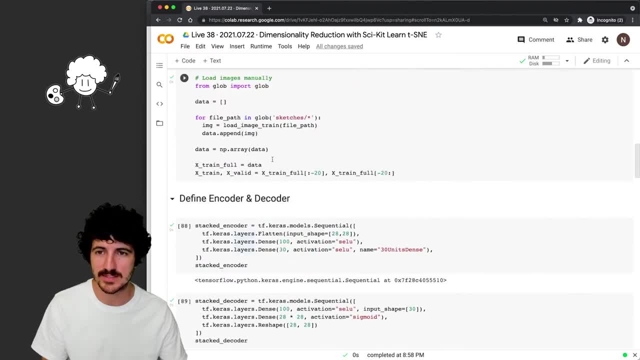 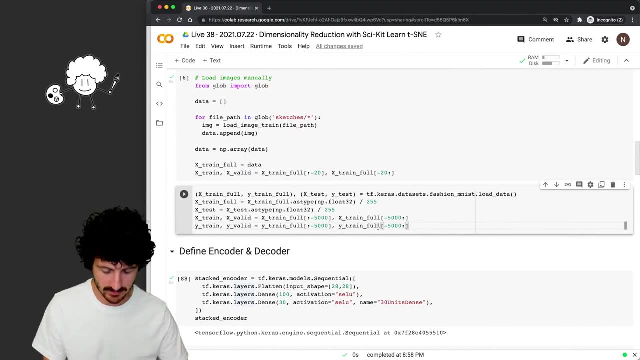 Right. So now we're going, after all this effort, to load our custom data set. we're going to define here their data set. So then we're going to have the same X train, X valid the set. I don't think we need this part. 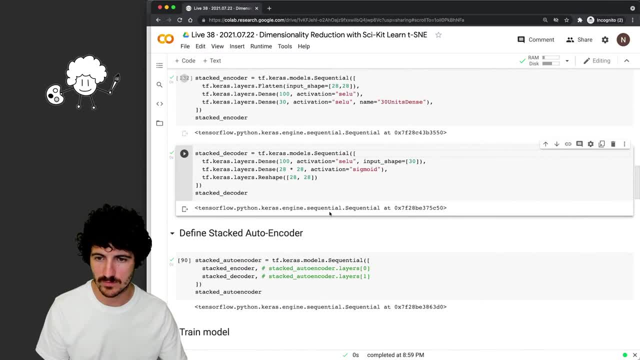 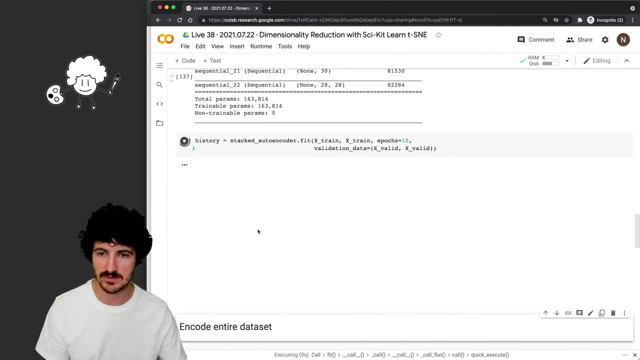 We do need this one. So we're going to load that, We're going To load our model, We're going to define everything the same way and we're going to train for tenant books. Let's see how long this takes. 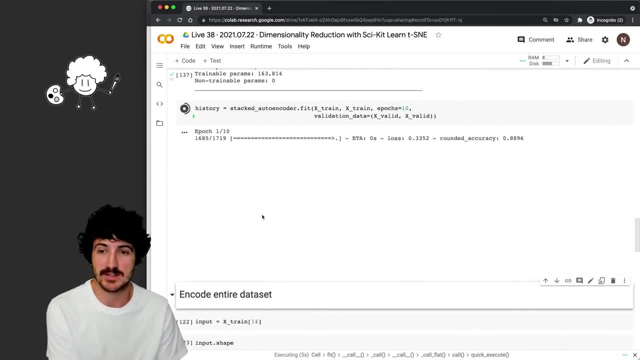 This takes a bit longer now because we have a bunch more images. We have 55,000 images for for training and 5,000 for validation And, uh, you should be uh thinking right now. the accuracy is slowly going up. 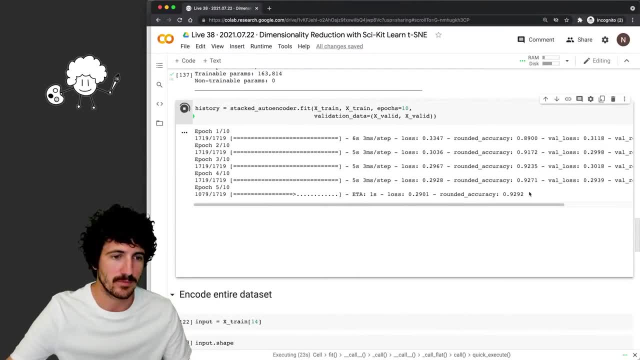 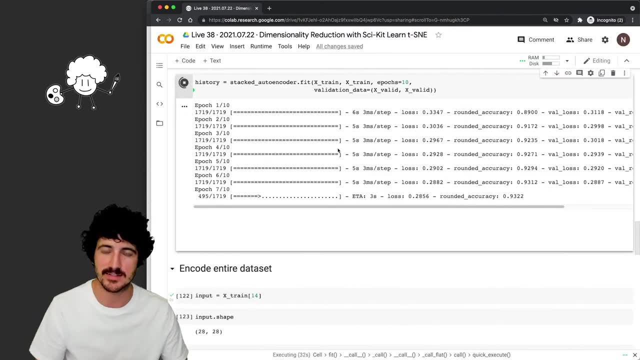 It's not as fast as it was going up before. So we can see here: this number keeps changing, And that's good right. This means that there is some actual learning that is happening, Not just that we're overfitting on a data set and learning a few things. 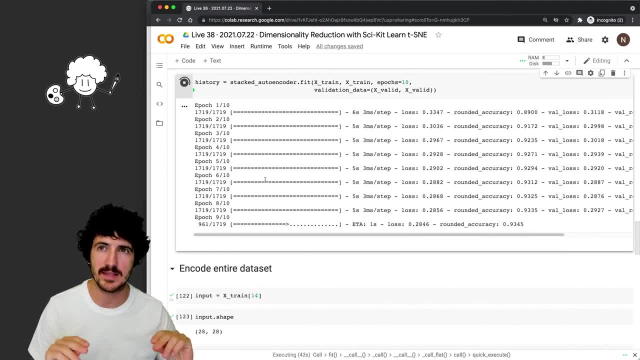 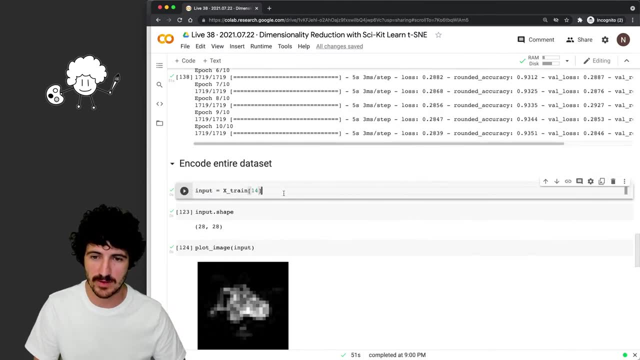 I would be interested in seeing this network how many data points it needs to give any like some information that makes sense. All right, So the model is trained. Now we can put input 14 here. That is this. that looks like a shoe. 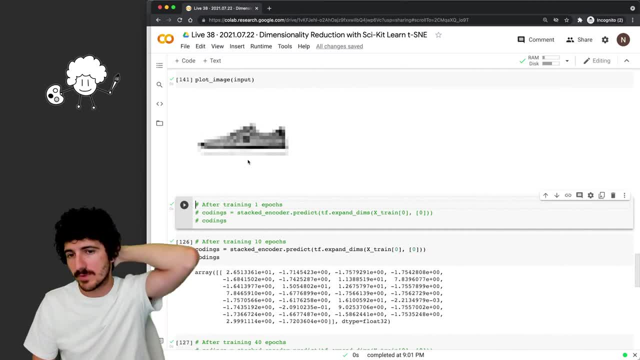 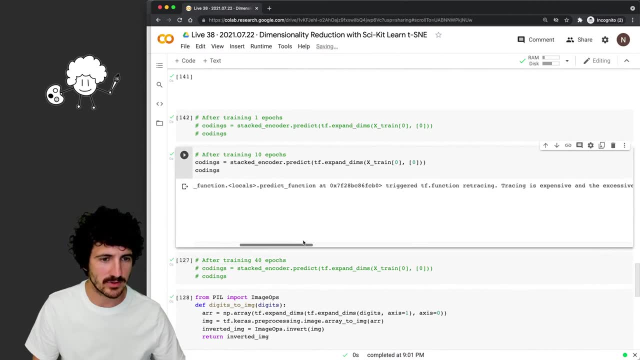 I also looked that the data set is inverted, So that also might make it learn in a different way. So We get the coatings. We still get Oh, five out of the last 10 calls triggered to your function. Retracing is expensive repeatedly. 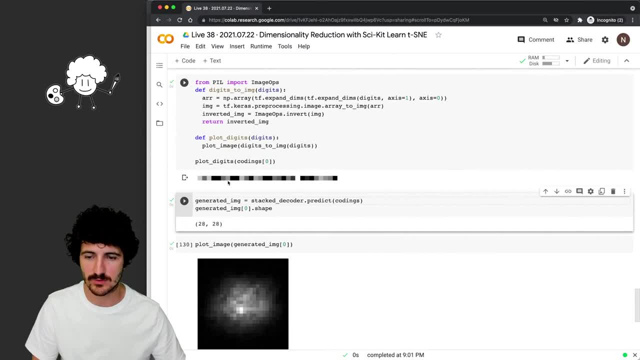 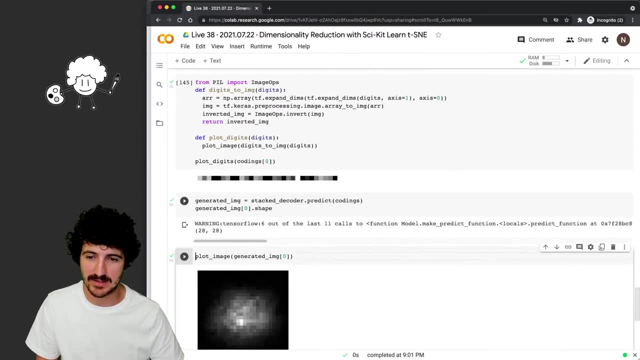 All right, But we get our data and now we get our coatings. These coatings may a lot more sense. It's it's a bit more granular, It's not just like a lot of black, and we get our generated image here. 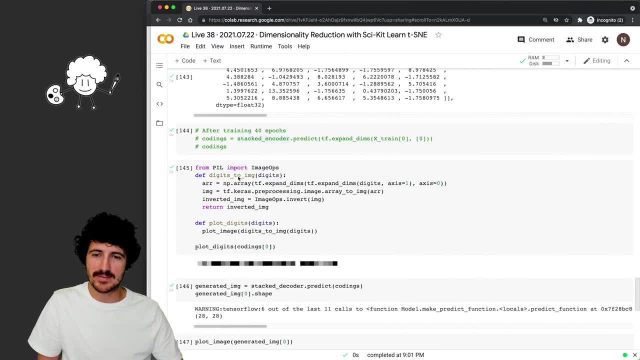 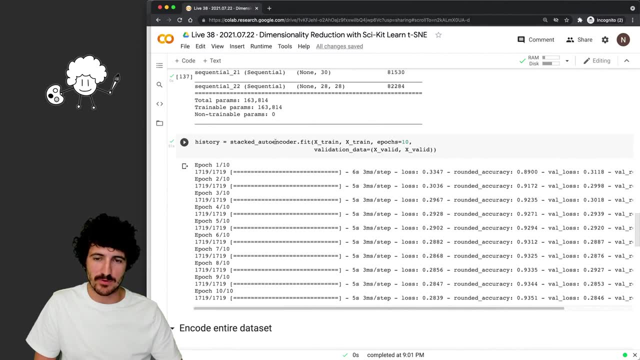 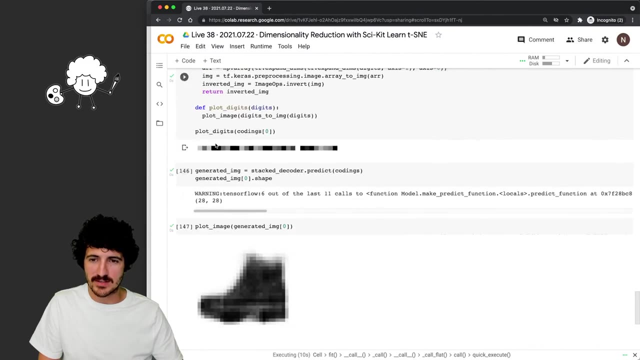 All right. So it doesn't look anything like it, but at least it's a shoe. So it's learned something And it seems like We're able to reconstruct the output from what we have. Let's actually just train for 10 more epochs and and see where we get just to, to let you know while that's training, coatings here actually represent the issue. 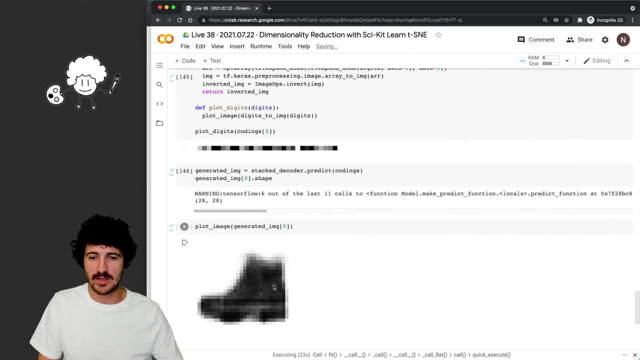 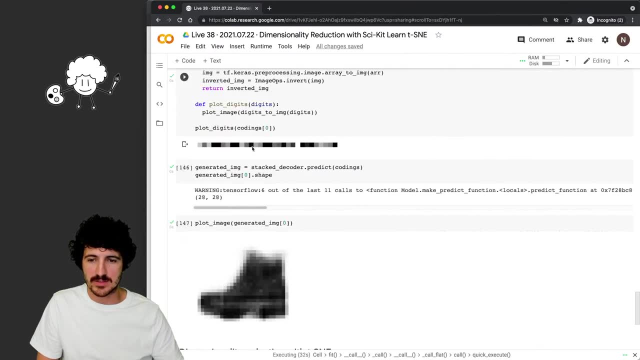 If we modify these coding, we're going to get a different image. That's like a puppeteer, Like we. we have an image, we're encoding it into this image and then we decode it back. So if we generate images like this one, we will get images like this: 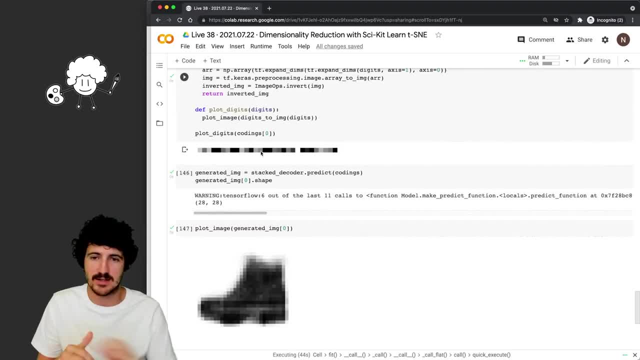 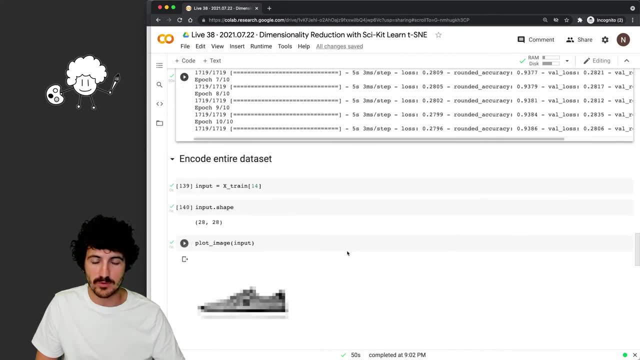 There is a correlation, of course, because of the weights that the neural network has learned from the coatings to the output. It seems like we're almost done. We have a bit more accuracy- not too much more- and we are going to use the same input. 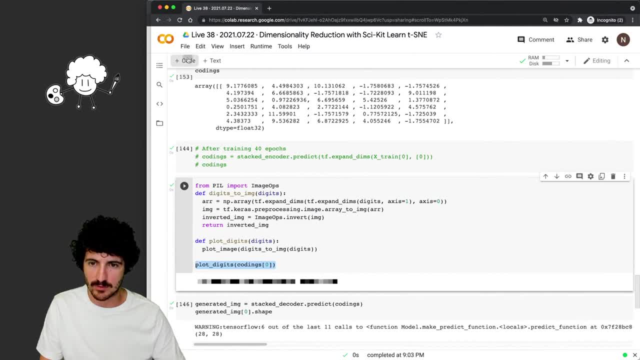 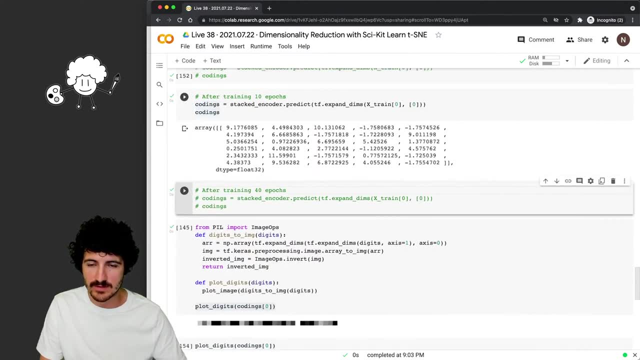 I'm going to do one thing: I'm going to leave this here and I'm going to compare. So how the coatings are different. They are almost the same. So I say, let's regenerate this, as in case, generate the coatings. They seem to be almost. 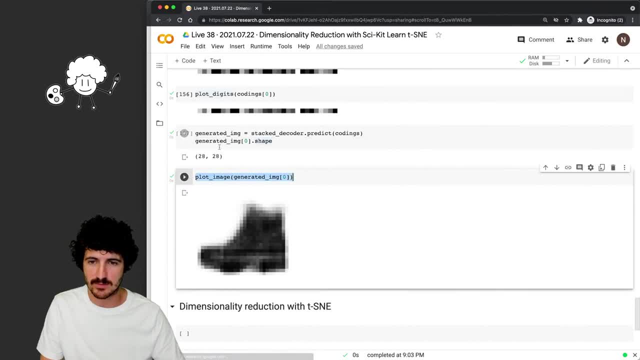 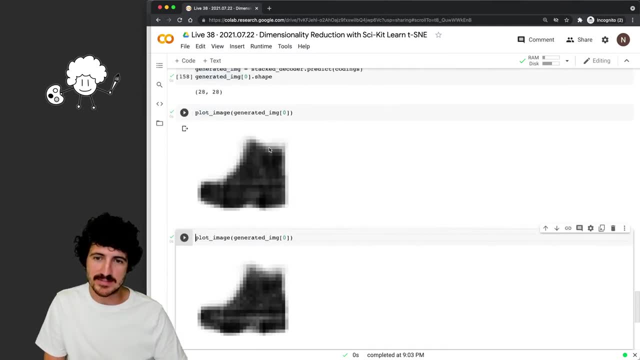 The same. Let's see if the decoder has learned anything else. So we have the image, here We're going to predict and now? so I'm going to put it here, So I'm going to regenerate a new image and I can already see some changes in there. 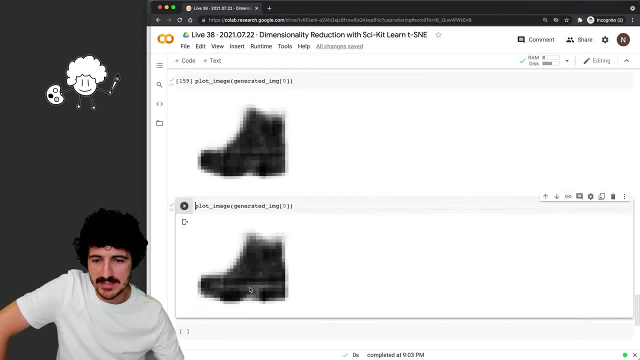 I'm going to say I made an error. I made a mistake. This has changed right, So we can compare these two images and they're different. So there is something else that the network is learning while we're retraining. What is funny is that I forgot to change these variable here. 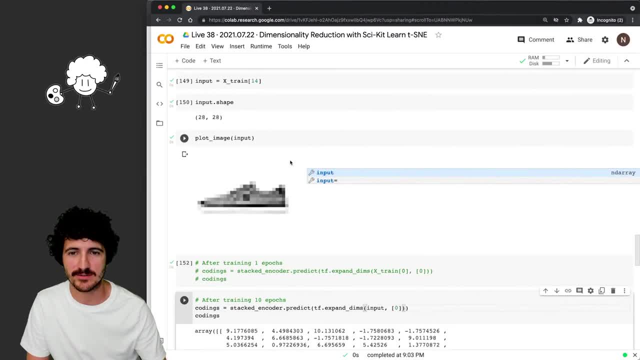 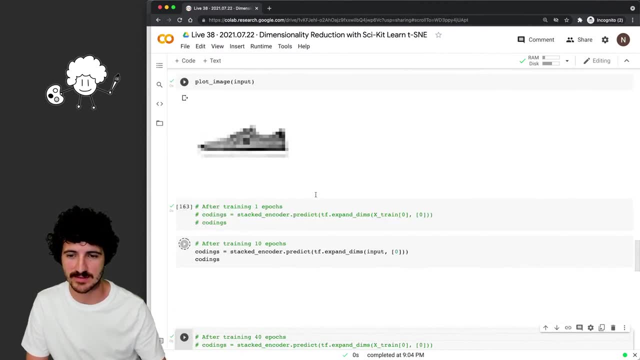 So these should actually say Input, because we were continuously using extra in zero while we were visualizing here the number 14.. So if I actually do this right now, you're going to see how the coatings that we get are going to be super different. 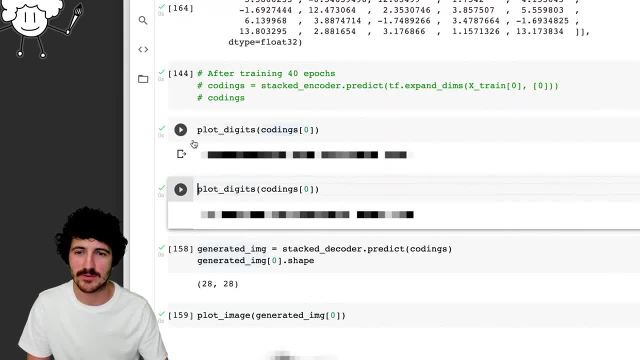 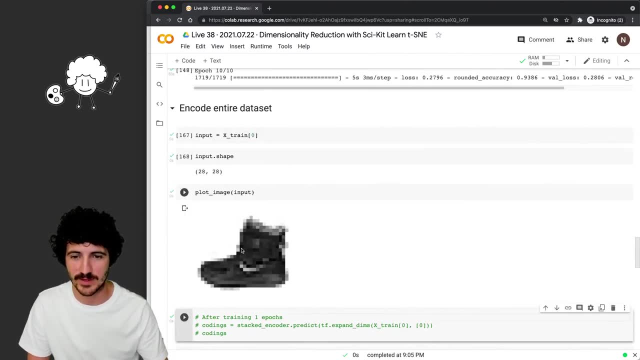 So look at the coatings. So these coatings here are super different, right? These now do encode the shoe We can see is that we go to zero and we plot that image. We indeed have something super similar to that boot that we were generating before. 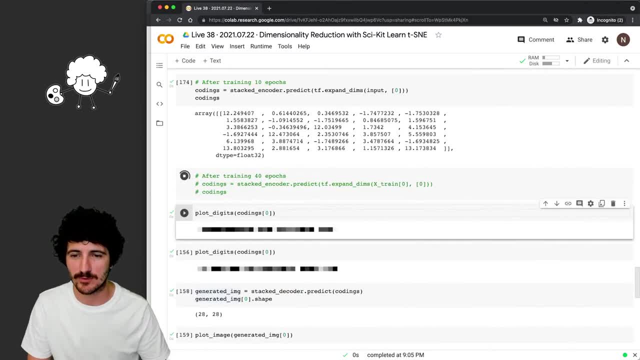 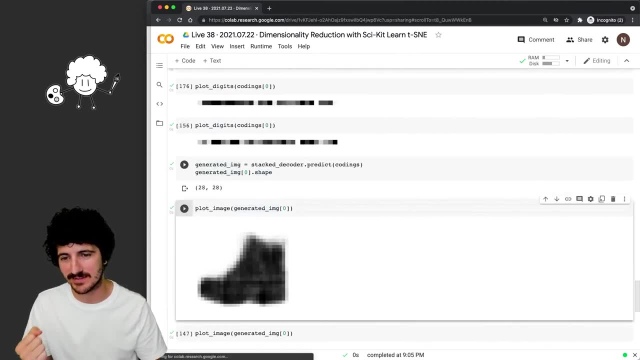 Which is super funny. So we're going to go back to the shoe, I'm going to go back and generate the coatings And now I'm going to generate that shoe and I need to predict before. So predict and generate that shoe- Awesome. 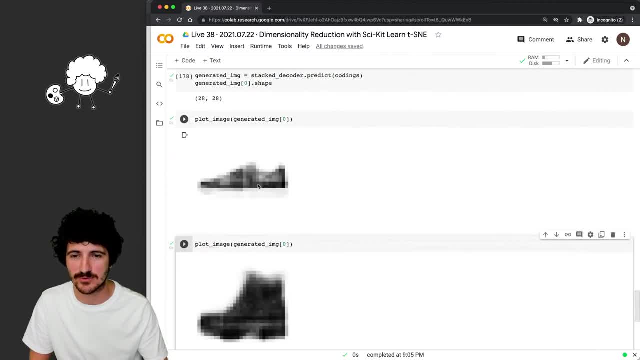 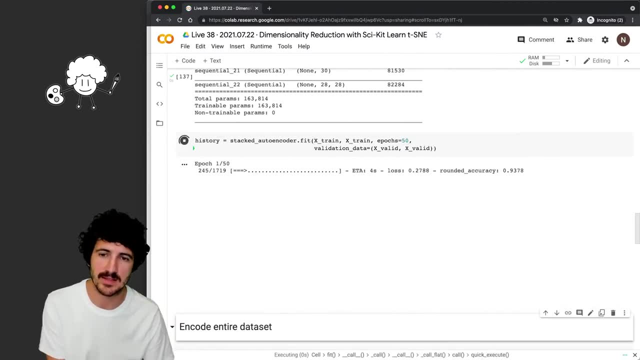 So now our decoder knows how to generate a shoe. So what this brings us, or where this brings us, it's actually trained for 50 more epochs, something that is going to take a bit, And let's try to take the rounded accuracy up. 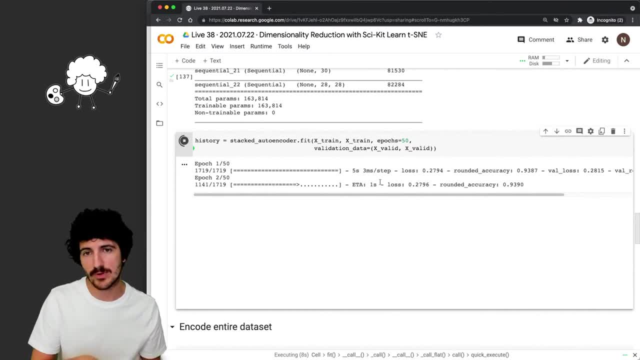 Let's see how the network learns differently, And later we're going to go back. Okay, We're going to use the data set of the sketches and actually verify if there is something that is being learned, because before, even though we were training, we were not changing the actual input that we were predicting with on the encoder. 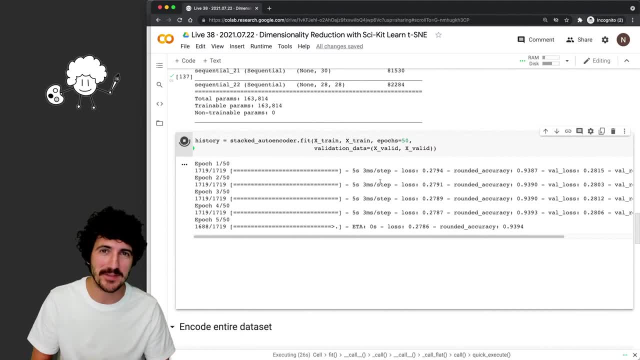 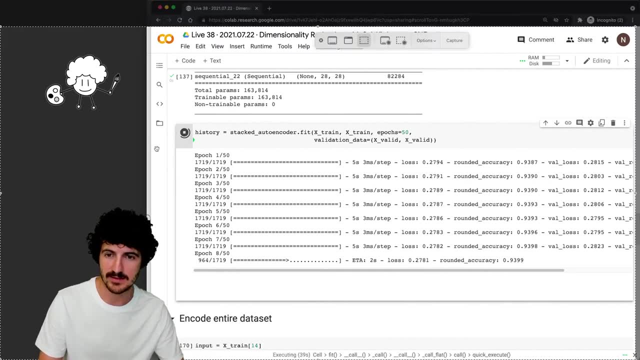 The coatings were not really changing, So I do still have hope that we are going to see some, some things there and that this is going to improve a bit. All right, Maybe I can. Yeah, no, I'm not going to do that. 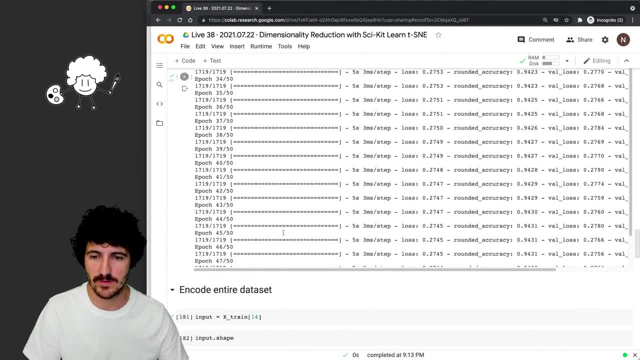 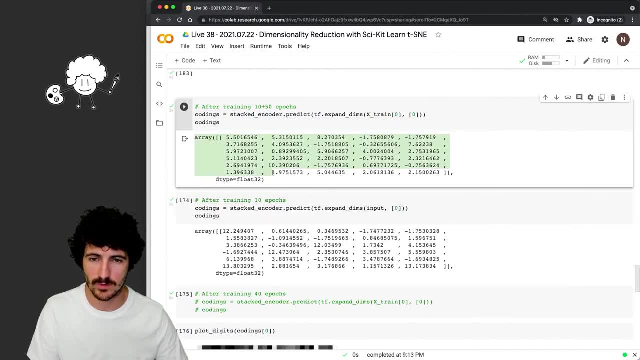 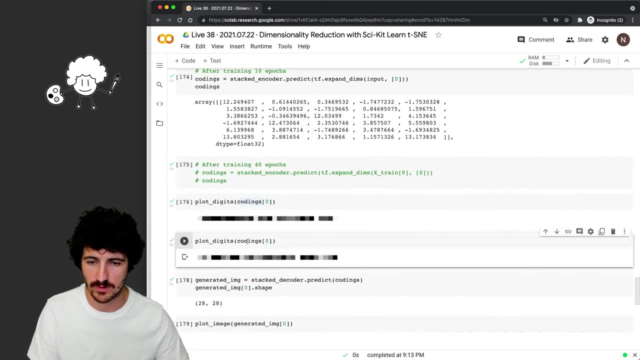 All right, Okay, We've trained for, I believe, 50 more epochs, right, I think? I don't know, it might be 10. Plus 50. So we can see those here. So the coatings do change a bit, and now when we plot them. so these were the ones from before. 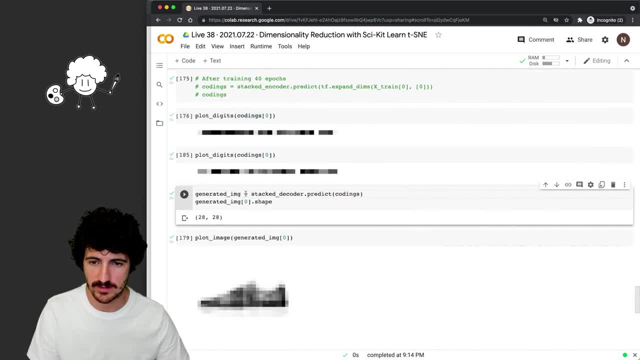 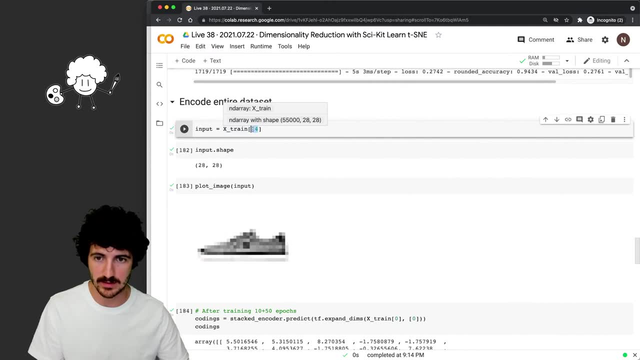 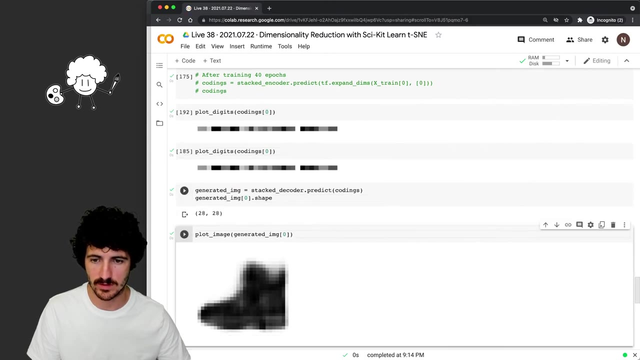 So when we plot them, they're really different, and let's see what the generated image looks like now. So we put a block in here. We need to define this year 14.. We put this here, We plot our coatings, We is. 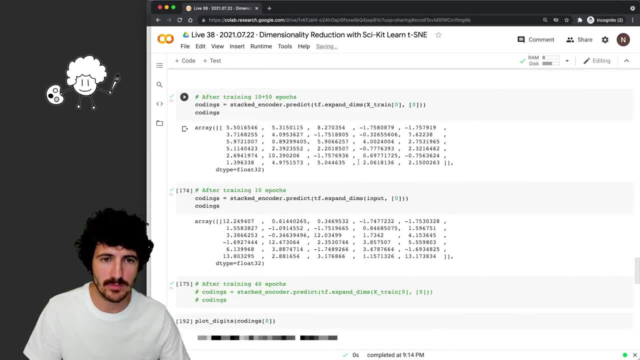 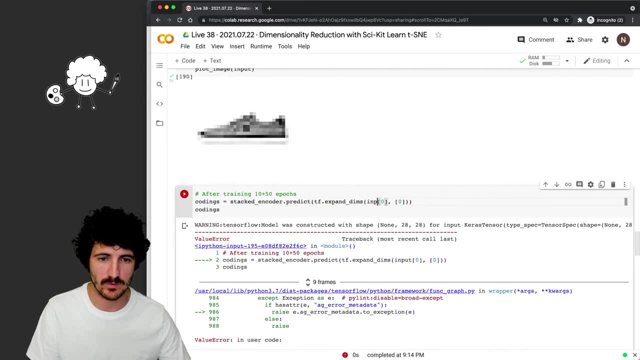 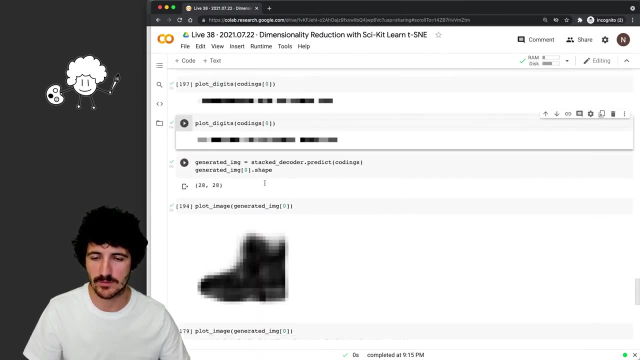 Huh, What am I doing wrong now? Input: Oh okay, So same error as before. So we left these on the old code. So that's why we were erroring here. So we get the coatings. Did these look a bit more like the ones below these look back again differently. 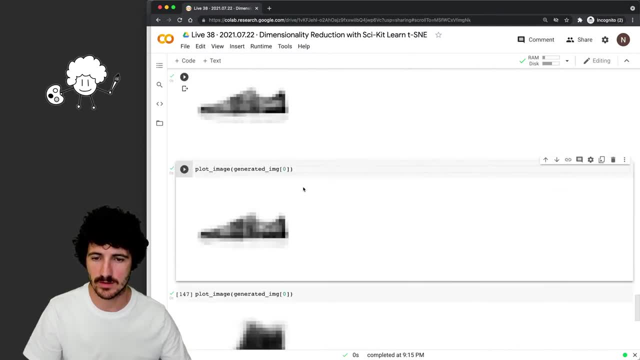 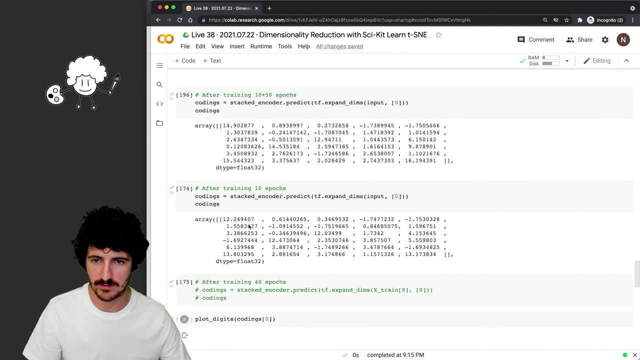 And now we predict and now we plot. Okay, So we're getting you know. you see here stripe, and I would say it's hard to notice Which one looks more similar. This is a bit more refined because we've trained for longer. 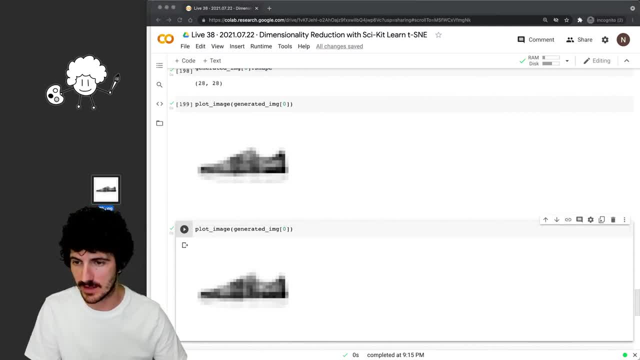 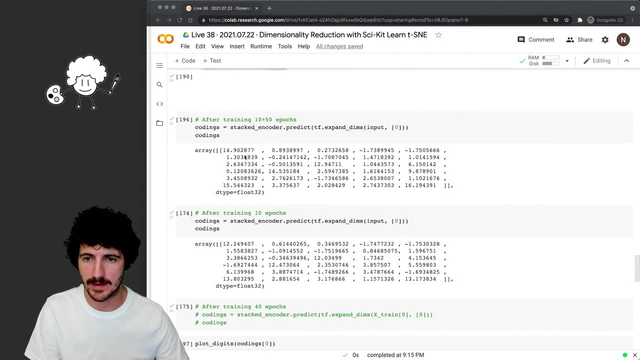 So I would say, maybe this one, So this is like a 10, this is a 10 plus 50.. Let me show you here, And this is the input, is the original, So this is the actual input, So which one looks more similar? 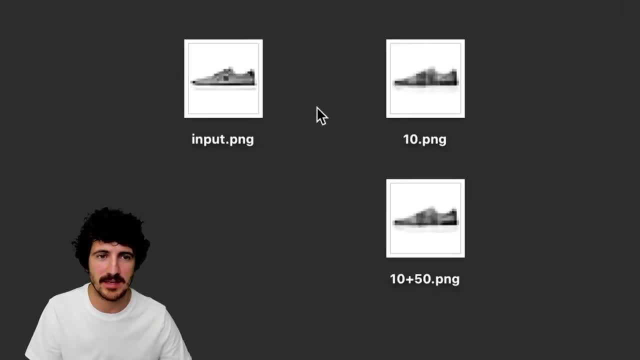 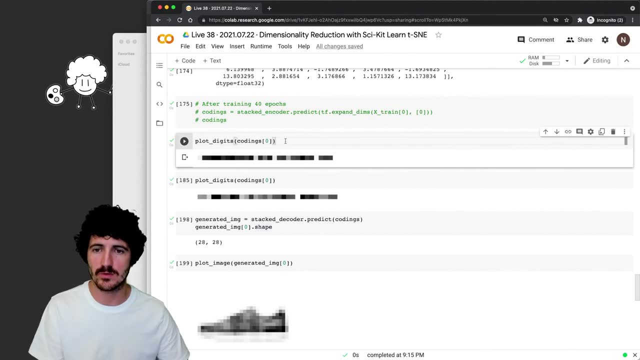 Not sure. They're more or less the same. So what I was mentioning before. so we try. what I said Is that These coatings right. If we look at the coatings what they really are, they're not more than an array contained inside of an array. 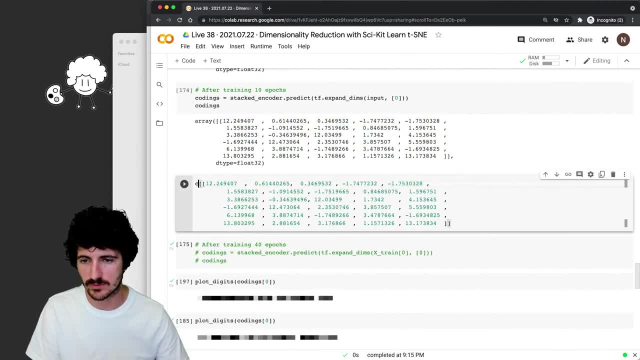 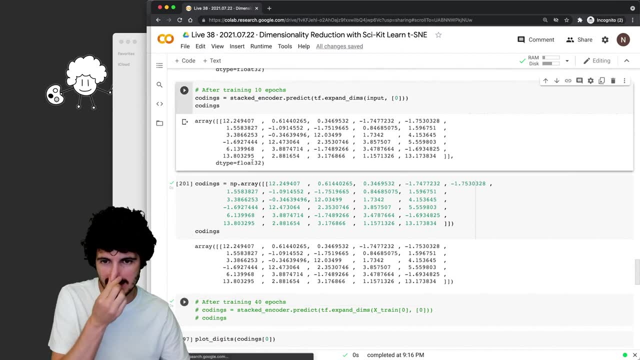 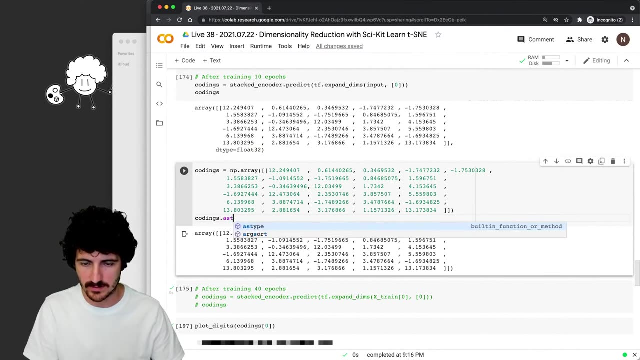 So we could get this here and we could say: my coatings could be an MP array with these data And now we put in the coatings and now we get exactly the same. but this is float 32 type And we could probably do that as type. 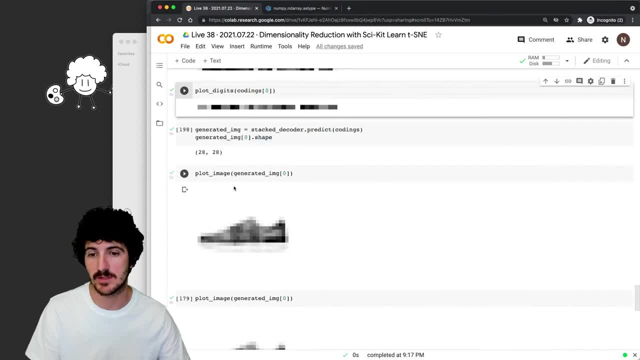 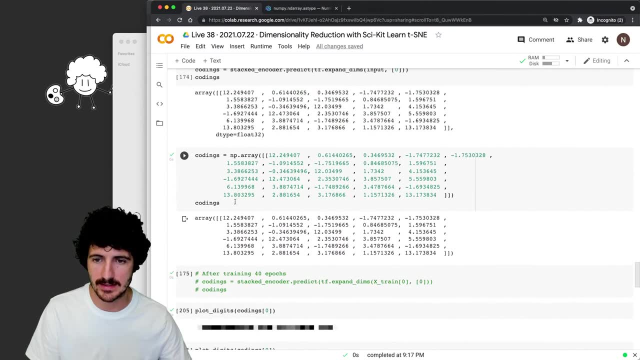 So I get the coatings. this way I plot them. They're the same because I just copied And then we predict we get the image right. Let's put that image below. So those are the same image and I'm going to bring these. we'll leave them here. 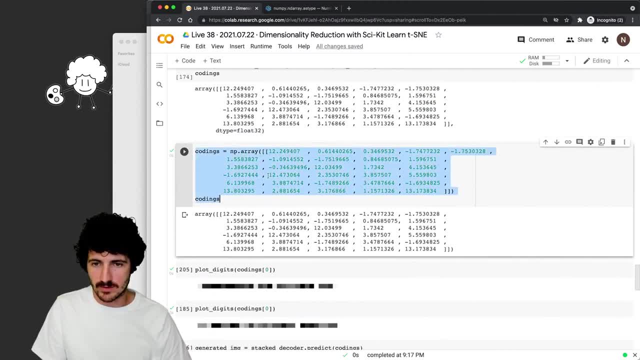 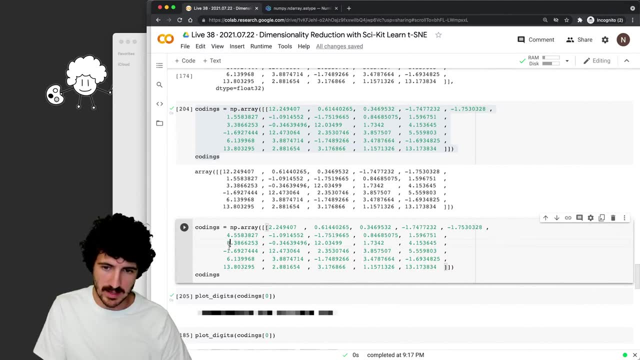 So now what I'm going to do is I have these coatings here and I'm going to copy them. So I'm going to change them, them a lot. So maybe we put here: a four is going to be an, eight is going to be minus four is going to be 13 is going to be one, right? 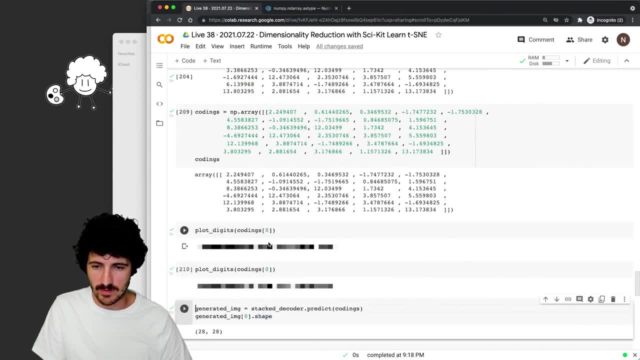 So we changed those coatings. and now, instead of the one we have above, we have. So we change those coatings And now, instead of the one we have above, we have, Okay. And now, instead of the one we have above, we have the one below. 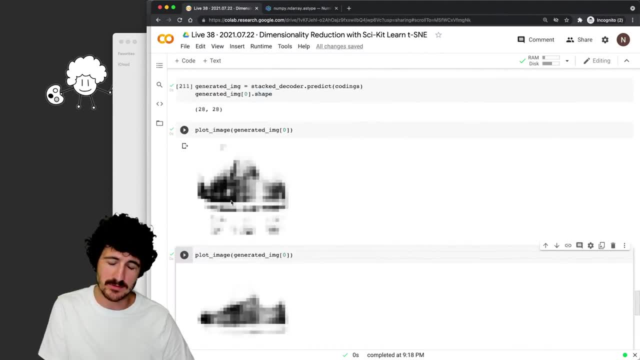 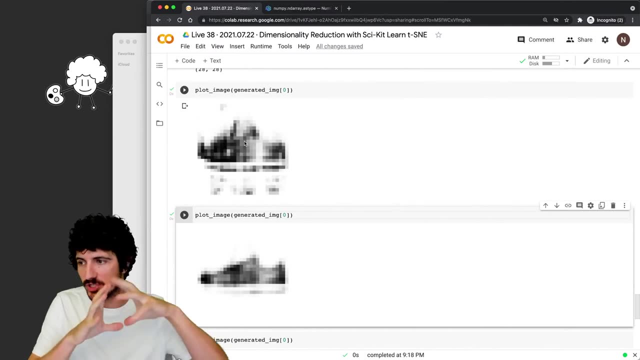 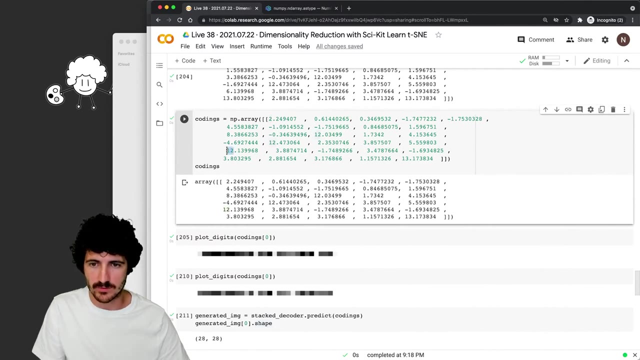 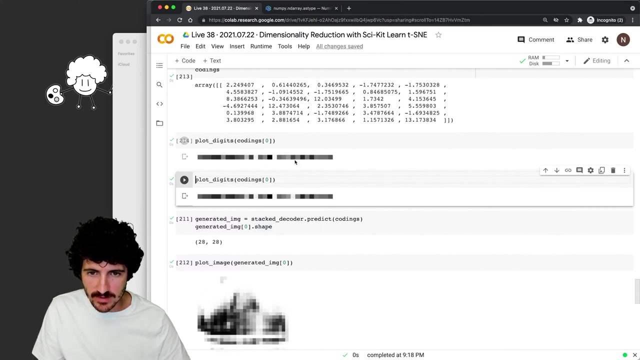 And when I generate the image, that is what happens. We've changed the things and there are some parts of the image that I still look the same, but by changing numbers we're changing different features on this image And one can imagine that now, if I do put this one here to zero and I plot again now, we have just changed slightly something here, right? 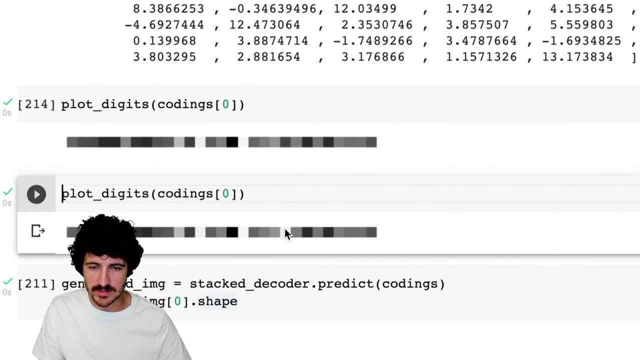 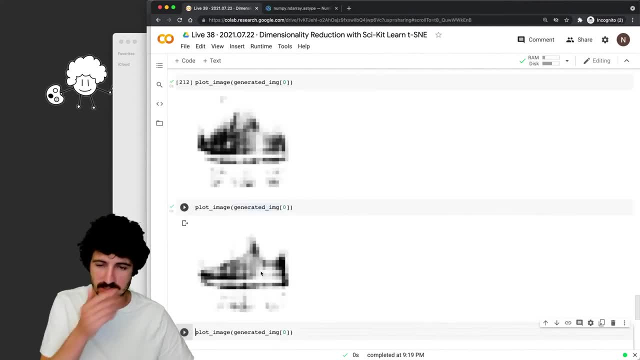 So instead of white, we get this gray, Instead of this gray, we get this white. And now I can predict again and generate the image And now that changes back again and looks again more like a shoe. just changing one number like changes the app a lot. 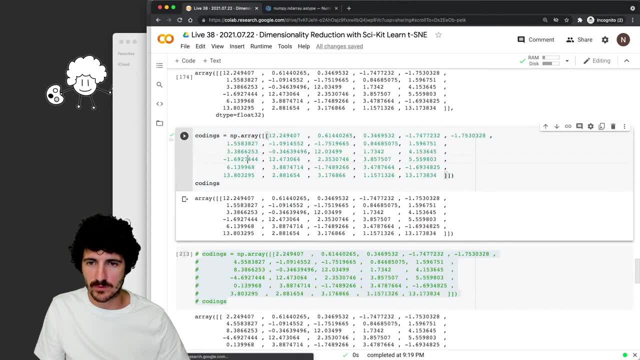 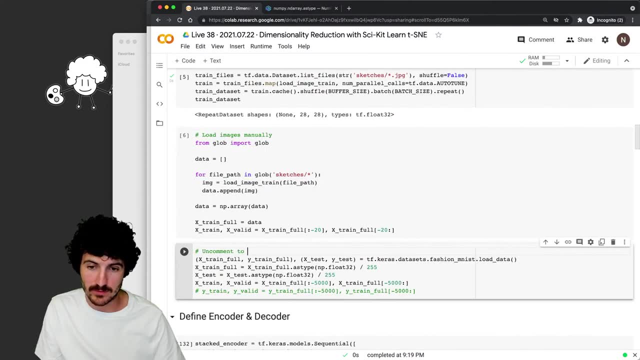 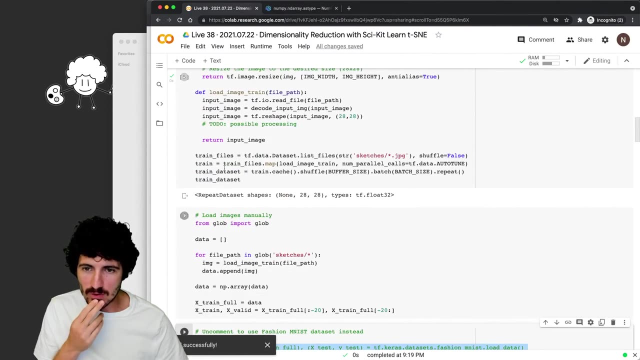 So what? we're going to make sure that we don't get confused later and we just use the actual prediction function and we're going to go back and comment to use fashion MNIST data set instead. right, So we comment this out. And now what? we just want to go back to where we are. I think everything right. 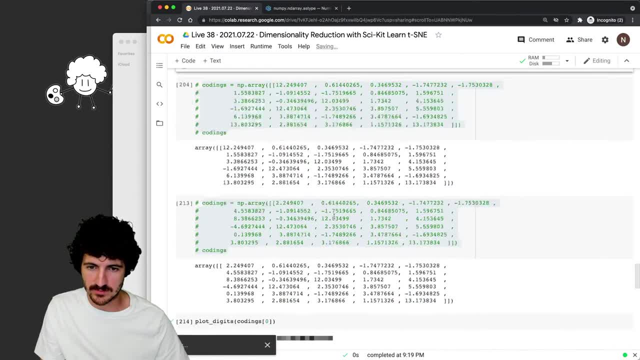 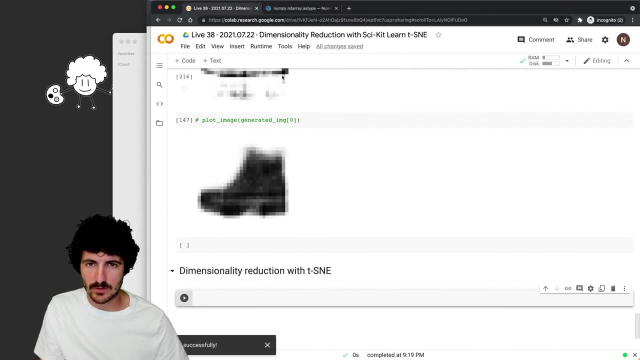 So we don't really need to expand twice here and we don't really need two codings and we don't really need three visualizations. So what we're going to do is that we're going to go back here, We're going to run, restart and run all. 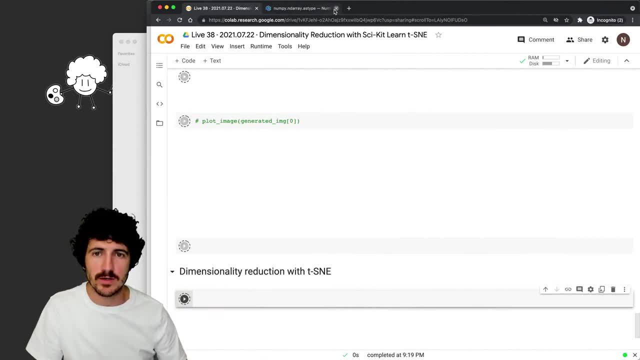 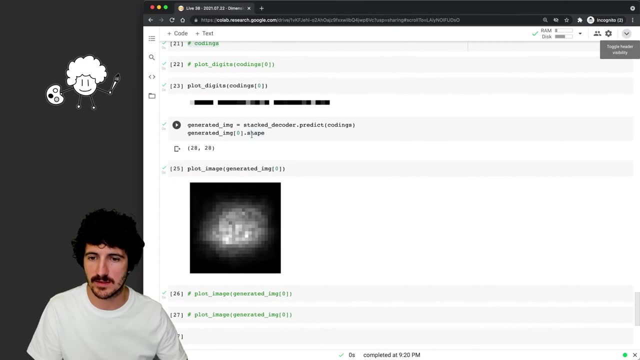 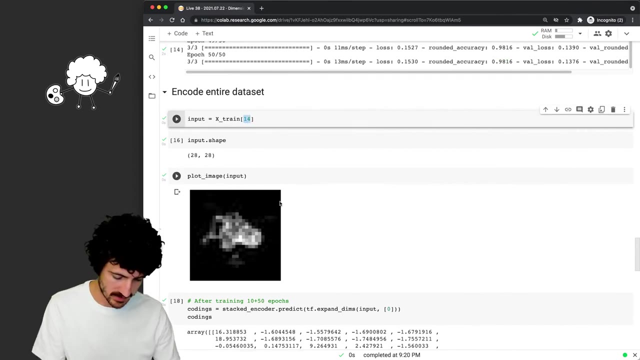 So this is going to restart the runtime of our Jupiter notebook in Coda and it's going to execute all of our cells once again And, yeah, Hopefully we can see something with our data set. So these are strained. We're at the same accuracy that we were able to get before, but now we have an image that, if I said here 60, we can see a different input. 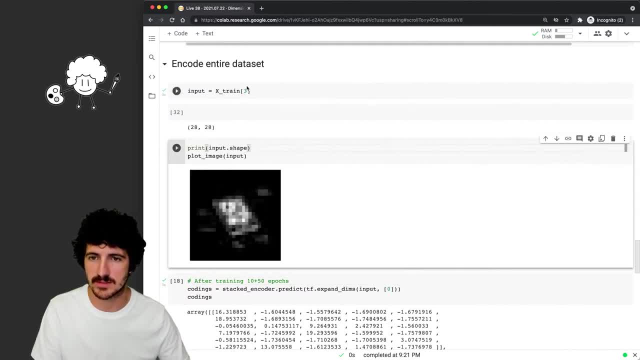 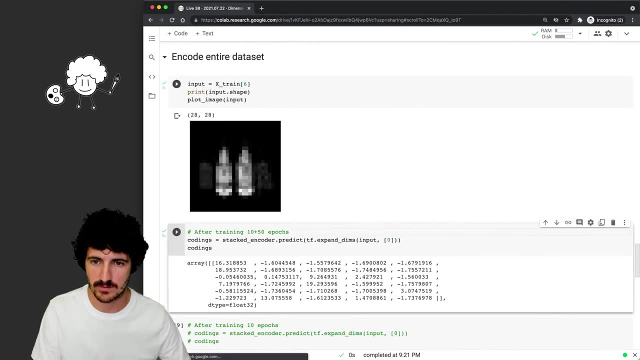 So maybe we can just merge these ones, because it doesn't. we don't really care that these are just one cell, So we're going to remove these other two, So let's see six. Okay, So this is different, right From everything else. 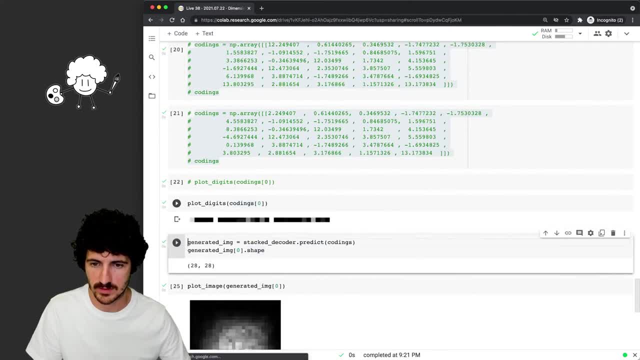 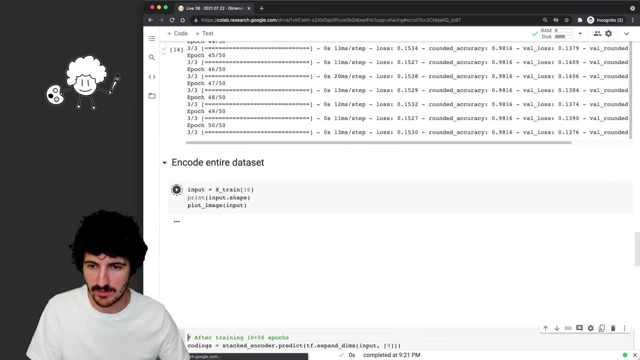 So we're going to go and We're going to Run the codings, which are a bit different. This doesn't seem like it's changing a lot. So we go now with 16, we have the input. we're actually predicting on the input. 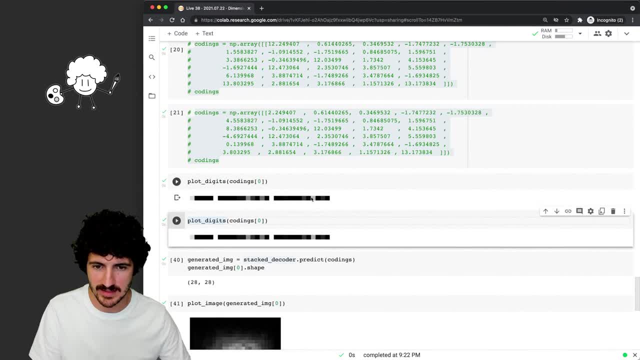 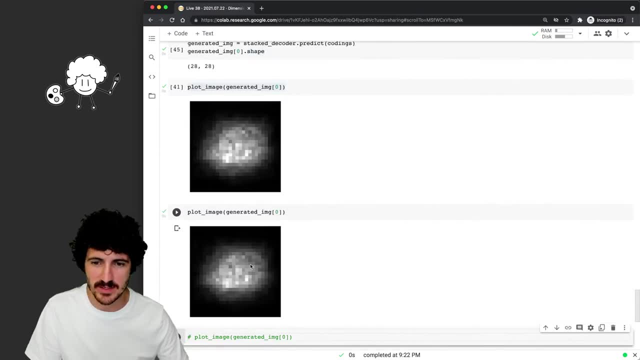 We plot the digits here, So we're going to plot the digits again and they barely change. So we do this and we do this. Yeah, So this is changing, but it's barely changing. It's just learning like a real weird mapping. 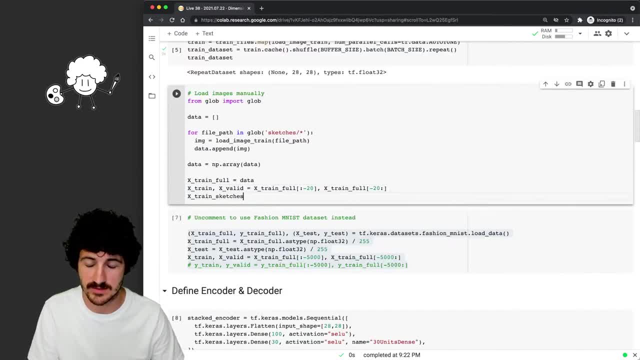 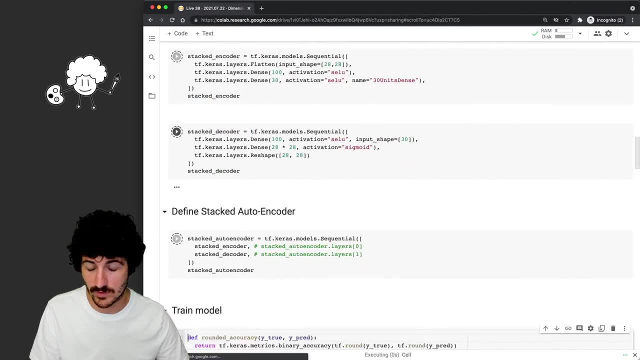 Let's do here: Save this as X train sketches, X value sketches equals X train, X value. All right, So we're going to rerun everything, So we're going to retrain now and regenerate the images. So it seems fairly simple. 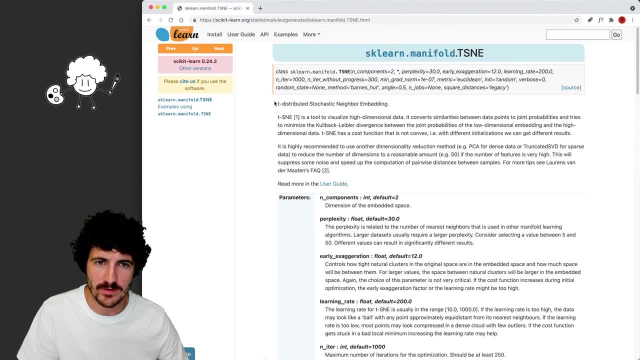 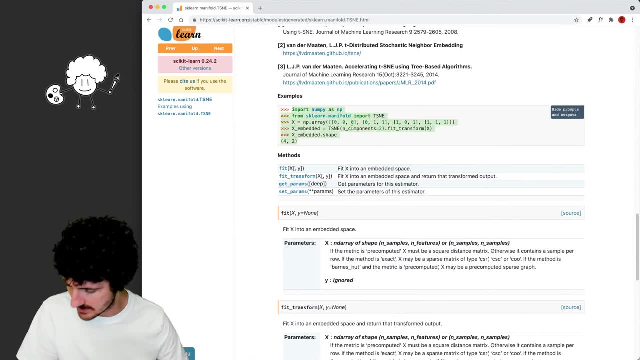 So we have need the scikit-learn implementation, which is including a scaler manifold Disney, And all we need to do is something like this, more or less. We're going to do that coding before we go today, And let's see how this went. 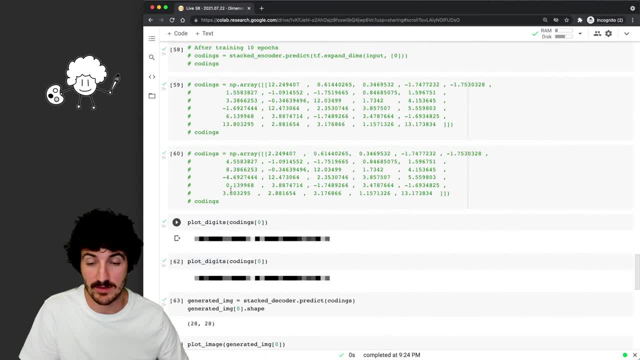 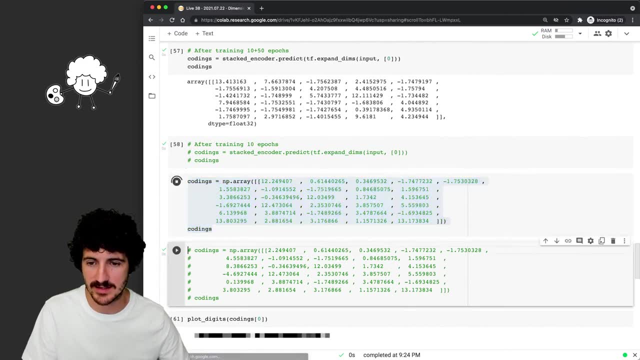 So we have this And we get pants, which is pretty good that we have a lot of data involved in in this Experiment. right, We could get these again like hand generated coatings which match this one's here Pretty similar. 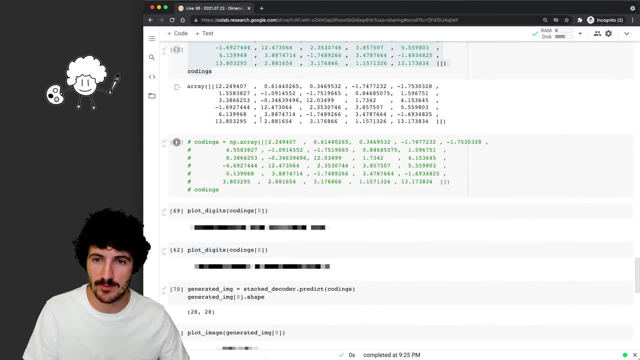 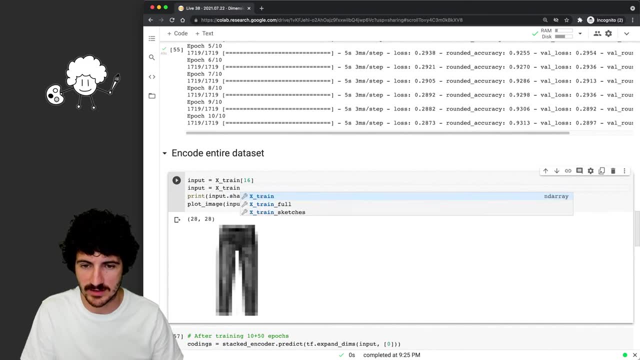 And we get this, which is a completely different output. Again, let's comment that out. And instead of getting an input X train, so we're going to get an input X train sketches and we're going to get the fifth sketch. 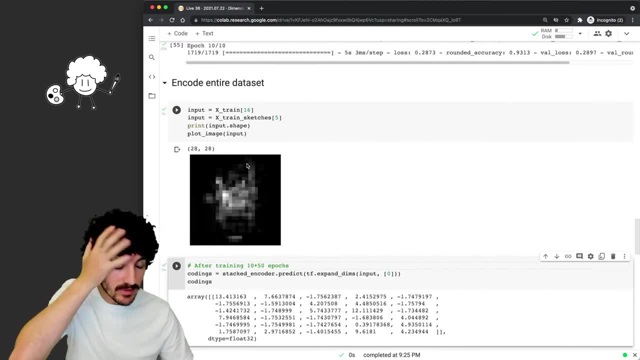 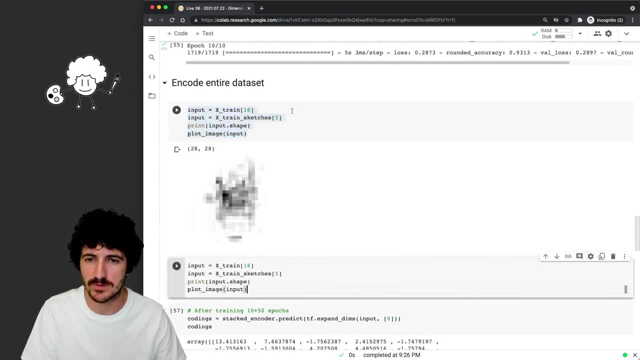 So now we're talking about This one And, uh, one thing that I mentioned before is that the inversion of those, So let's actually put this separate. So we put all their logic here. current data set or force. custom loaded data set. 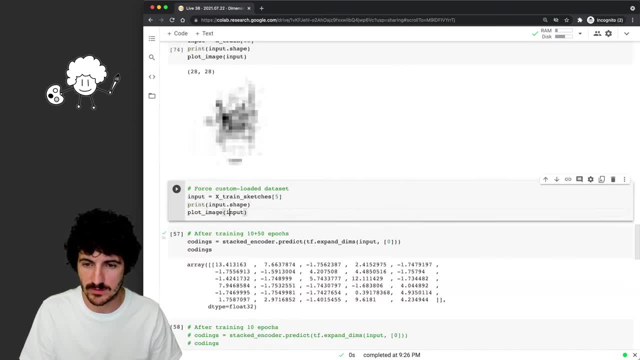 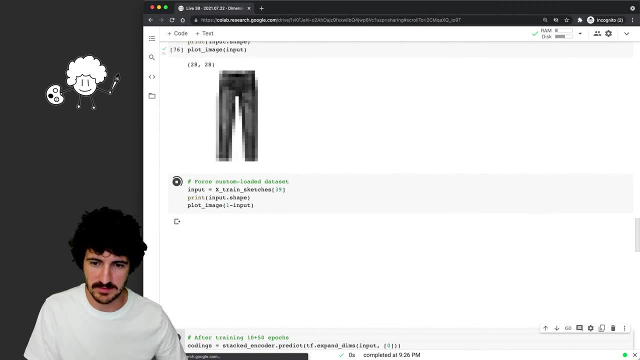 All right, So we are going to load that and we're going to plot. So the input minus one, these would load the original image and this one would load like a separate sketch. The interesting part here is that we have images that correspond to to my drawing. 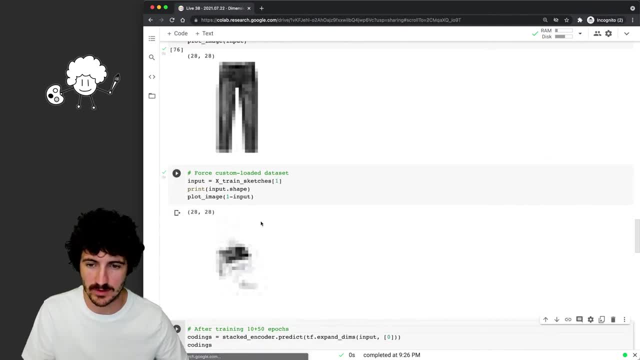 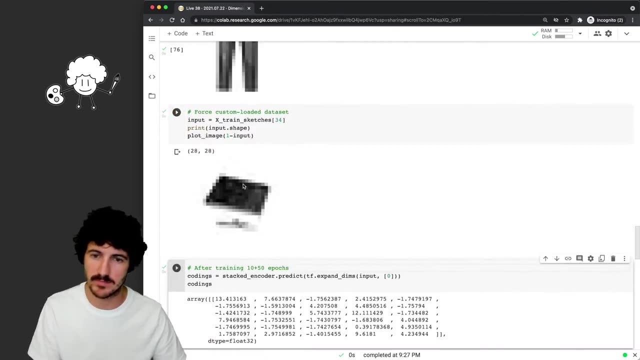 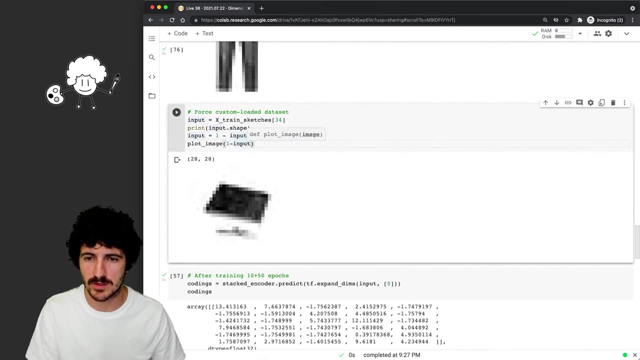 And not to clothing. We want to see if we obtain the coatings of one of my sketches. what is the the corresponding image from the decoder that we're going to obtain? All right, This one, for example. So I think what we need to do is say: here, input equals one, minus input to get it negative. 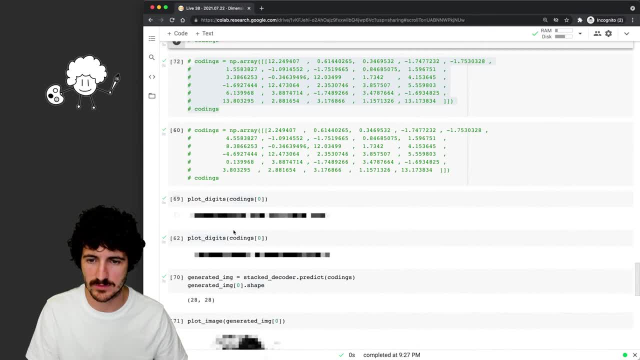 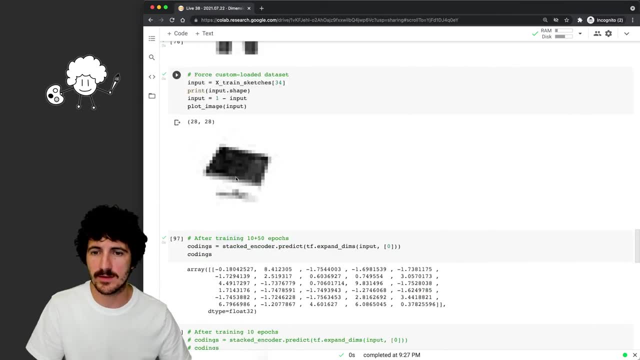 So we don't have to do this here and now. we can do this. We can extract the coatings once again and we generate the image and then we plot it All right, So You can see Right Like it's activating that part here. 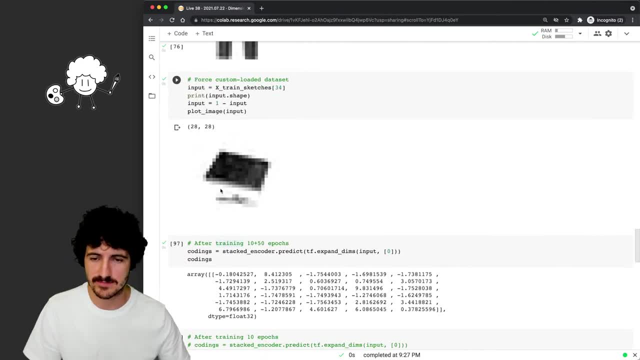 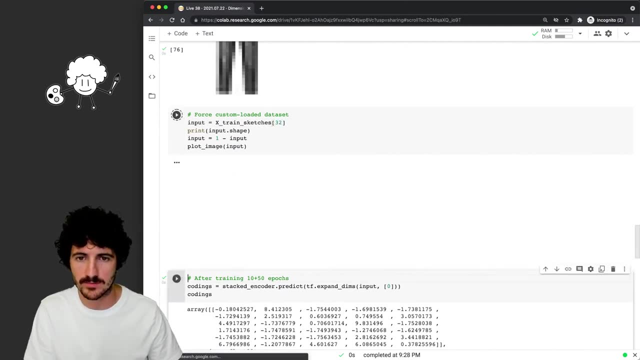 So he's trying to make it into a shirt and, um, it's a good experiment. It's kind of activating or encoding with one data set and then obtaining with another one. Good thing is, if we just comment this out, we still have the proper data that we needed. 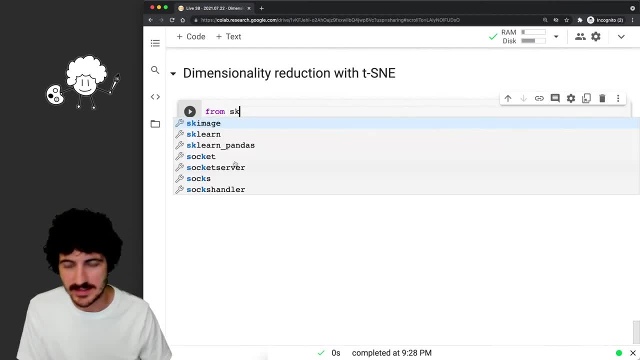 We just need to say okay, from It's gay, Learn, manifold What we saw before. import Disney, Right. So we import that library, Okay. And now we say it's valid because otherwise we're going to have too many. 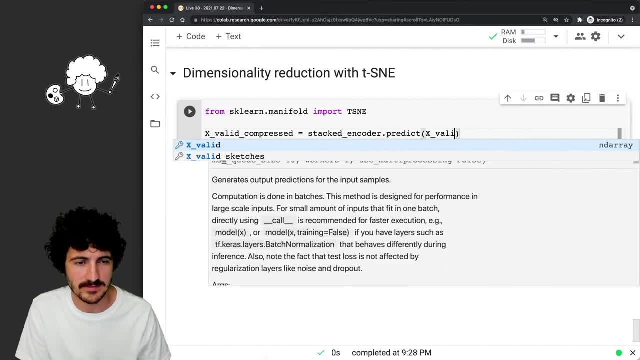 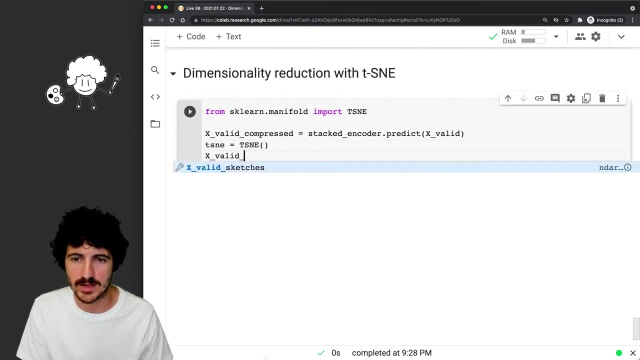 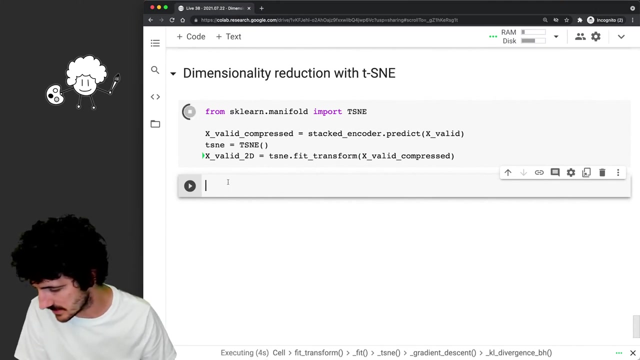 We say stacked encoder, predict X valid and we do Disney equals Disney. So we instantiate this library and then we do X Valley to D equals Disney fit. transform X valid, Compressed. All right. So I'm going to run this and this is this is processing, and the next thing that we're going to do is that we'll 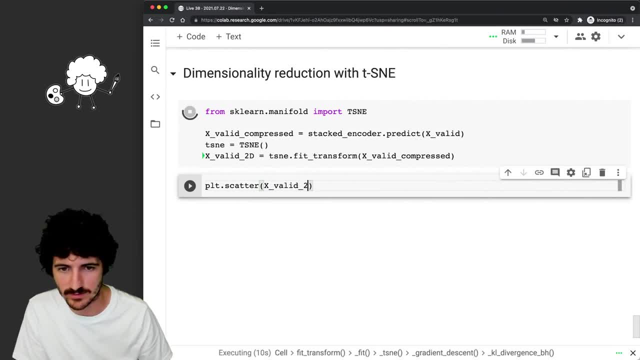 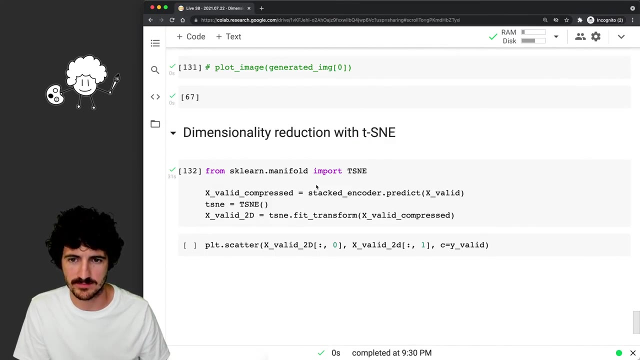 Plot make a scatterplot with the X valet to the everything and the zero X valet to the everything. on the one, C Y valet. Do we have Y valet? I don't know if I removed that for okay, So we need that for some reason. 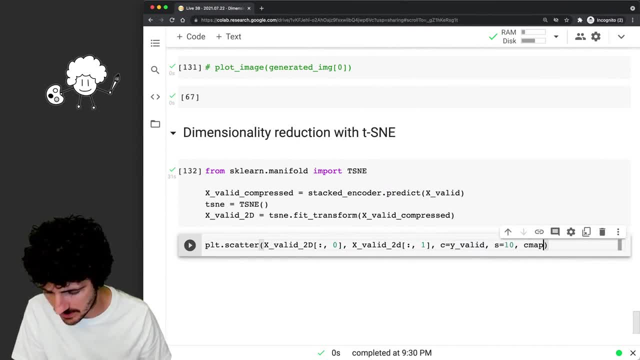 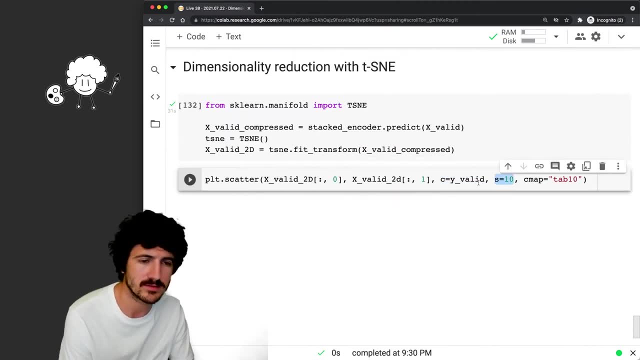 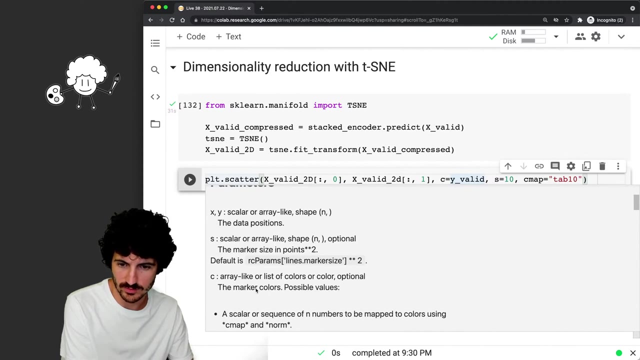 And we just need here, as 10 C map, top 10.. Yeah, And these are the categories, because we know the categories and we know that there are 10 different class. So scala shape rave list of colors or color options. color uh. scala array like shape option. the marker size in points. 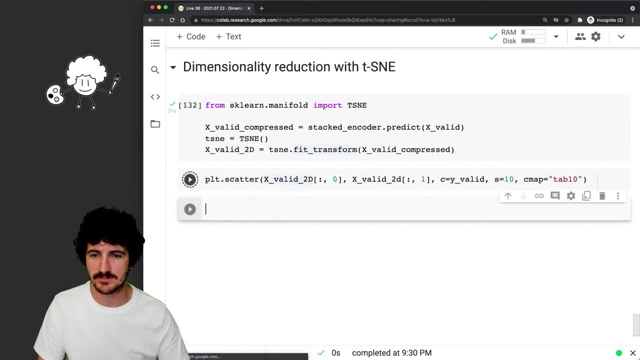 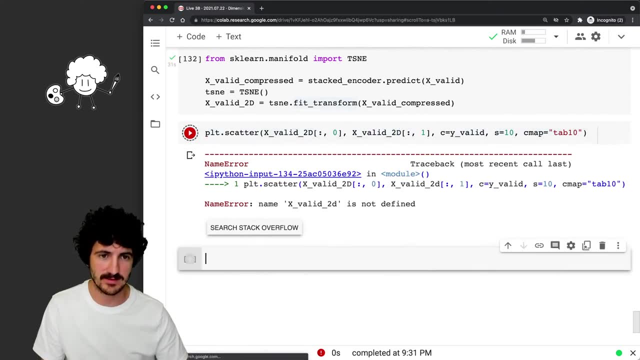 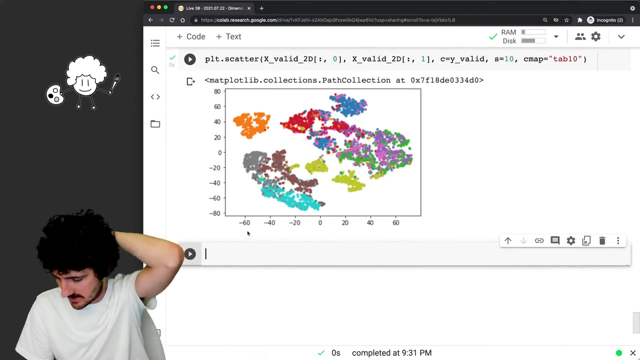 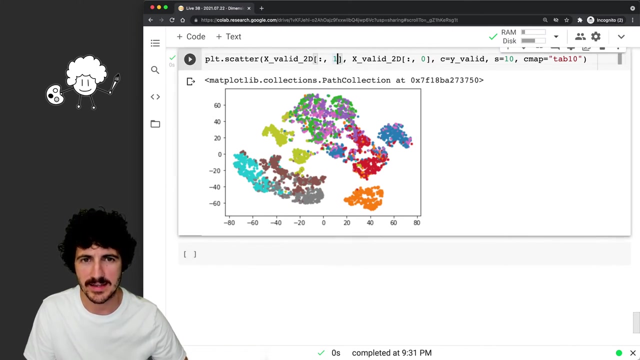 All right, Cool, Let's try this. X valid is not defined. All right, Cool, All right. So these actually matches This in some ways, kind of changing the axis. but I have on the um on the book So I think maybe if I changed, yeah, it's changing something on the axis. 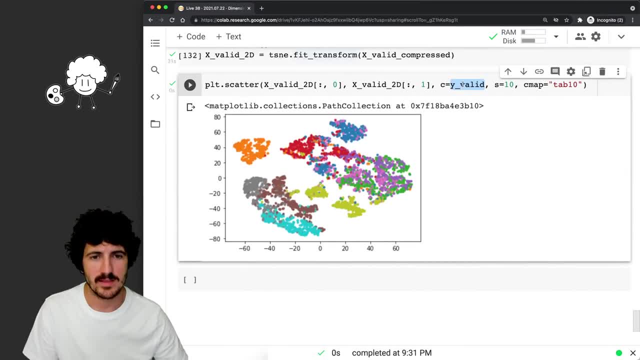 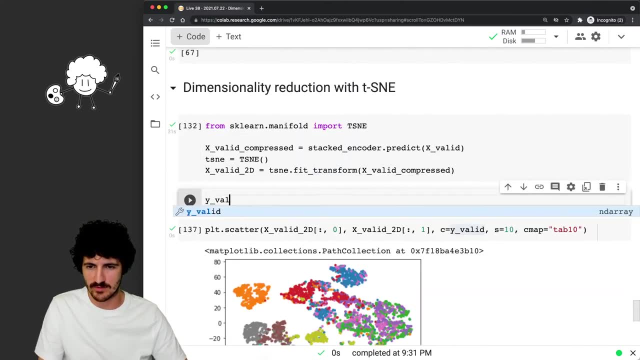 I don't know why, but it matches what I have on the book. Yeah, So if we didn't, if we didn't really have the call, so the valid, so if we print here, just so you see why valid and I take like maybe. 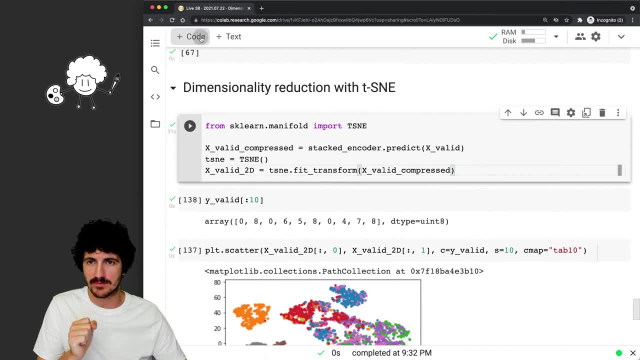 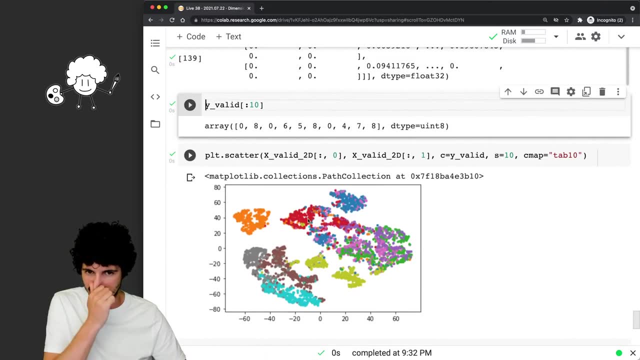 10, right, These are the classes of the data, right? So we have here X valid, And if I take 10, you actually have the images, right? These are the images that we're supposedly plotting there, And then here we have the colors. 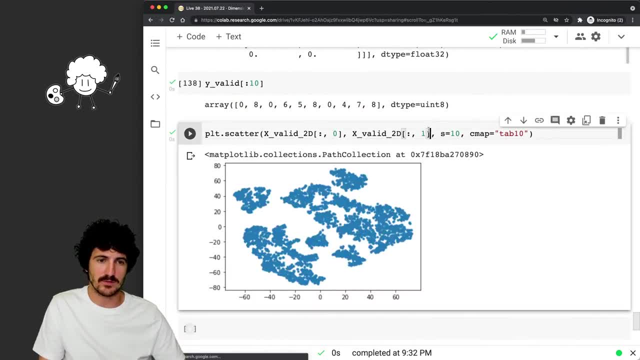 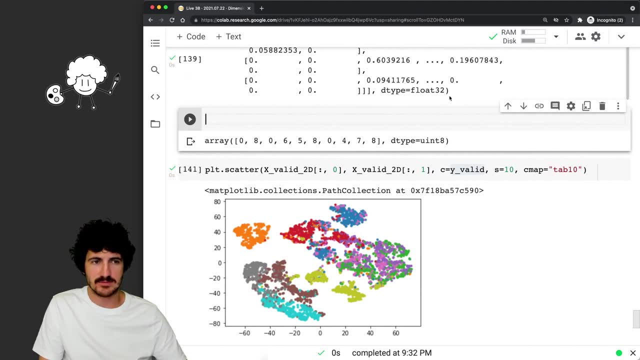 If I were not to provide that, we'll just get a set of of um Blood right, And you have to think that those have similarities among them. So this is neat right. This is the basis of what we were looking at. 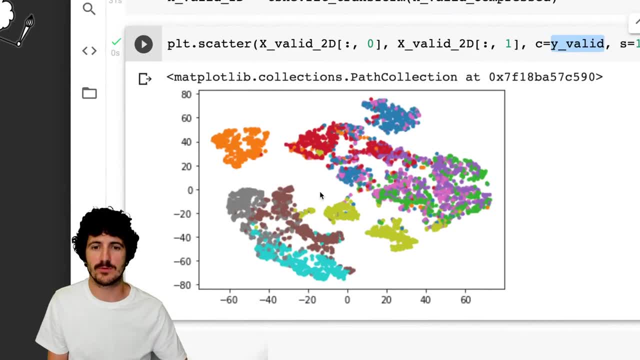 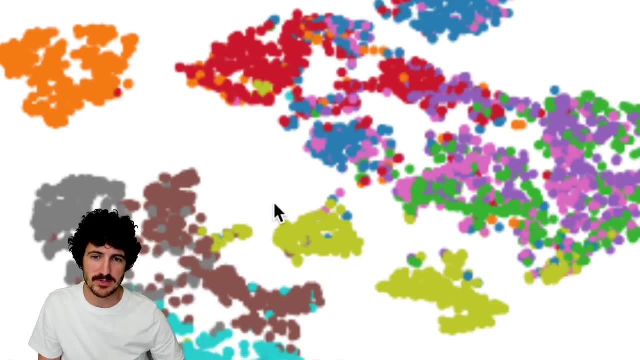 I want to continue, Continue farther with this. So continue, um, looking at this a bit more and developing these farther, because right now we just see, like plots here. We don't even see images or anything, and it would be good to lots of images here or like even have an interactive board where we display the samples. 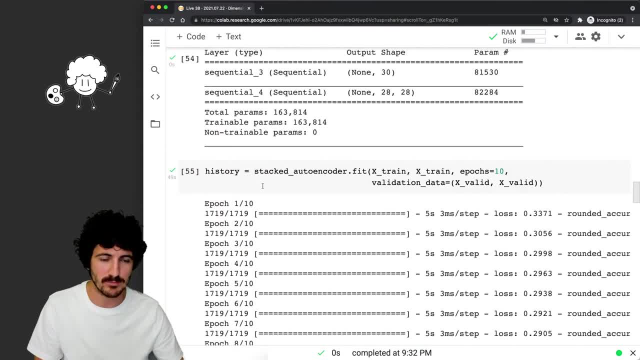 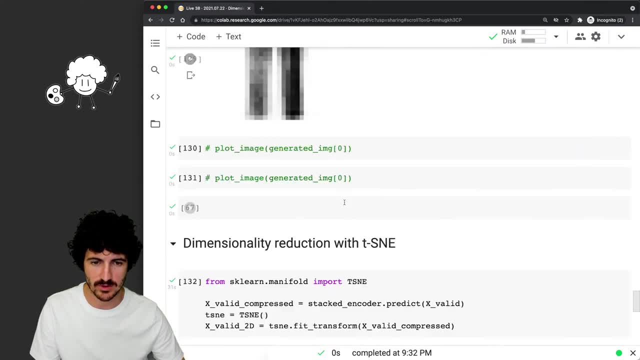 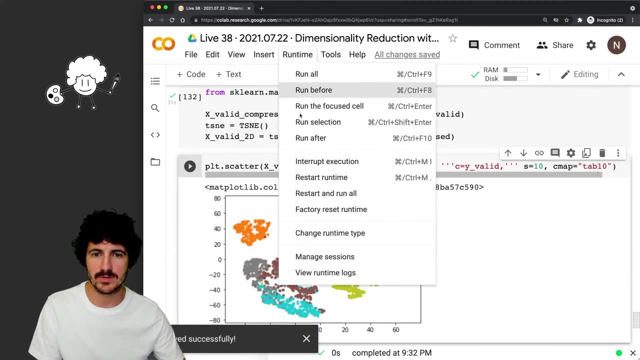 And what else can we do? Can I try once more? We're going to train- or this is super fast, So let's do a hundred epochs- and that we're not going to have X value this time. So we're just Going to remove this part and that we're going to reset and run all. 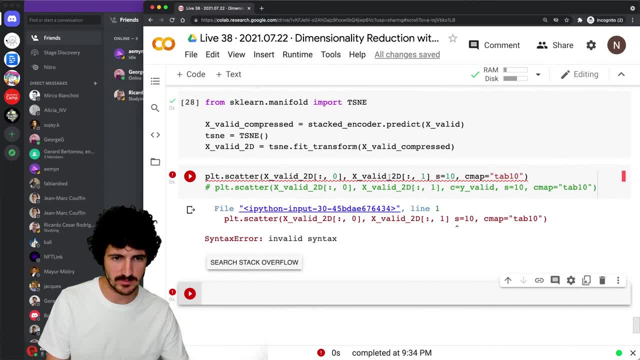 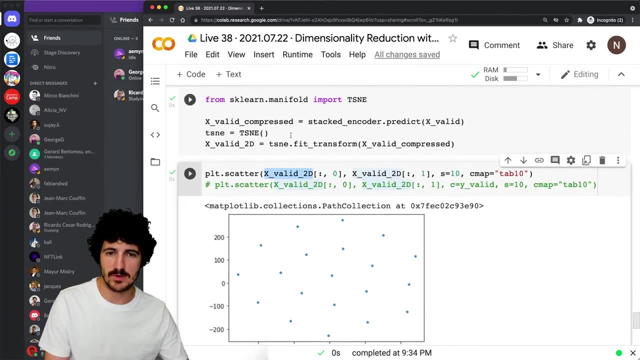 We're going to be looking at more dimension ID reduction algorithms. All right, So this goes here. Okay, What does this mean? X valid? I don't really want X valid here. We want the actual thing. So let's actually do here. 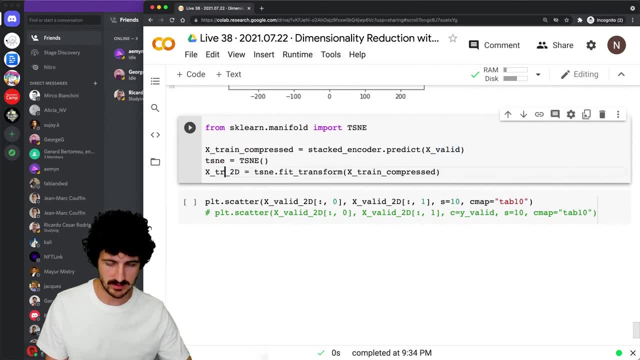 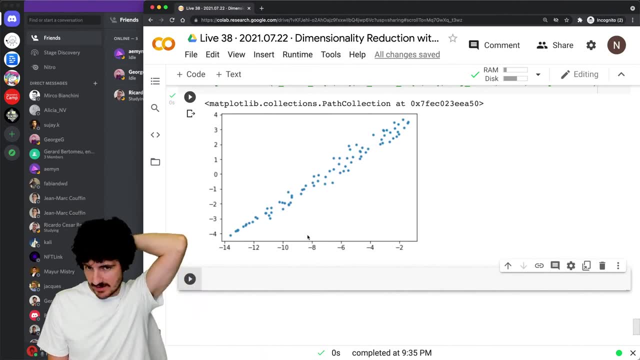 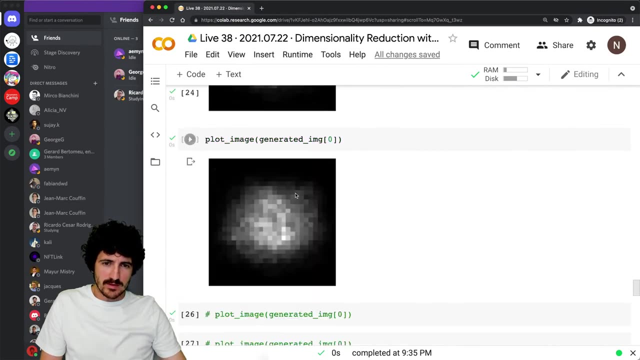 X train, compressed X train to the X train, And that should be it All right. So It seems like it's still is fitting some in some way. these these drawings, by similarity. I don't know that they're that different for them to learn any other things. they're spread on on space. 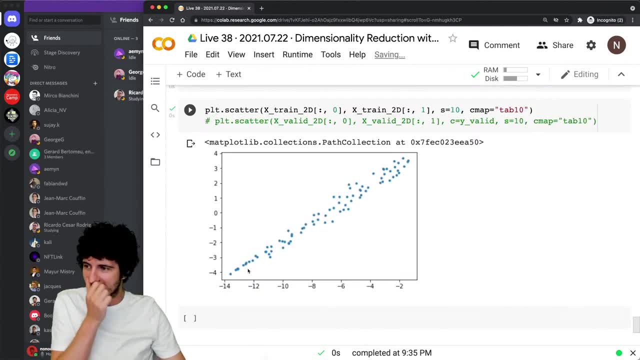 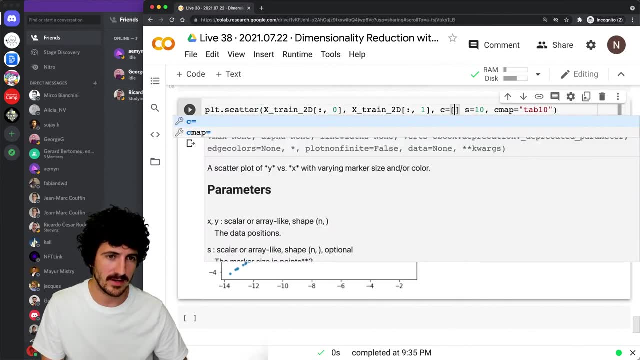 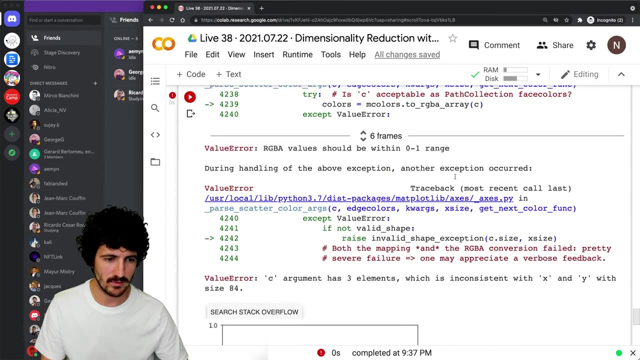 Let's say and- and I really want to now see the plots in this individual sketches and see which ones they are- Can I provide here a like an array or something, when like zero one, to remember now what the shape Of this was: 84 with X and Y. it's size, 84.. 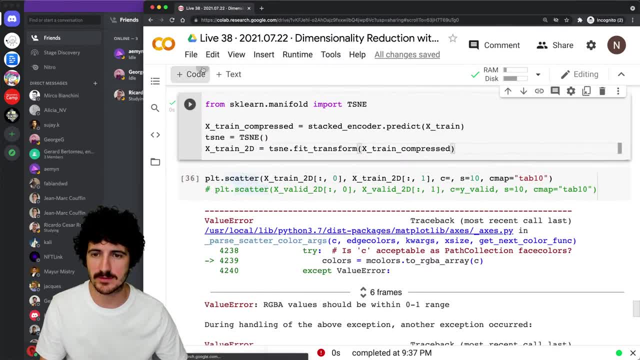 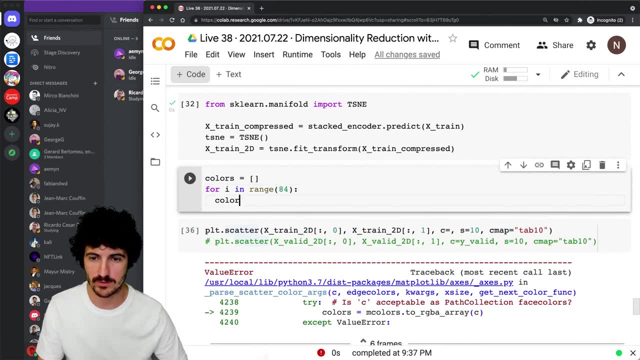 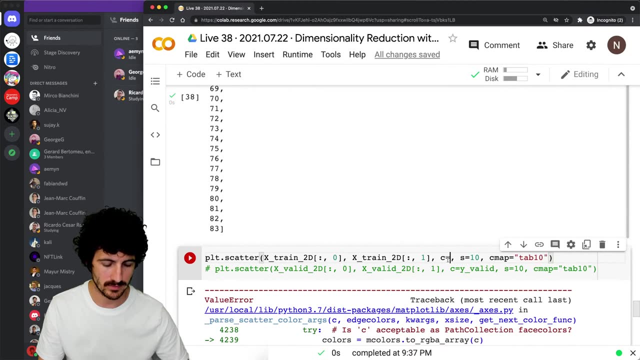 All right, So range: let's actually make a list manually. So colors equal that. And for E in range 84 colors, append I colors. Let's see All right, So we get 83 and then we can put that here. 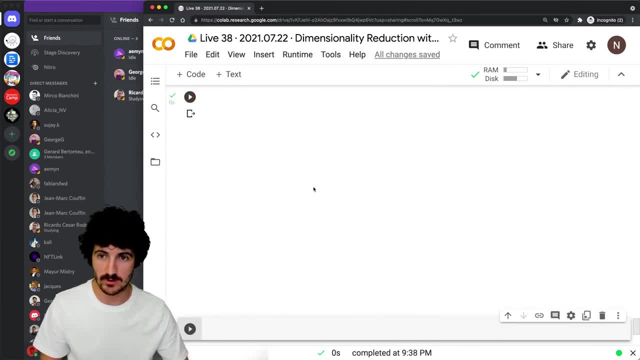 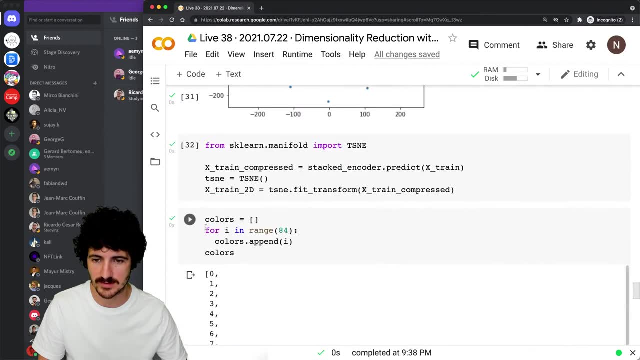 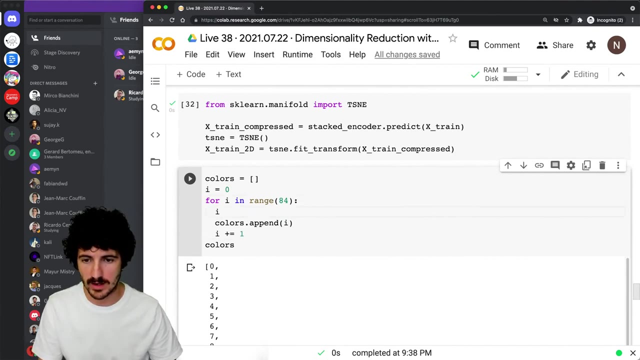 Colors. We get 84 colors and that plots. All right, That is useless, but we're going to do something, just at least to cluster them. So we're going to say equals zero and E plus one, And then when I, if I is greater than nine, I is going to be zero. 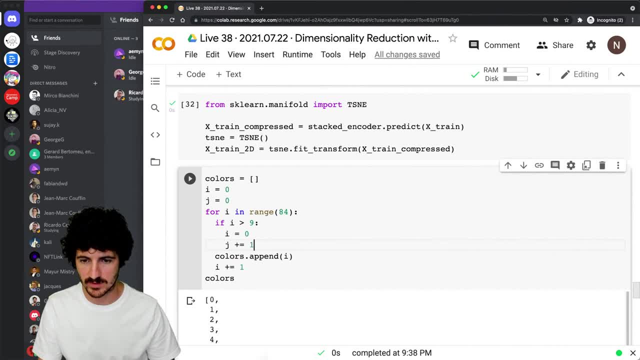 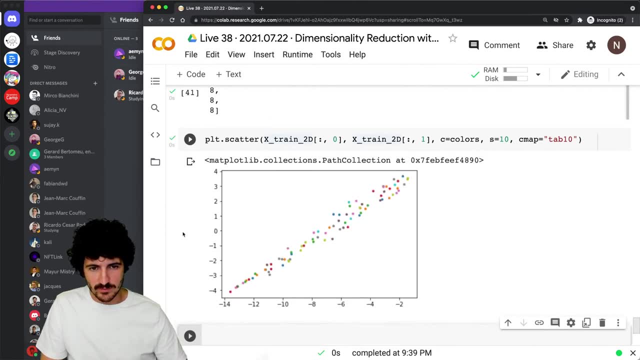 And J is going to go up, So J plus one. So we have less colors. So Let's see, So let's see how those colors play out. Great, We have too many colors still, So we might just need, let's say, we just have three clusters. 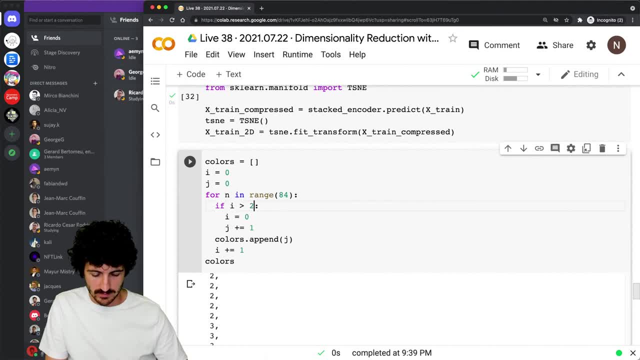 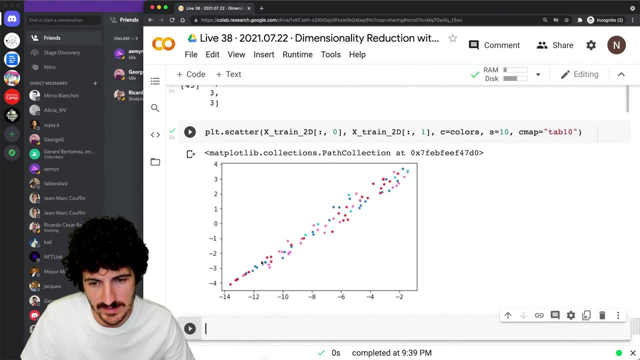 So 84 divided by three, that's 28.. So there's a 25, right, We have not three colors. So it means that this is telling us that drawings that are not initially together- right, That this is not the order they're like, being clustered in different ways. 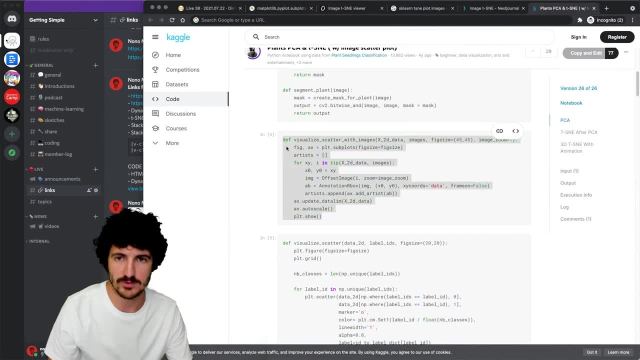 What do we Have here? We should like scatter with images. Let's try to just copy paste this one, which you shouldn't really copy and paste code, but because we're finishing up, let's see if we get that stretch goal. 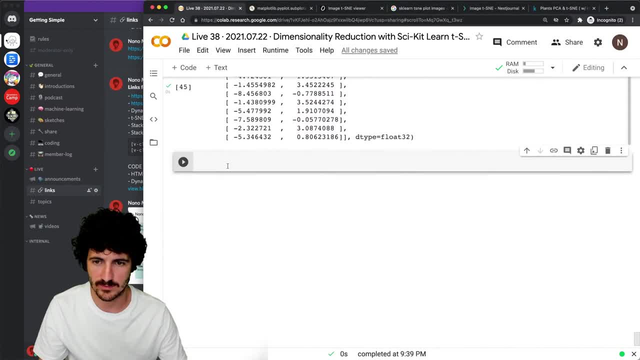 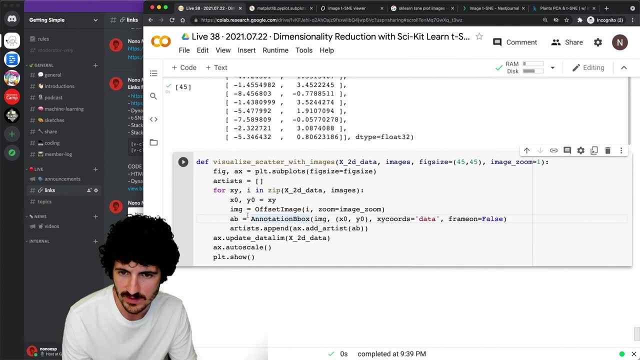 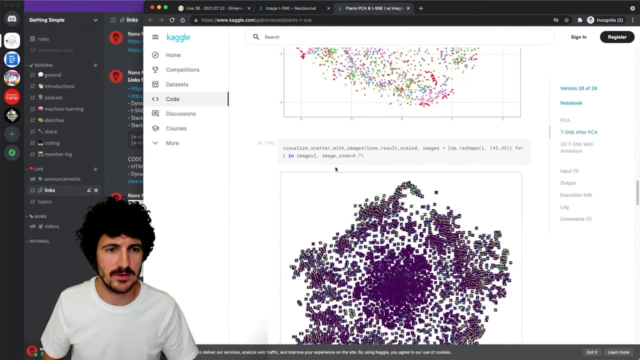 All right, So we got this here and we have this. So plot annotation: bounding box um offset image. Okay, Let's see, So we can define this. So visualize: scatter with images. Let's see. Oh, that is awesome. 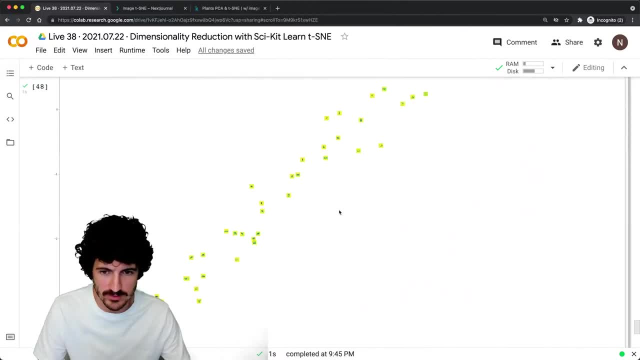 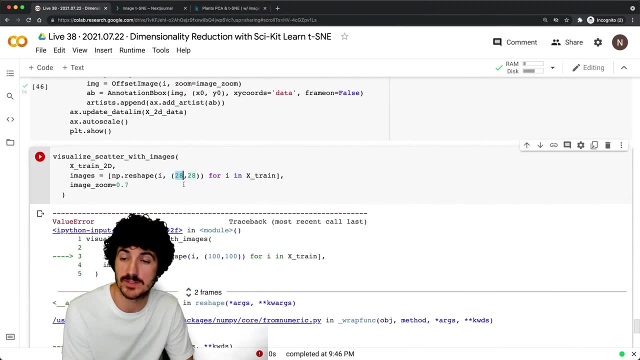 All right, So copy pasting. we got a pretty good resolution image, I think, and I might be able to maybe pump this up. Can I reshape array into shape? Oh, reshape not rescale. Okay, Image soon, Let's do maybe four, because this is, these are too small. 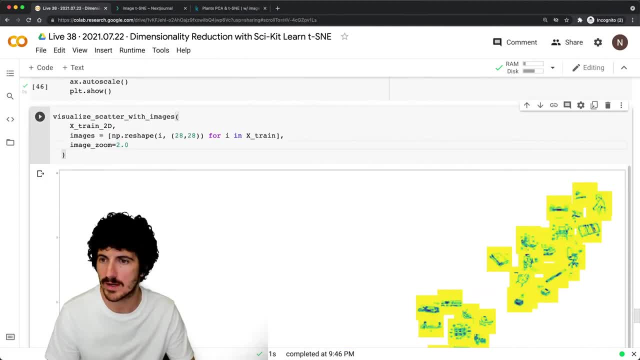 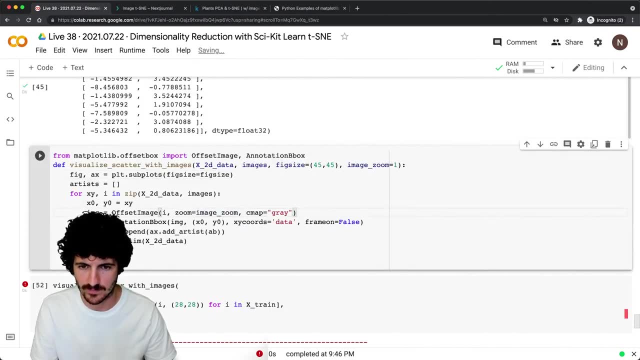 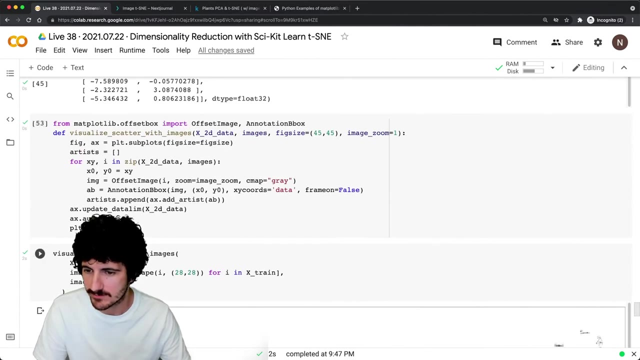 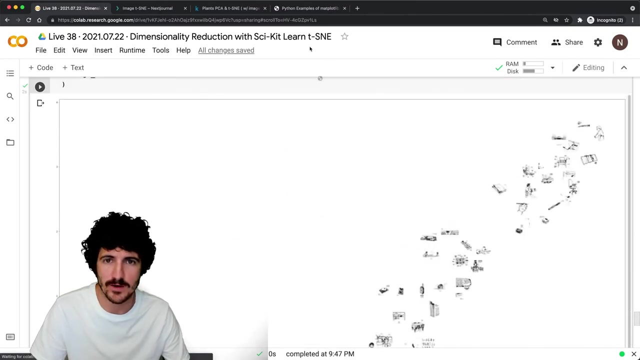 Great, This is pretty awesome. Maybe let's just do two. I don't know why it is coloring with that. Ooh, this is looking super good. All right, We got it. So, um, I don't. I don't think we're going to. you know we're going to get too far with this, but long story short, I think we got it. 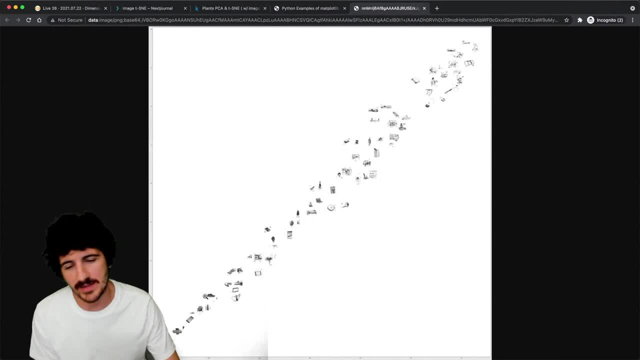 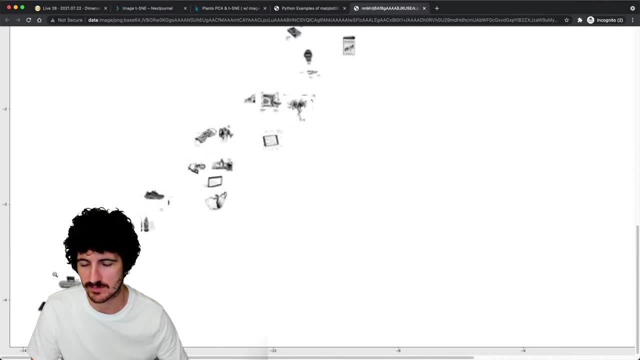 We got what we wanted. So it seems in some way it doesn't seem like it learned too many different features. It just seems like the darkest ones are, or like the more infield ones are on the bottom left. These ones are the ones that are from some like people. 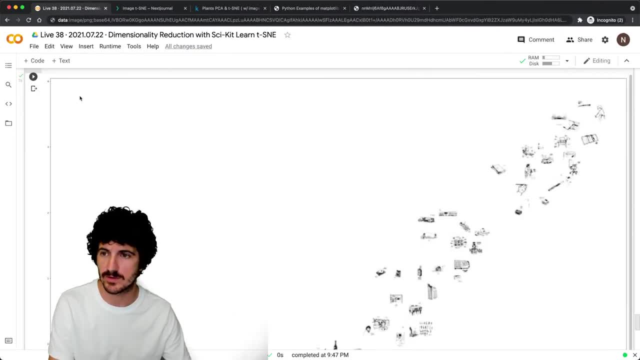 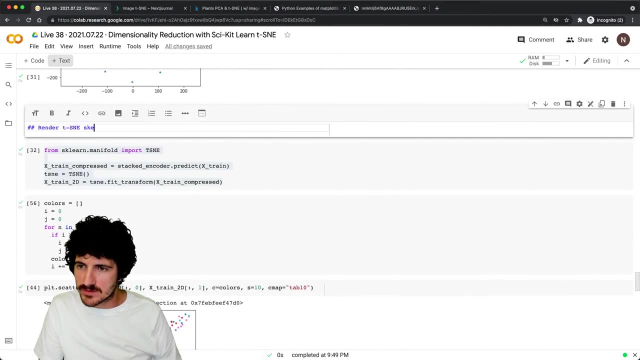 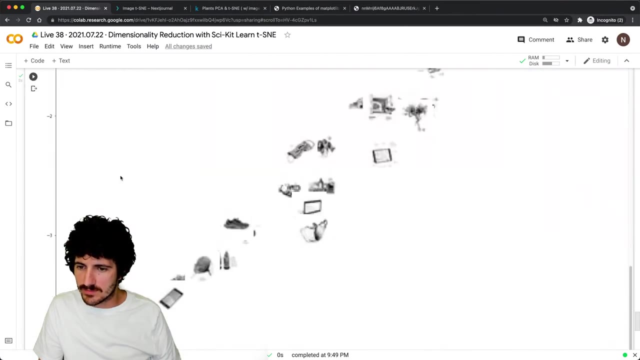 I'm here. I think it would be a bit crazy if we do that with a segment of of the other ones. So let's try to just copy these Disney sketches. Um, we're now going to copy these and paste them. I don't know if I can paste them here. 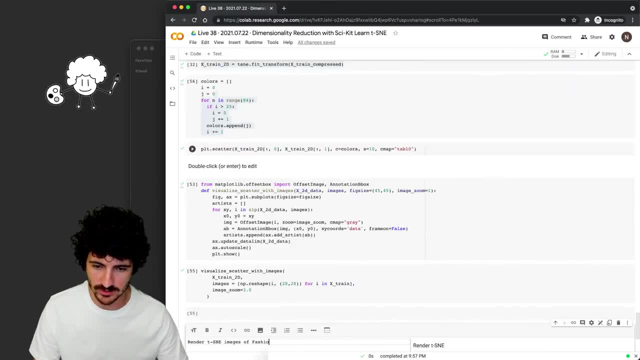 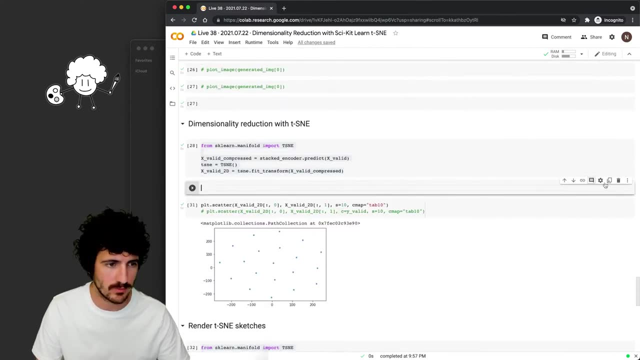 Render Disney images of fashion MNIST. Okay, All right. So how are we going to do this? We can remove this. We don't really need to Bring this anymore. We do have this with it here this year and we do want the colors. 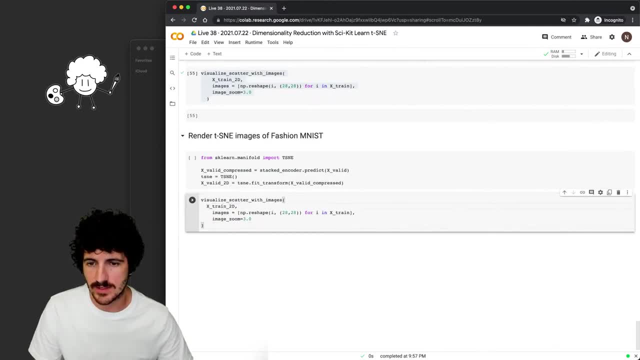 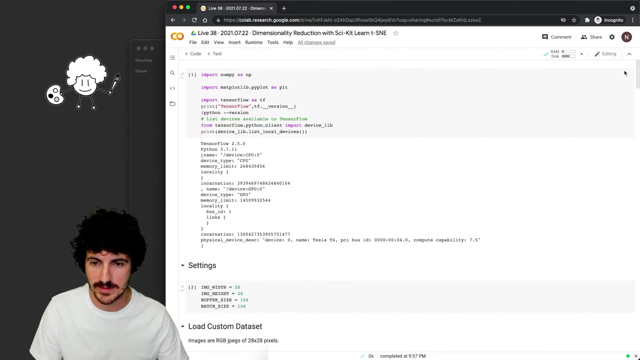 We don't really need this anymore. and X train to D and X train. Maybe we're going to have more images, X valid. Maybe let's just pick 500 images for now. We need to train the model and that's going to take a bit of time. 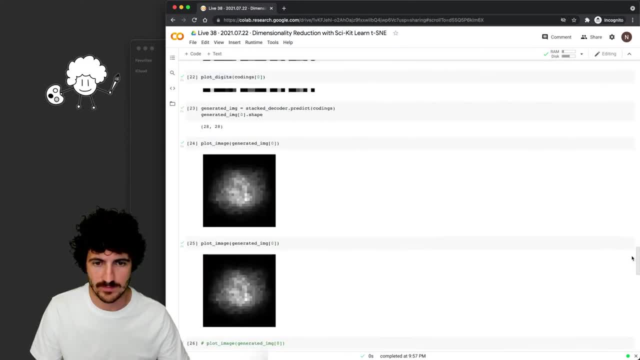 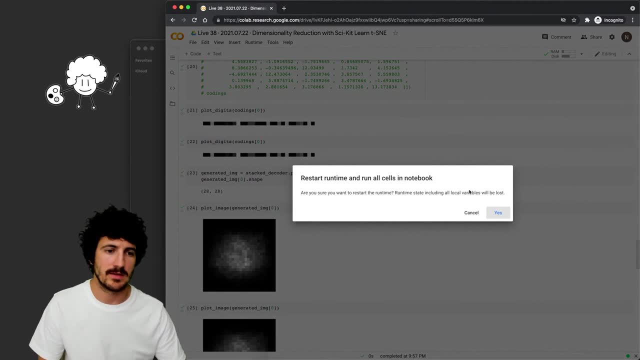 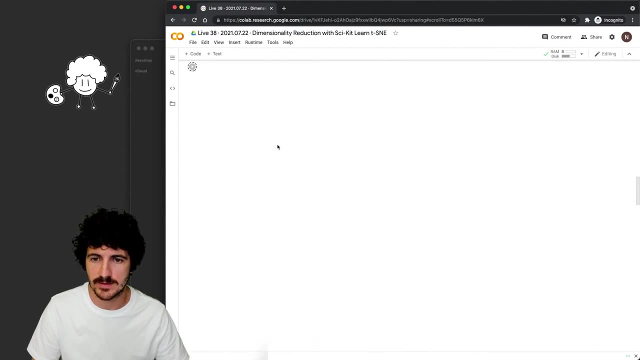 So let's put this back. Um, let's start and run off. There'll be things that are not going to work, but, uh, we'll get there, And these probably the thing that's going to take the longest. So we're going to start again. 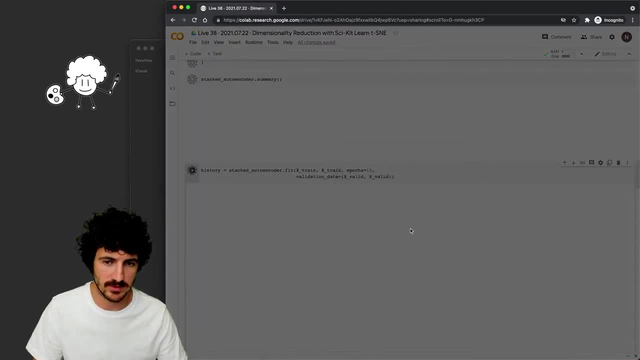 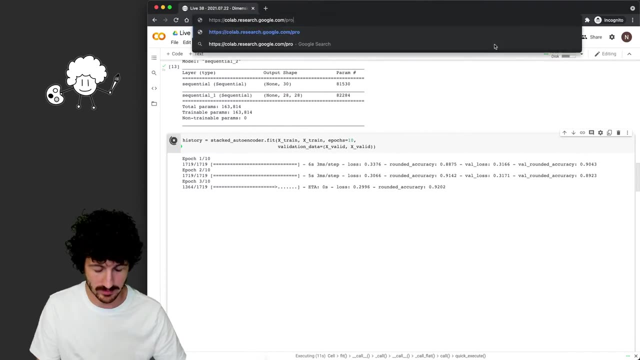 All right, So we're running again. I think we're still using a GPU and you should get a call-up pro if you're going to, if you're going to be training models for long call-up, it's in maximum, so definitely worth it. 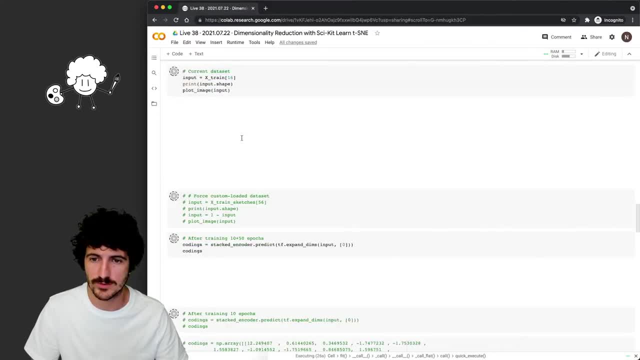 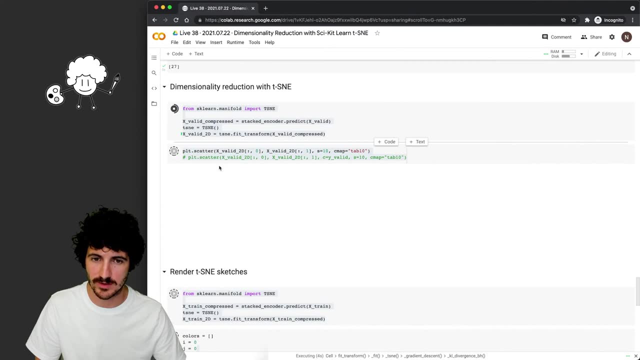 All right, So we're training five or six out of 10.. We're almost there, So we should be now done with training. We are great And we probably going to see some error below, but let's see, probably not. 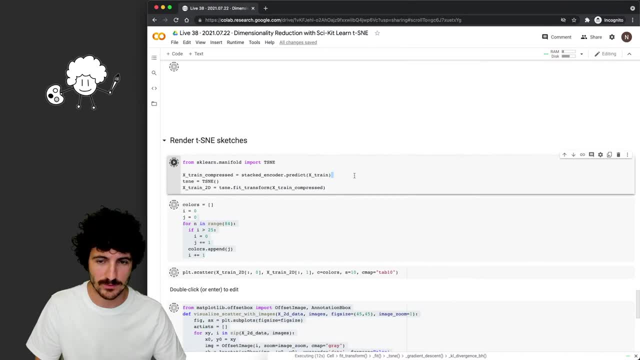 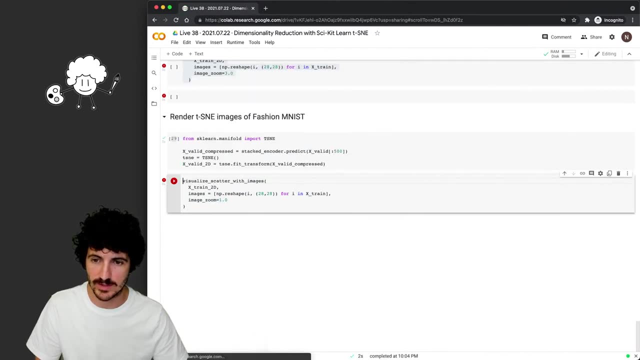 I don't think this is going to get completed. This is too much to be plotted All right. So I'm going to interrupt that one, because where I want to really get is here. So we do that And then Visualize. 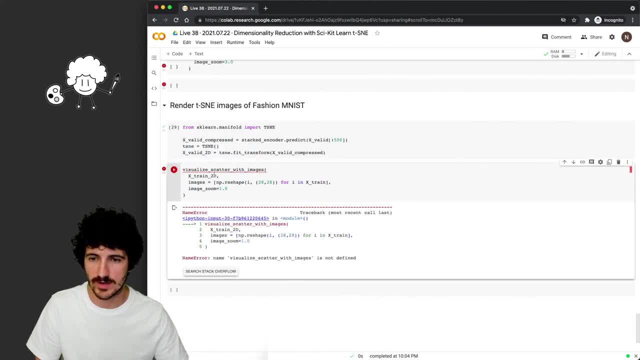 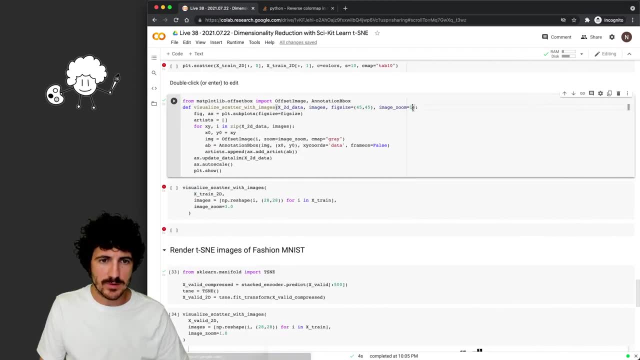 Okay, And we run this helper and then we run the cell once again: X train to the X valley, to the all right, Whatever. So we do here, see my gray, we'll run that again And we're going to do that here. 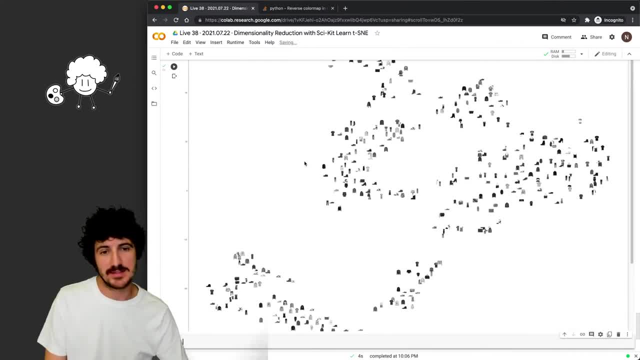 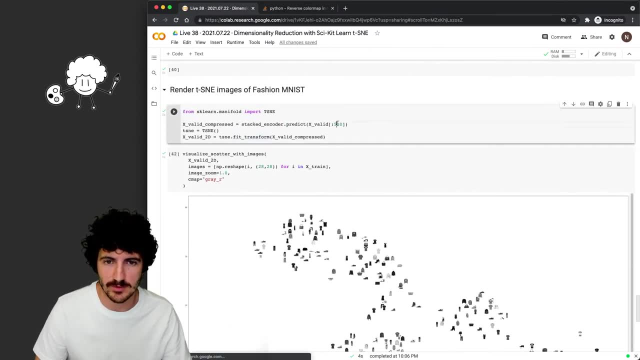 See my gray are. this is indeed a pretty, pretty cool Okay. What this tells me is that you know we haven't trained for long enough. Probably I'm going to get more samples, So I'm going to take 2000.. 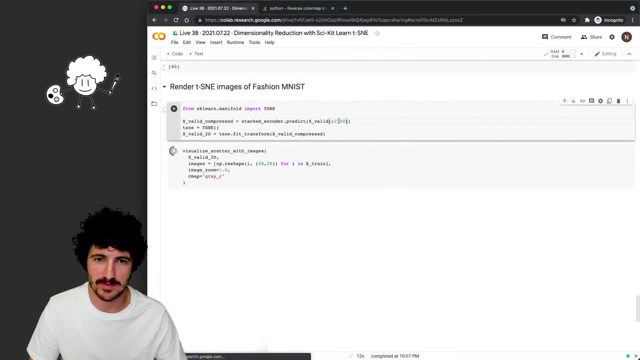 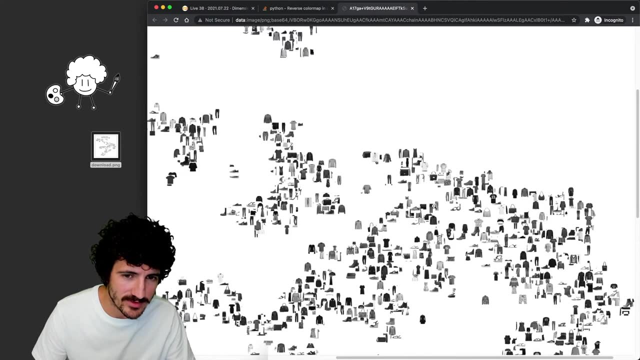 500.. So let's see, maybe it's a bit too much. Okay, That works. That's a cool image, right? I don't think these ones are similar. Not sure if we're doing anything wrong here. Let me see if there's anything. 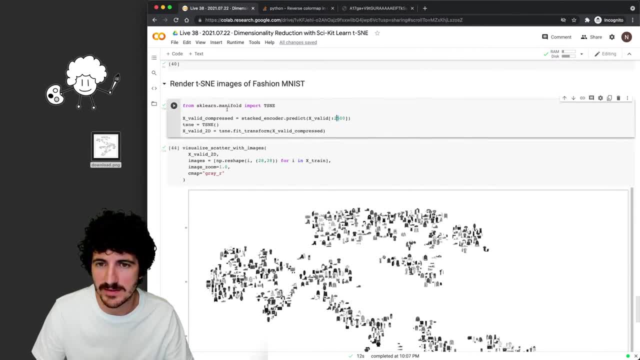 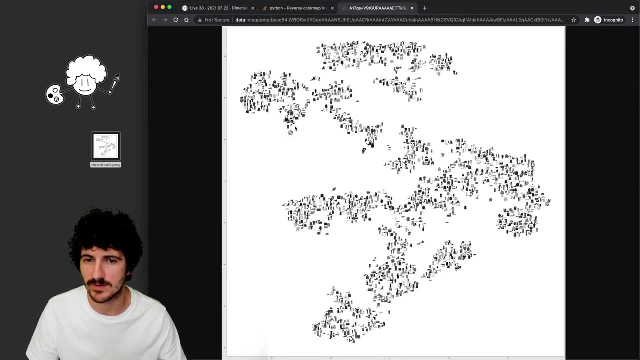 So X valid, X valid compressed X valid, It X train, All right, X valid images. Okay, So we're X valid to 500, right, Let's see? Yeah, this is like looks wrong, Definitely. 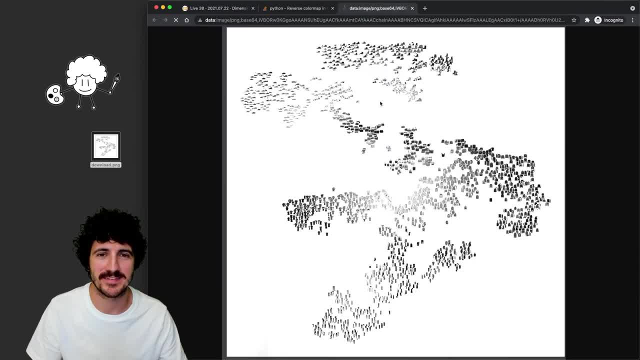 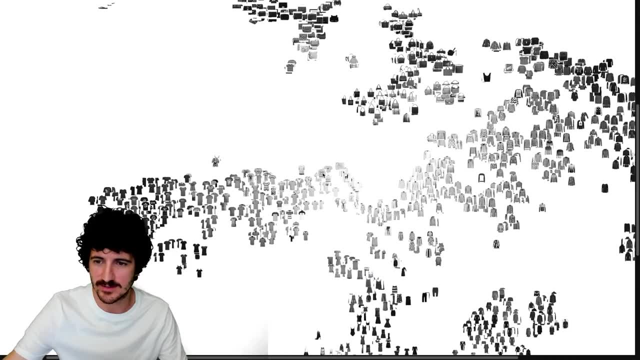 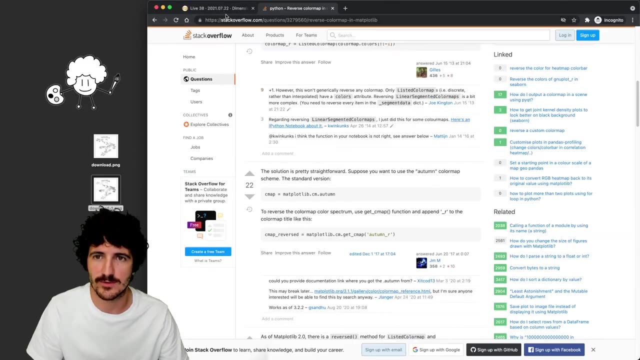 Okay, That's so much better, That's awesome, Okay, So this is, this is really cool, So this is awesome that just with 10, um 10 epochs, these looks so good. So let's parameterize these then, because these maybe we can do even better. 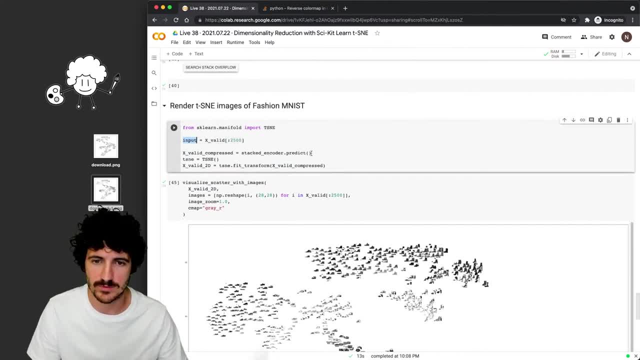 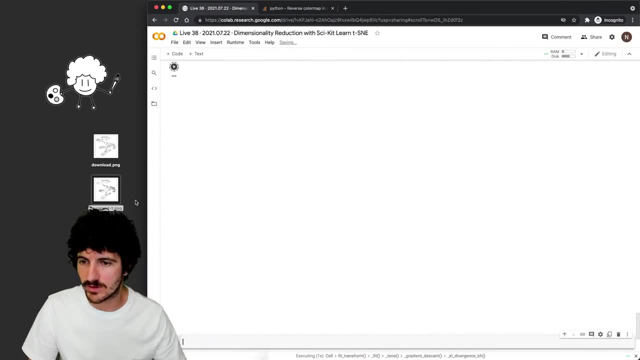 So we'll do input. It's going to be this and we'll just predict on the input and maybe it's inputs. All right, I'm going to generate this just to make sure that we're getting the same. So zero, zero, zero one. 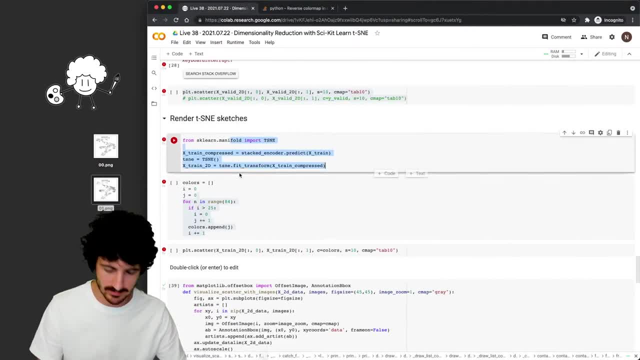 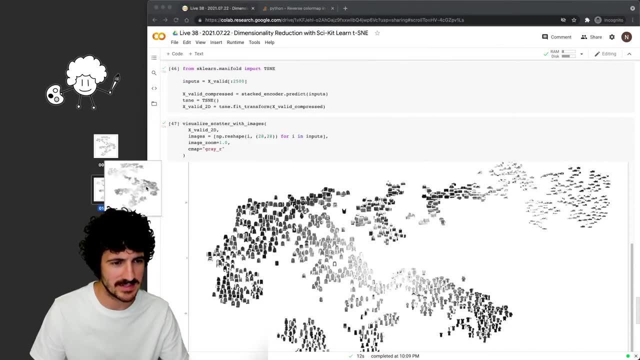 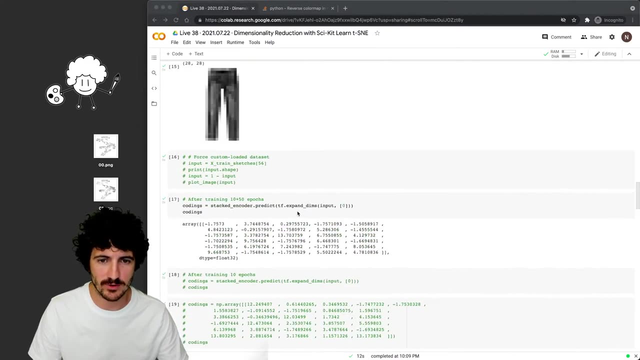 And, uh, what we're going to do right now is I'm going to close this thing. So common. this is being plotted, which is pretty cool. This has not changed. I'm sure why he changed for some weird reason- And we're just going to train for longer just to see how that image actually changes, how the sorting changes. 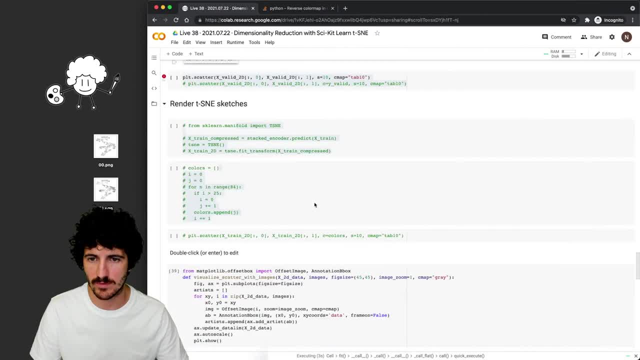 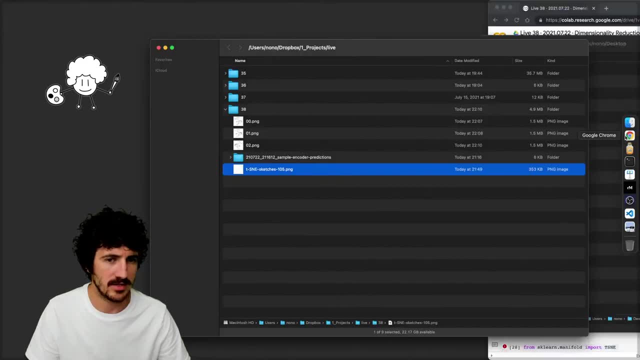 So we're going to train here for 20 epochs And when we have the model trained, these will be trained for 30 epochs total, And then we'll be able to get this thing. Let's check that the images on the other data set at all.